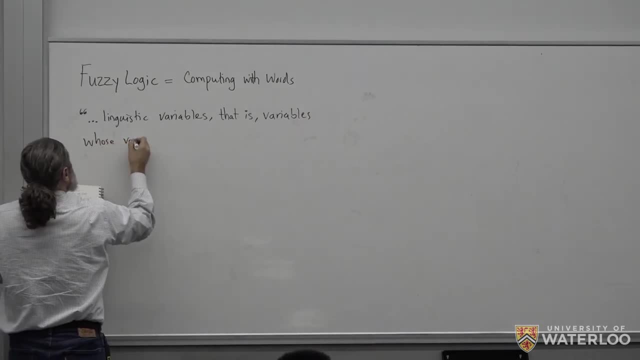 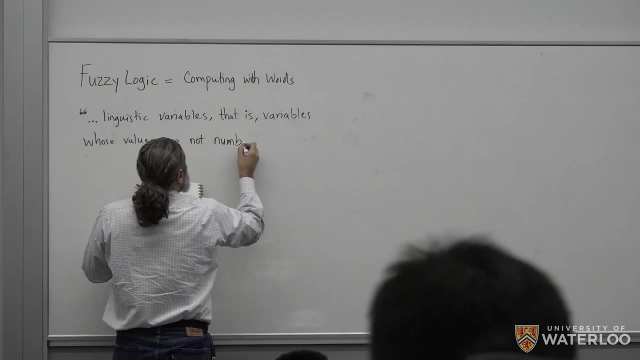 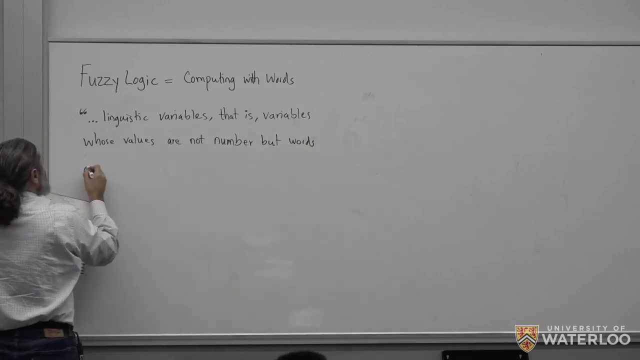 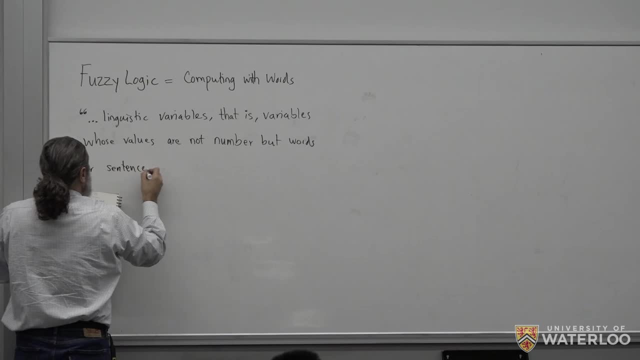 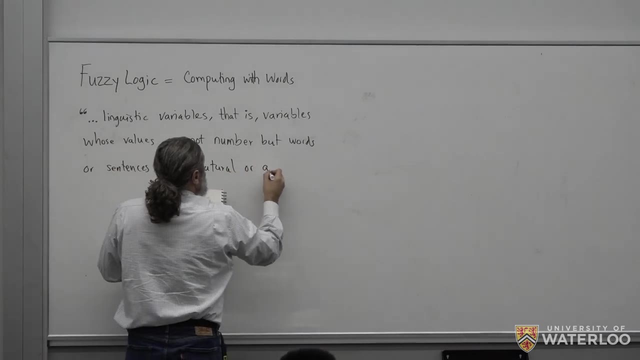 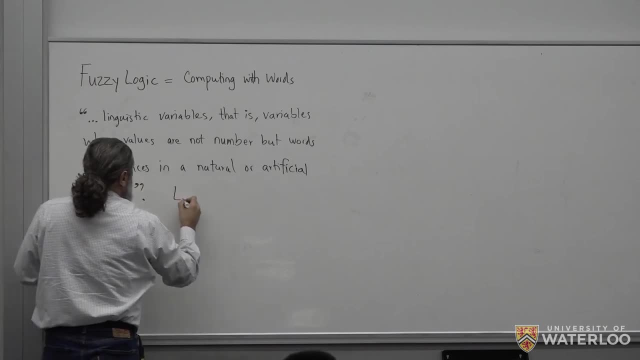 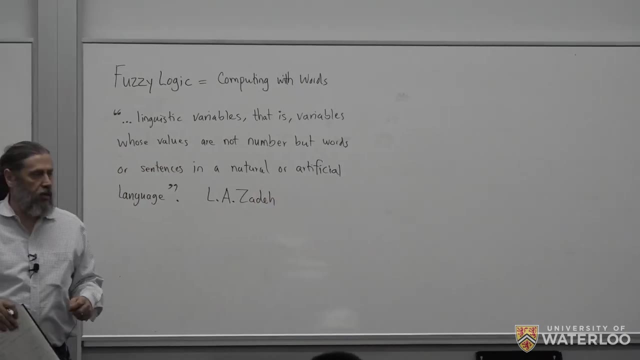 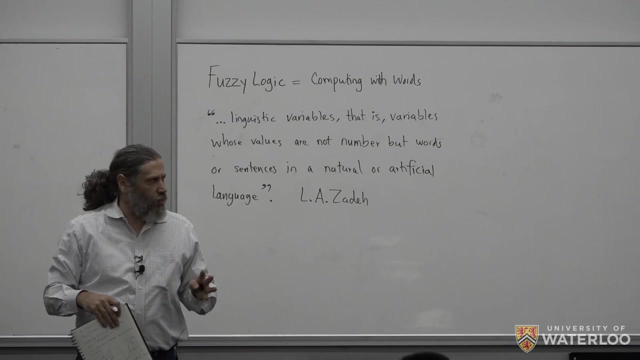 Okay, Okay, Okay, Okay, Okay, Okay, Okay, Thank you. So that's in one of the first three papers that the father of fuzzy logic came by and established the concept of linguistic variables, which was in mid-70s of past century, was something. 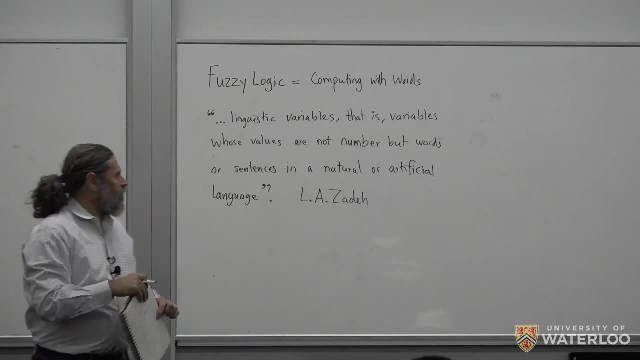 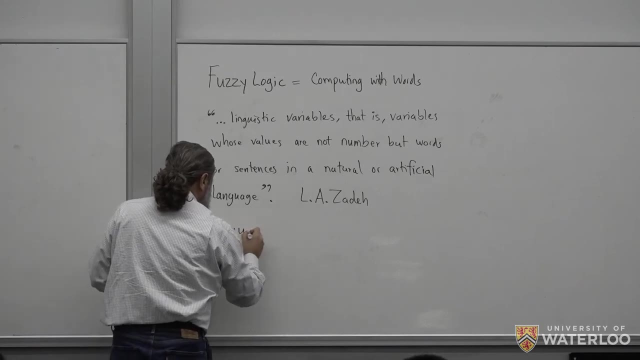 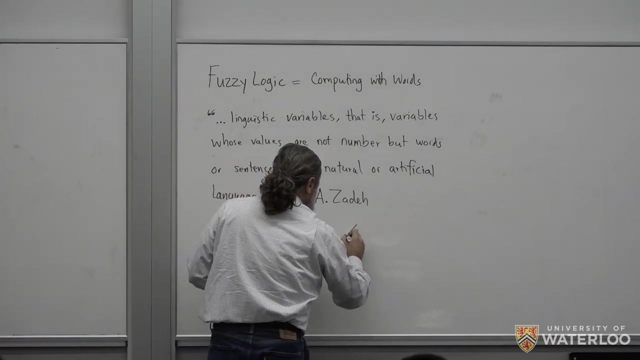 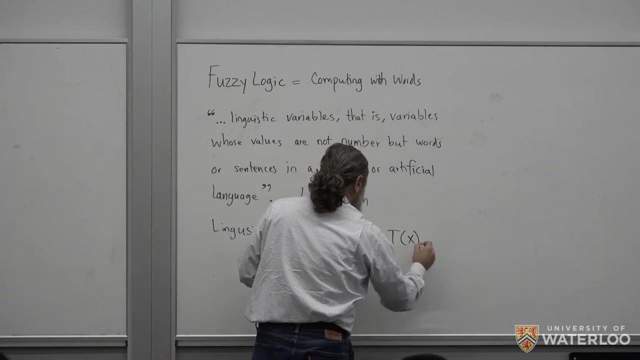 outrageous. So what is linguistic variable? So I want to work with numbers. So a linguist can't get rid of a language. So I want to work with a language, So a linguist can't get rid of a language. variable is a collection of five things: a variable name, a set of terms- T of X, a. 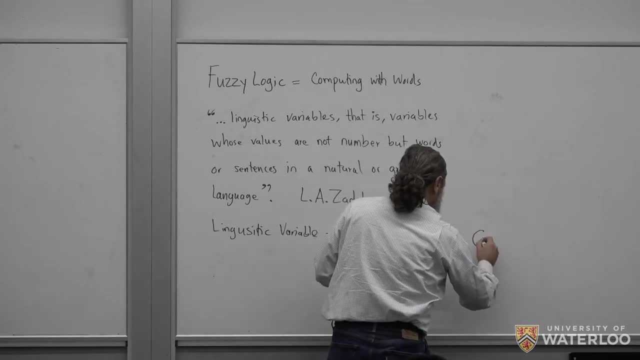 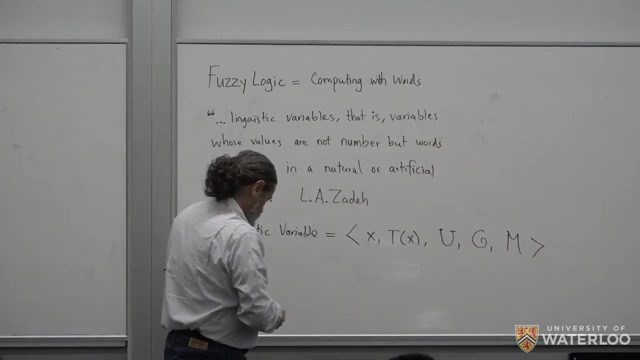 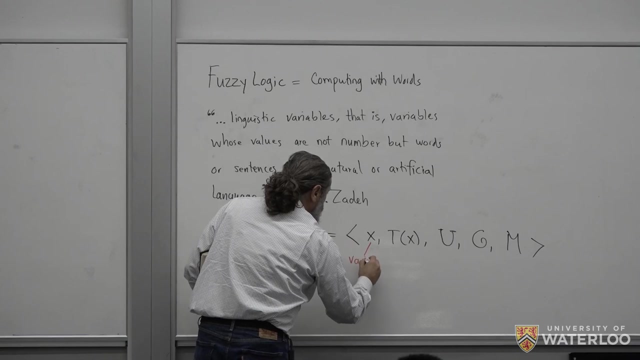 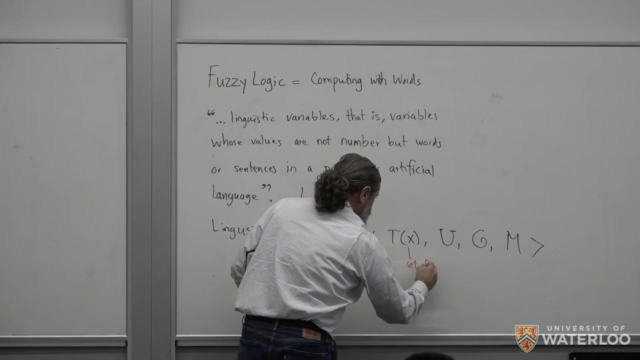 universe of discourse, a set of syntax rules and a set of semantic rules. So that's your variable name, This is a set of set of terms, This is your universe of discourse And this is your set of terms. And this is your set of terms. And if I 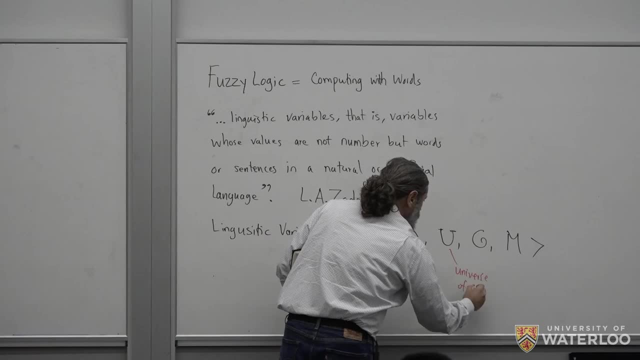 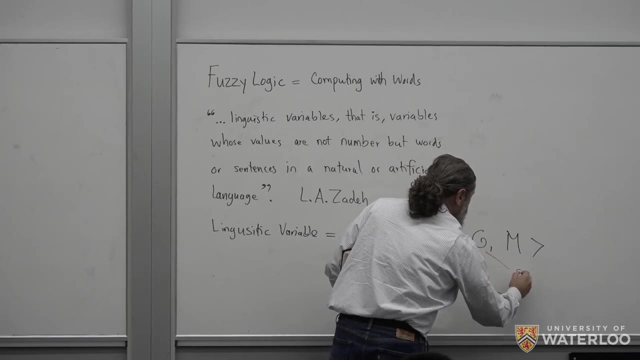 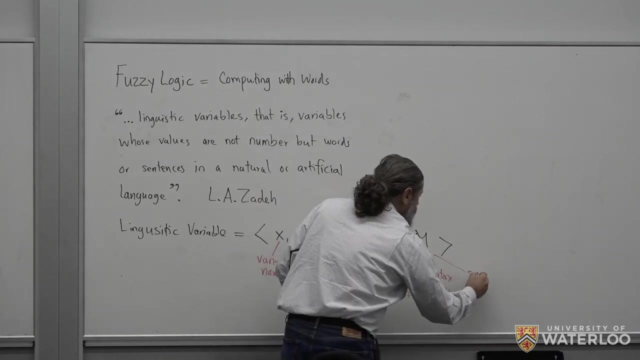 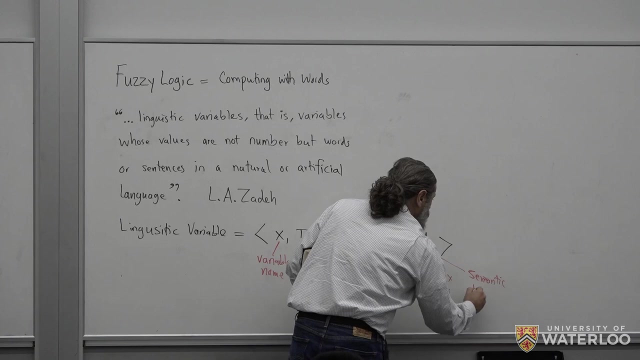 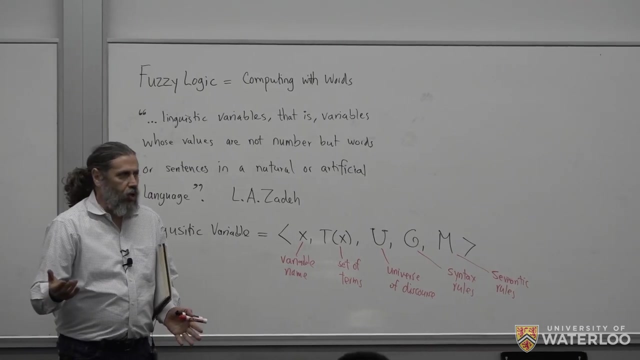 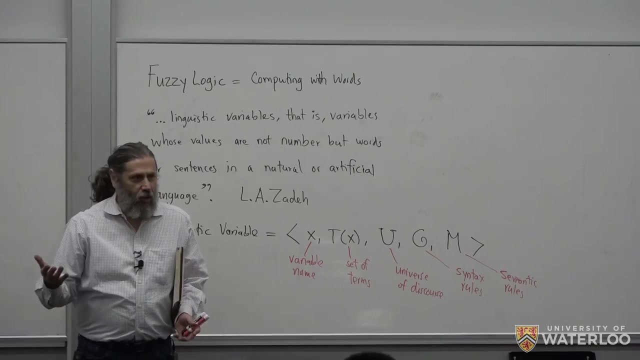 course, And this is your syntax rules And these are your semantic rules, Semantic rules. So usually, when we are working with variables, I just have a variable name and it has a value. That's it. But apparently linguistic variables are more complicated, So that's the way that. 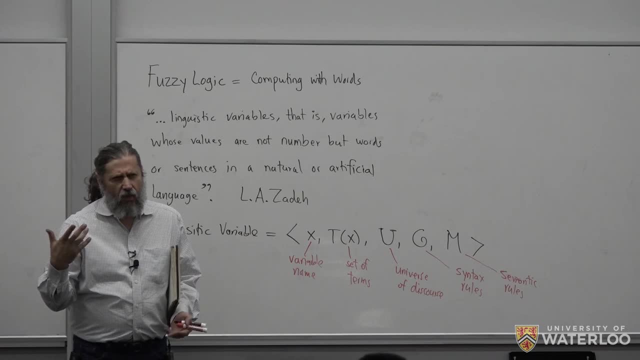 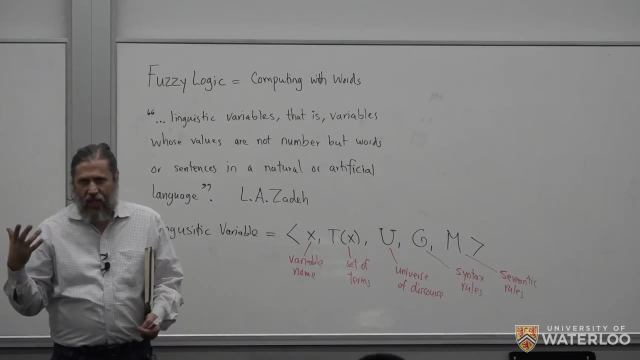 humans. So the main motivation for fuzzy logic was and is: we convey a lot of information through the language, And the human language is highly sophisticated And it's compressed, It's granular, It's ambiguous. If I tell you a little bit to the left, what does that mean? What is a little bit So somebody? 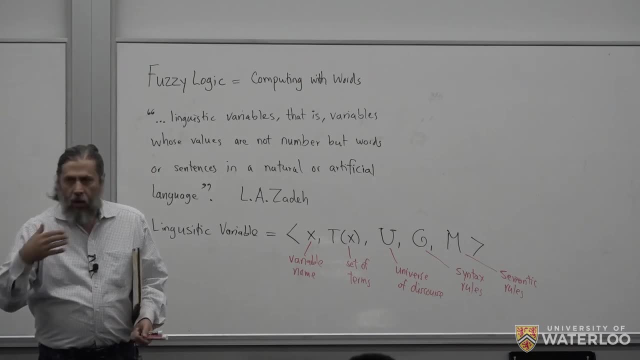 is not that old. What does that supposed to mean? We do that on a daily basis. We don't have a problem with that. Humans communicate with the vagueness of the language, But apparently if you want to put it into a computer, you have to come up with something that makes. 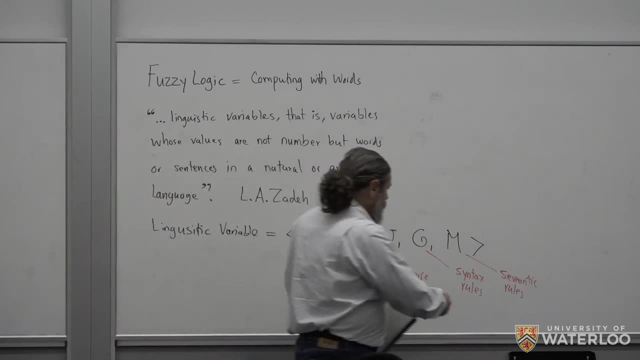 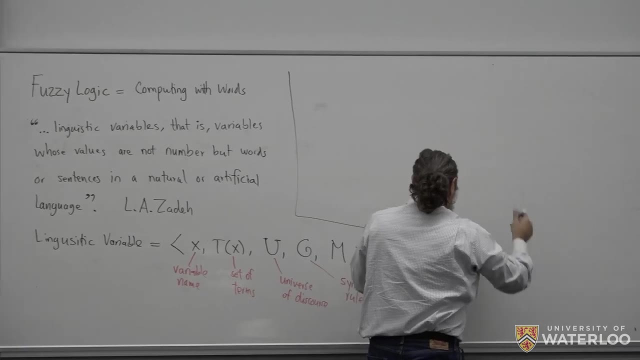 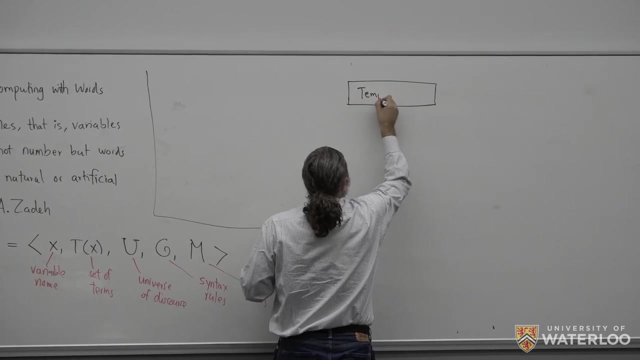 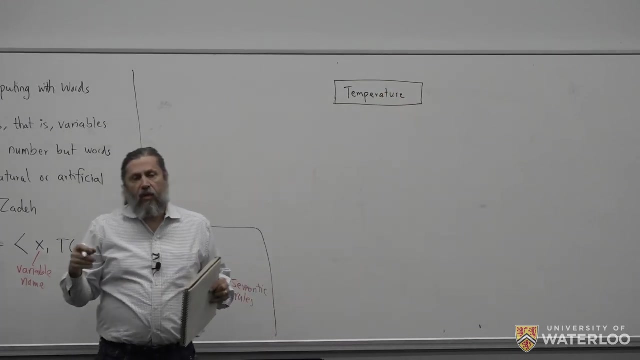 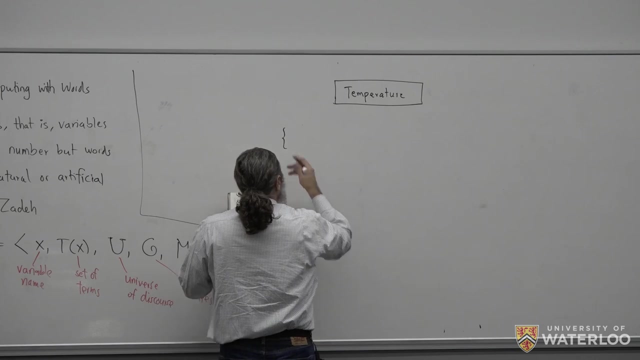 it more accessible to computers, So So Okay. So If we let's say we are talking about temperature, Temperature is something we understand, It's intuition, We can feel it, There's no problem with that, And temperature could be so when we describe temperature as intensity. 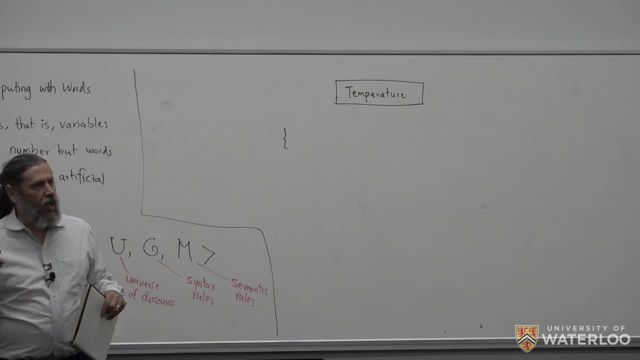 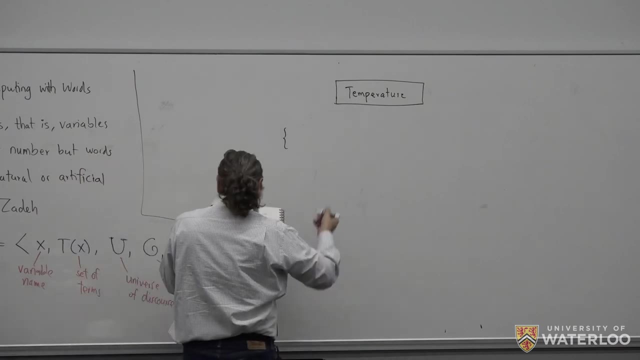 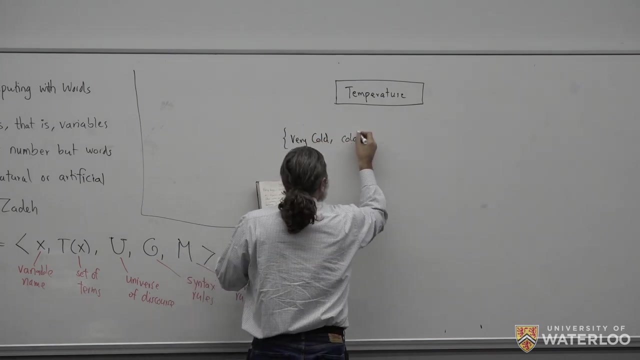 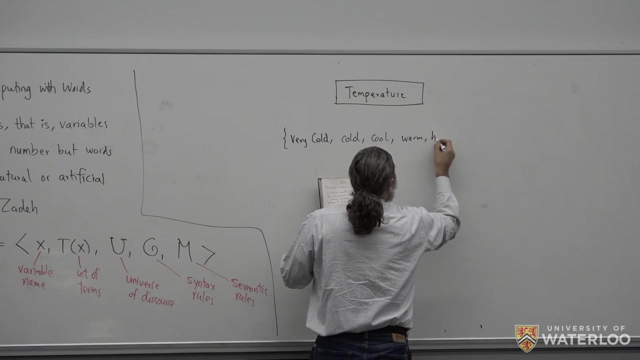 we use many different hedges, linguistic hedges. We say hot, warm, cool, very hot, extremely hot, and so on. Let's say I will go with very cold, cold, cool, warm and hot. So let's say these are the five terms that I'm using to describe temperature. 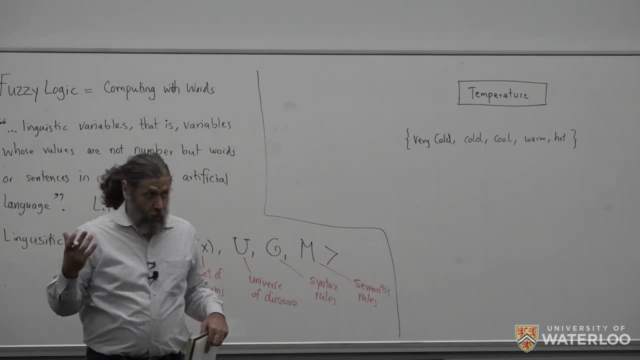 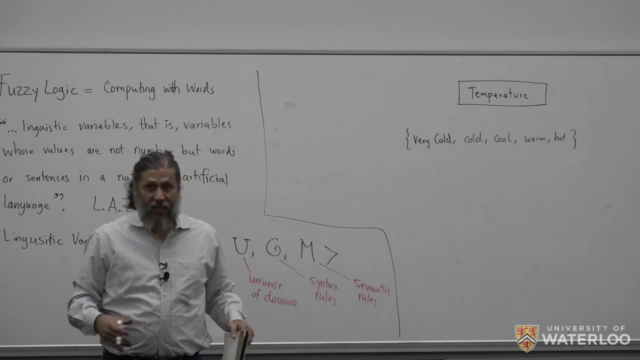 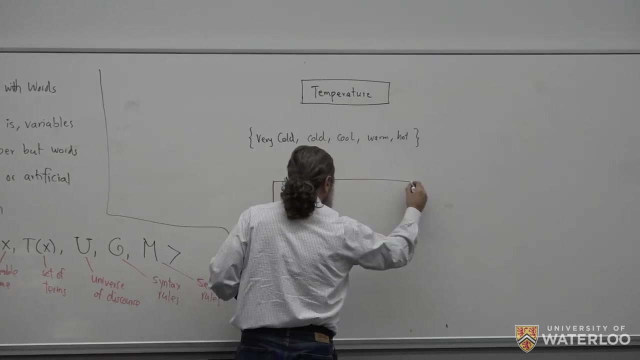 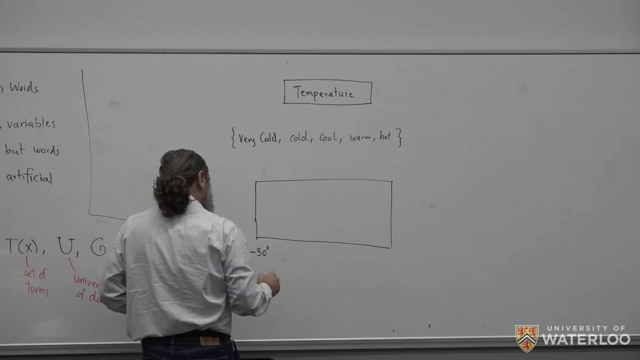 Of course, as humans, we don't do that. As humans, we are very flexible, We play with many adjectives, with many intensities, We combine them. So we are quite creative about the language. So and then? so let's say, we go say in Canada, we are used to what? 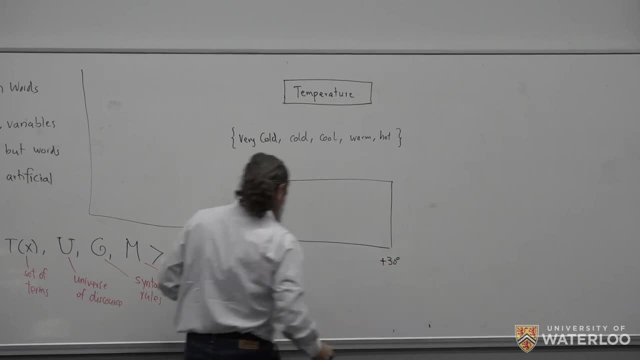 Minus 30 to plus 30.. It's actually more drastic than that, but let's stick with minus 30 to plus 30.. So that's the range of temperatures that we see. let's say So. I intentionally made it symmetrical, just to make my diagram more beautiful. 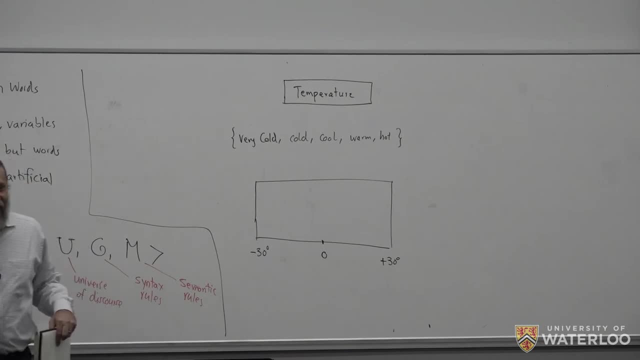 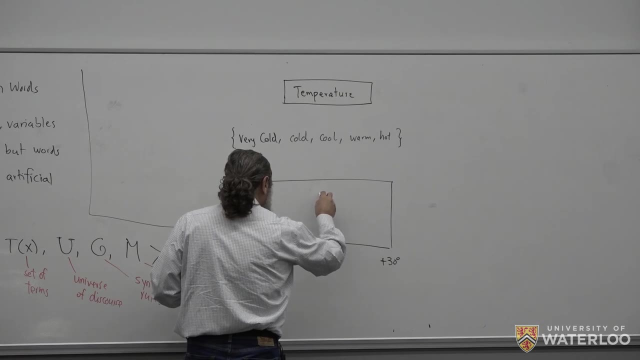 Usually things in reality are not symmetrical, not linear, They are nasty And then say, okay, so I don't know, Maybe so if I go for very cold, for example, it could be. but let me just start from the, from the center. 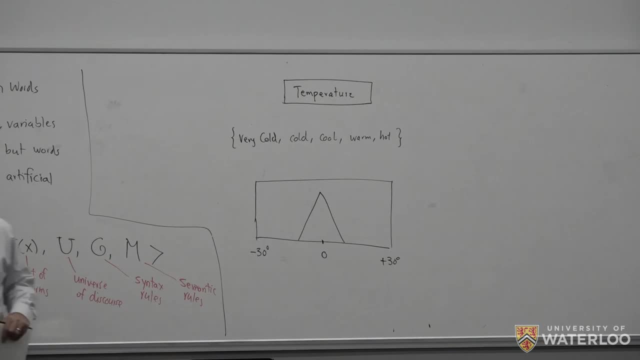 So if I put a triangle around zero, that means if you are at zero, this is a cool temperature for us in Canada. So if you go to Saudi Arabia, zero is not a cool temperature, It's an extremely cold temperature, because people are not used to it. 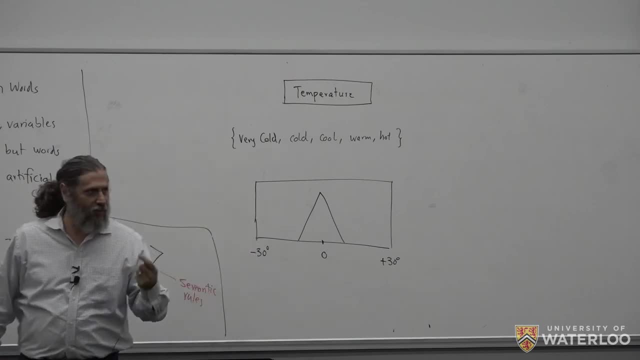 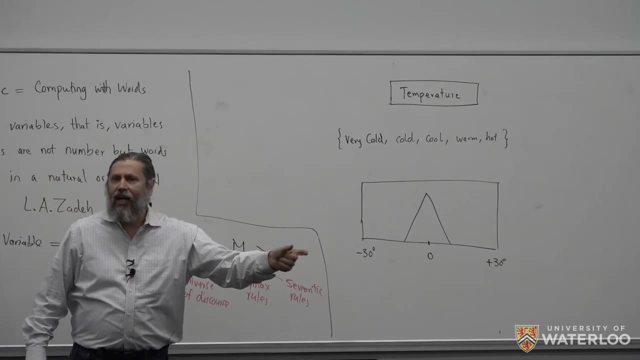 So, but for us you see the subjectivity of measurement. So when you, when you use, when you use linguistic variables, subjectivity flows in And then suddenly one word means something here and means something else in another culture because of the environment. 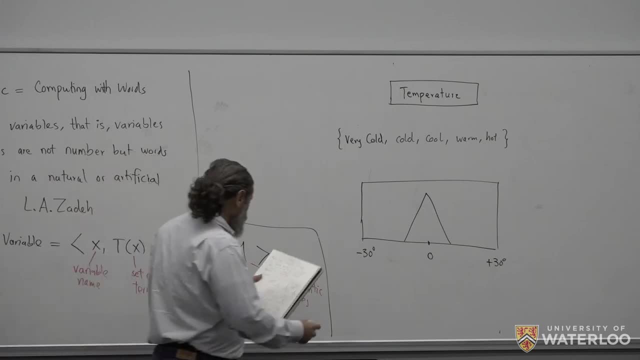 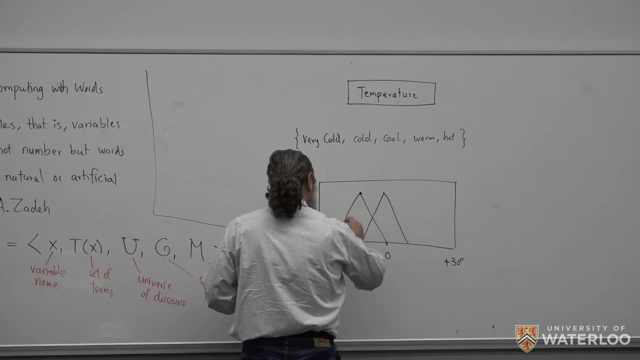 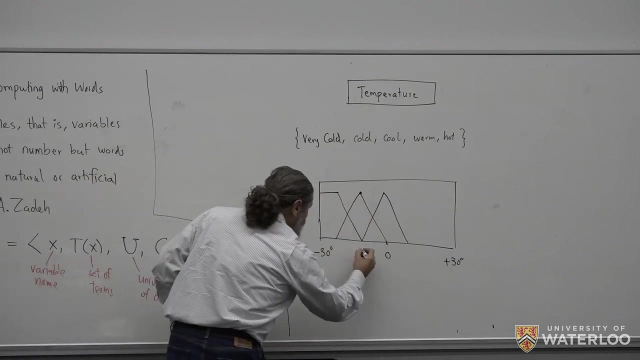 circumstances whatever, It becomes really human. And let's say: then I have cold, And cold is something like this, And then very cold is something like this. So if they let's say, if this is minus 10 degrees and this is minus 20 degrees, and this is minus 30 degrees, 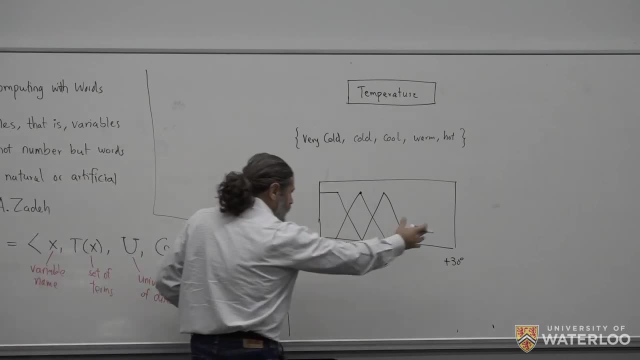 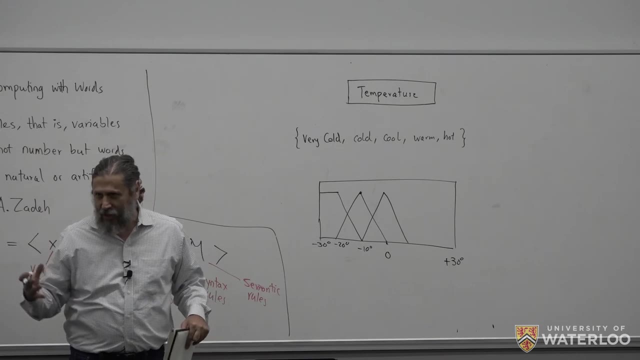 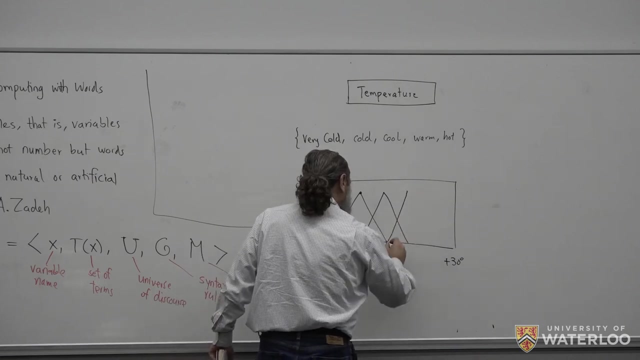 And I can go symmetrical. Again, I'm making my life easy. I'm assuming that the temperature perception by human is symmetrical And it's nicely distributed, which is not So, and then I have warm temperatures, perhaps, And I have hot temperatures of some sort. 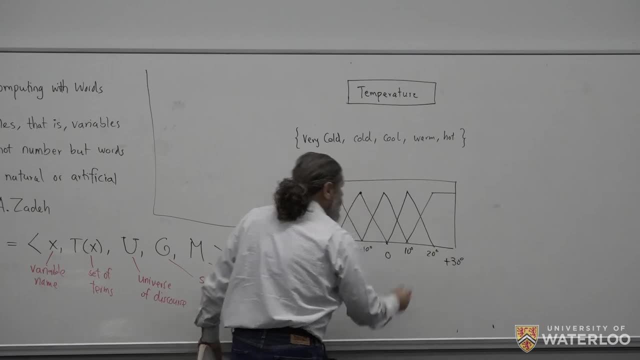 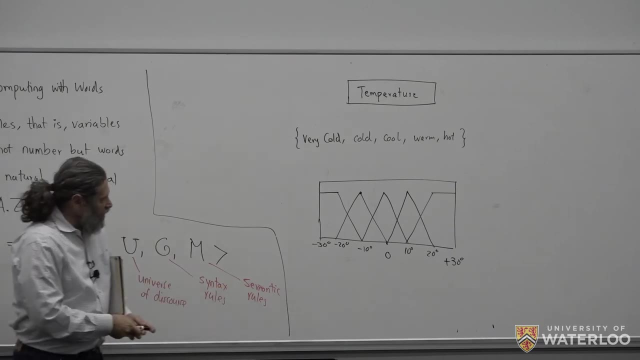 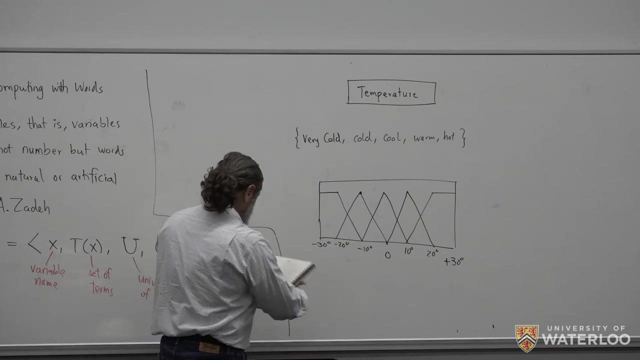 So let's say 10 degrees, 20 degrees, And then I have 30 degrees at that. So OK, What does that mean? First of all, if I see that? OK, so let me go to the end and then I come back and explain. 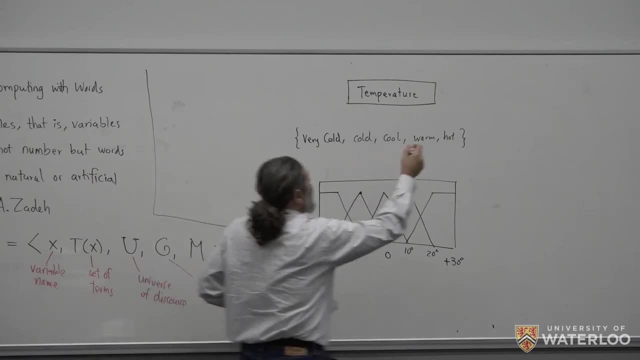 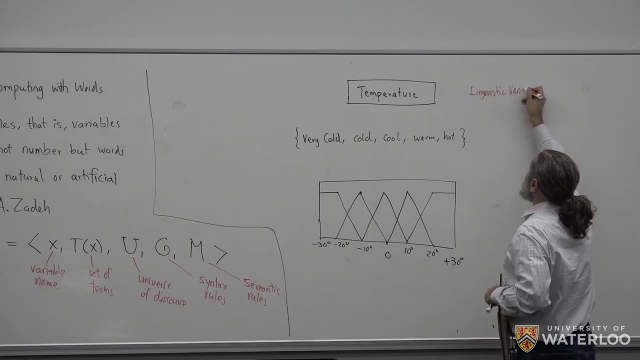 So, first of all, so this is your linguistic variable, This is the linguistic variable. The linguistic variable is temperature And this is our set of terms which, apparently, I chose subjectively. I chose them to be 5.. It could be 7.. 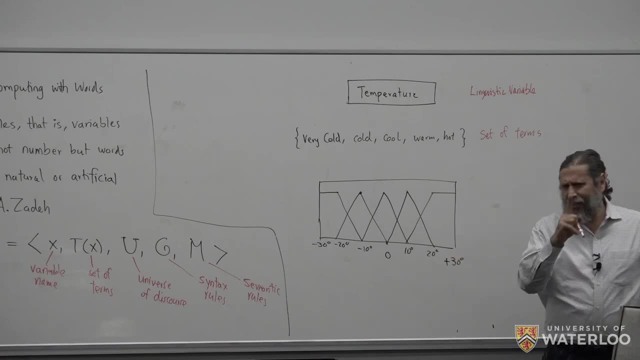 It could be 9.. Why is it uneven? Because it has to be something in the middle. There is always a middle, logically, So it has to be 5,, 7,, 9,, 11,, whatever, So we can say. I can start with extremely low temperature. 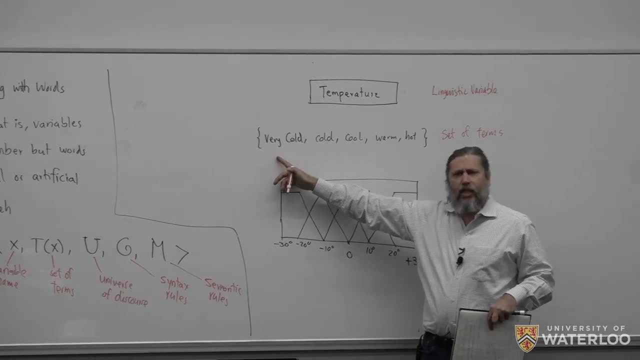 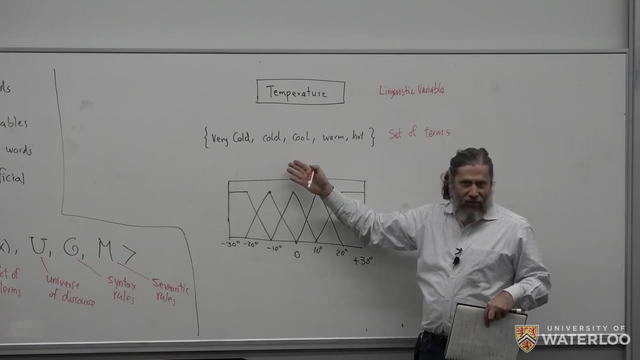 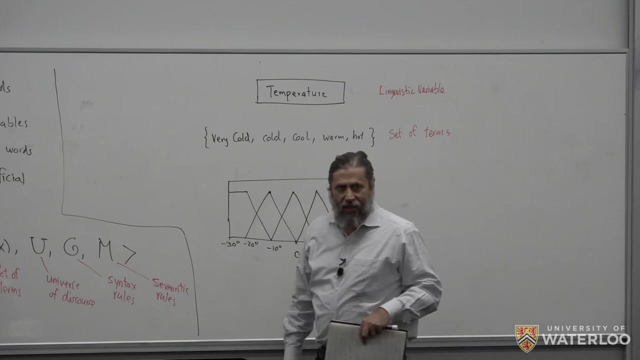 OK, OK, OK, OK, So we can say: extremely cold, Very, very cold, Very cold, Cold, Still cold, Cool, Not so cool. A little bit warm, Warmer, Warm, Hot, Extremely hot. You play with it. 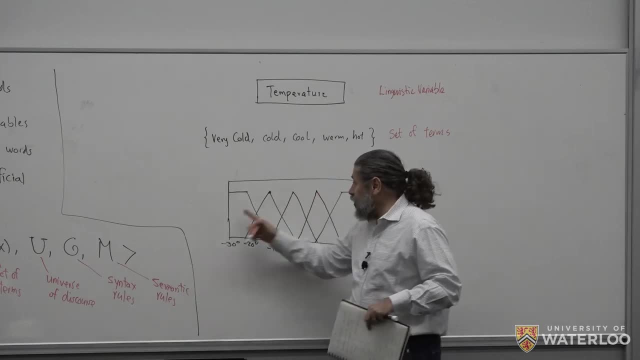 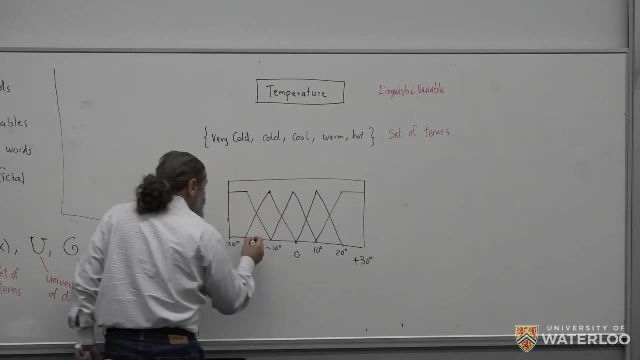 How much accuracy do you need? It's up to you. You pay the price because any function that you add, you are adding to the computation. So if you measure something, Let's say you measure minus whatever 23.. If you measure minus 23,. you see? 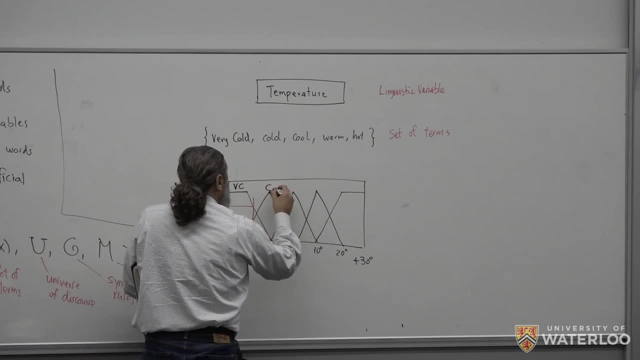 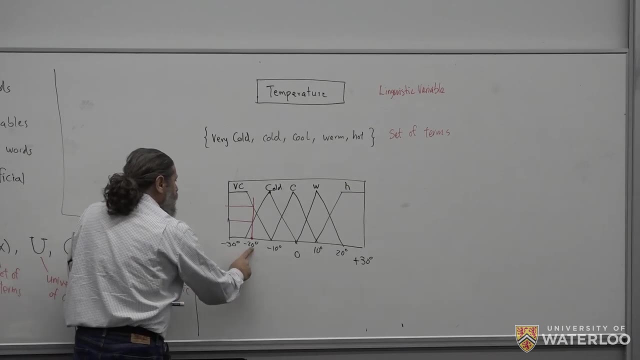 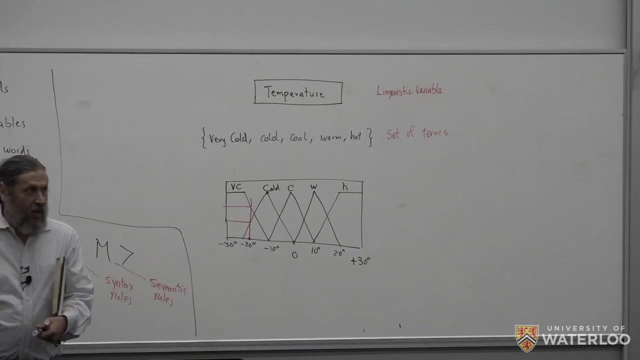 So this is very cold, Cold, cool, warm, hot. So if I look at minus 20, I see that minus 20 cuts two sets: Very cold and cold, Which means minus 20 is regarded very cold and cold at the same time. 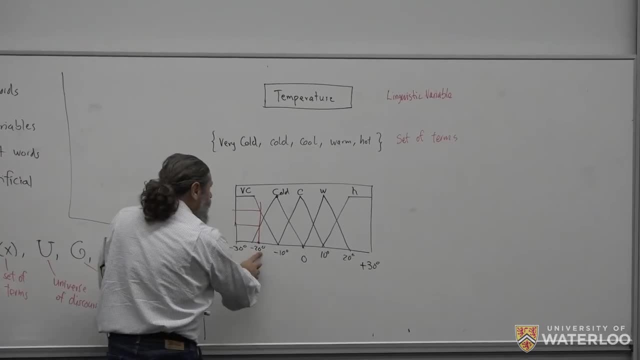 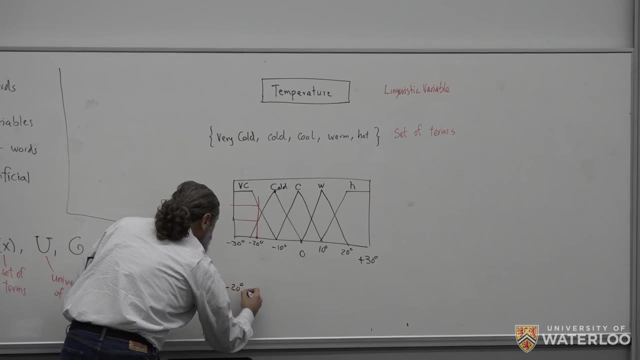 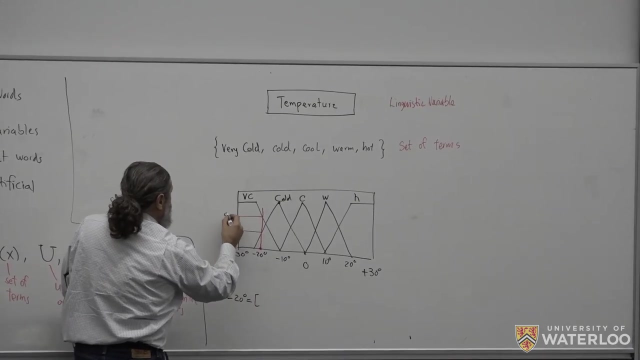 But minus 20 is not cool anymore. It's not warm, It's not hot. So if I write it So, minus 20 in language of Zadeh will be. So let's say this is 0.75 and this is 0.4,. let's say: 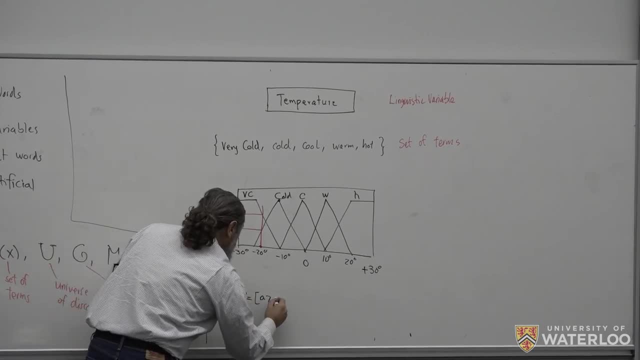 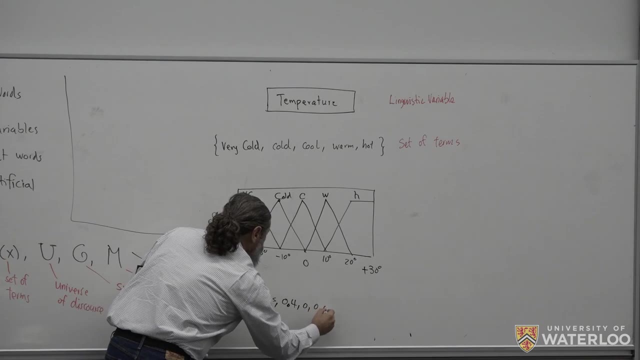 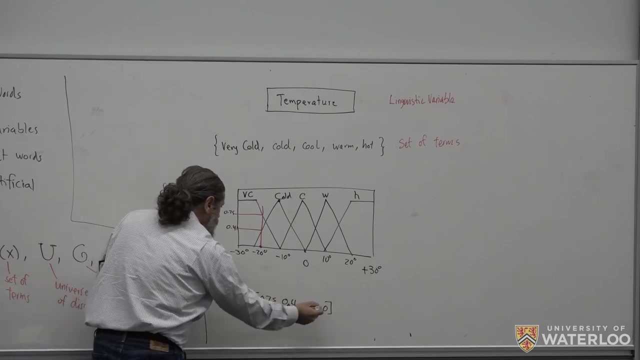 I don't know. So it would be 0.75, 0.4.. OK, OK, 0, 0, 0.. So 0.75, 0.4, 0, 0, 0, which is very cold, cold, cool, warm, hot. 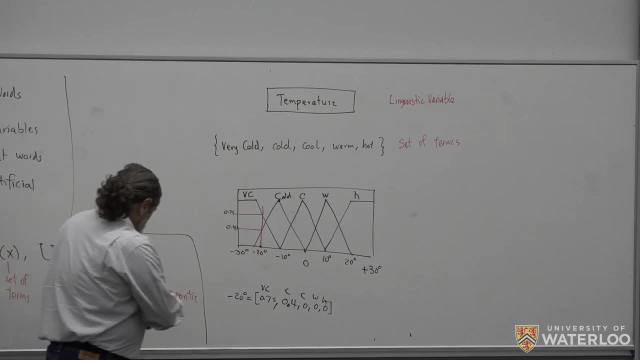 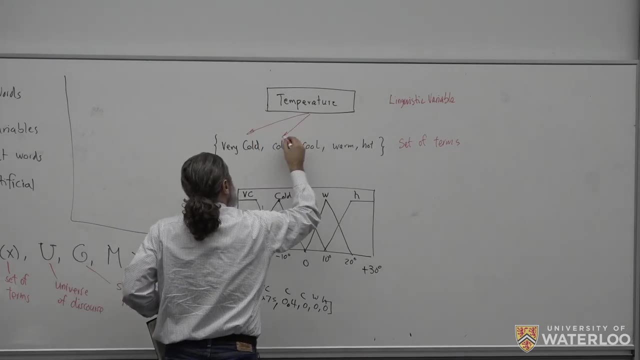 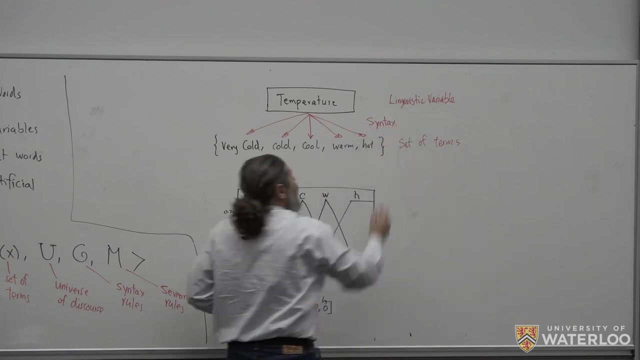 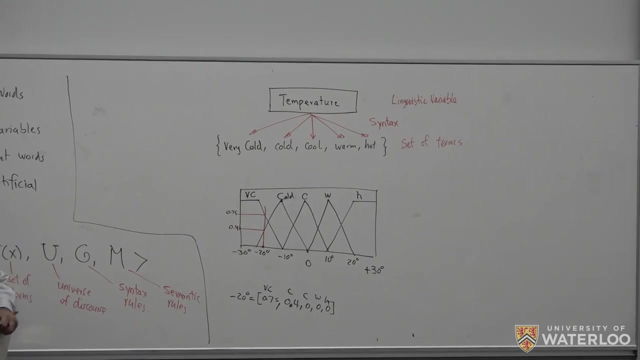 OK. So of course, In order to assign this temperature to some terms, You need some syntax. So you need some syntax rules to say what is what If I say temperature, which part of it is very cold, which part of it is warm? so how do? 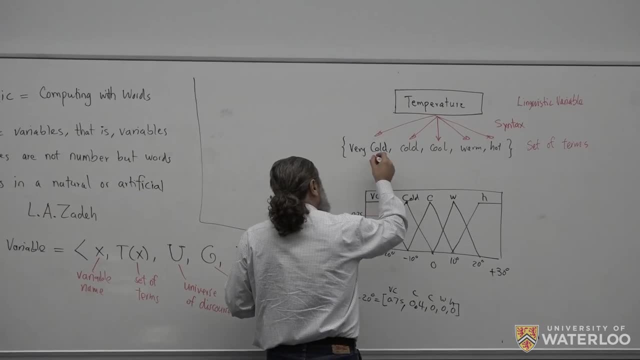 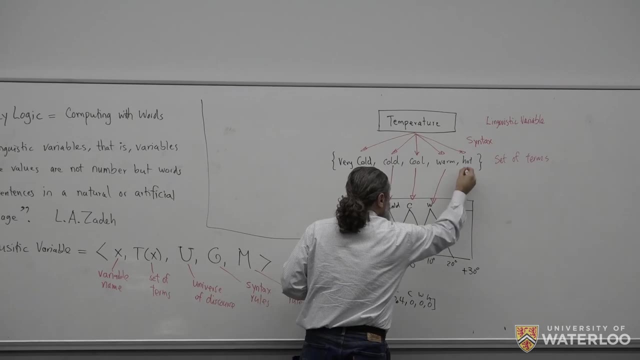 you assign the syntax To come from the term to the actual value. You need some syntax. Sorry, Mind, this is a problem. How do you assign the Amsterdam's? How do you assign the Amsterdam's from the Bastion? Why 對不對? 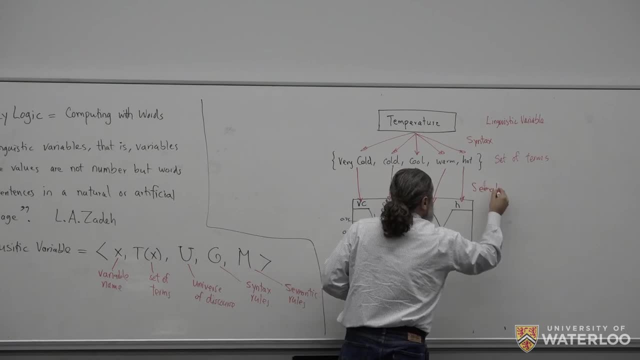 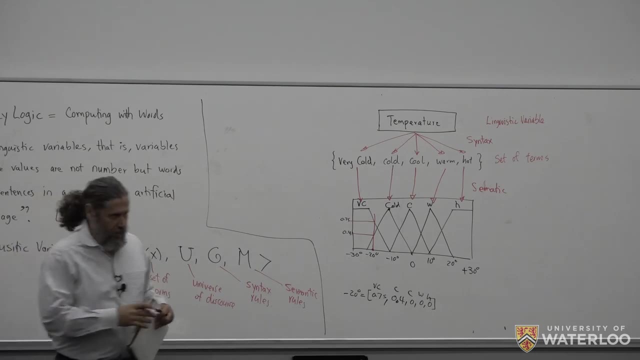 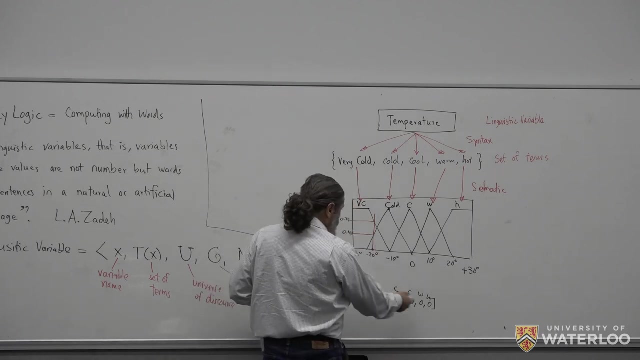 Exactly. Oh, sorry, Yeah, some semantic. So what is the meaning? What is the meaning of very cold, if I want to measure it? Yes, They should add to one. Maybe I used something unnormalized, but they should add to one. You're right, But you don't have to It. 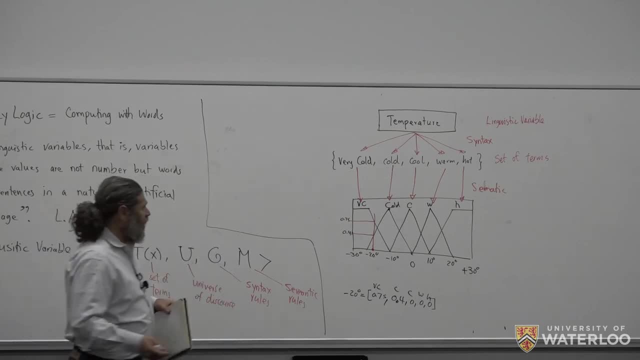 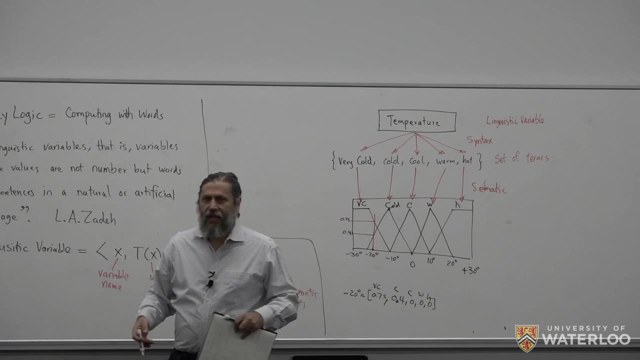 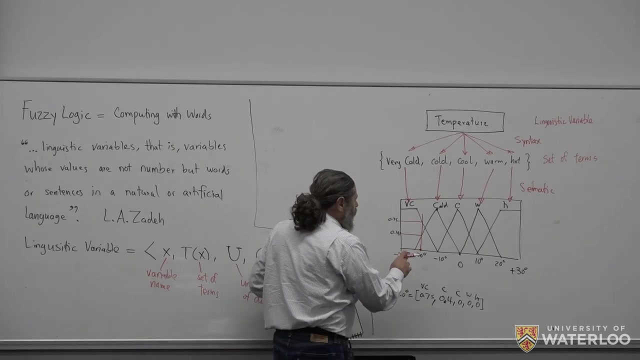 makes life easier, but you don't have to. But if I draw something really beautiful like this, symmetrical, and this is one, they should add to one. So, unless they are non-linearly distributed, So okay, And when I come here? so these are my. 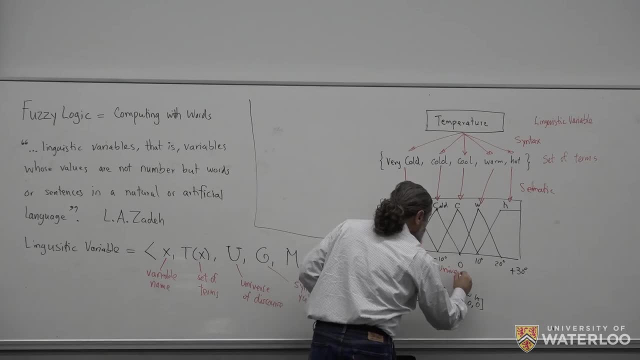 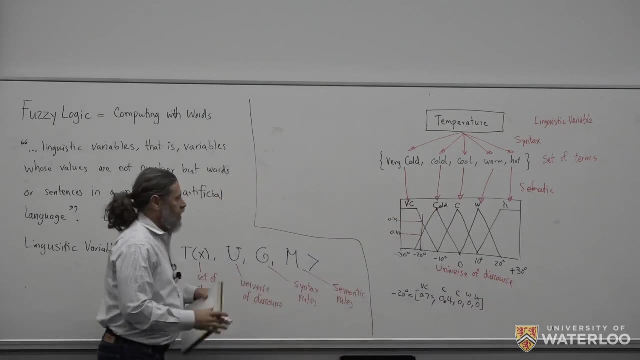 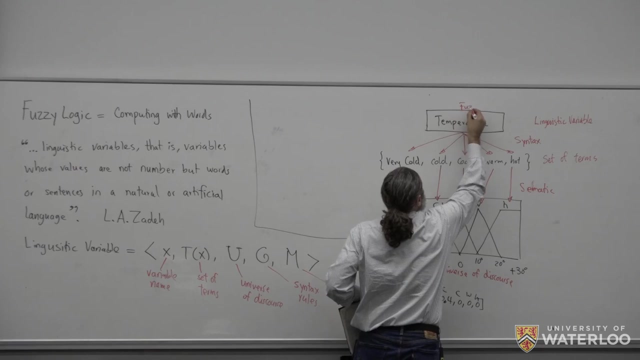 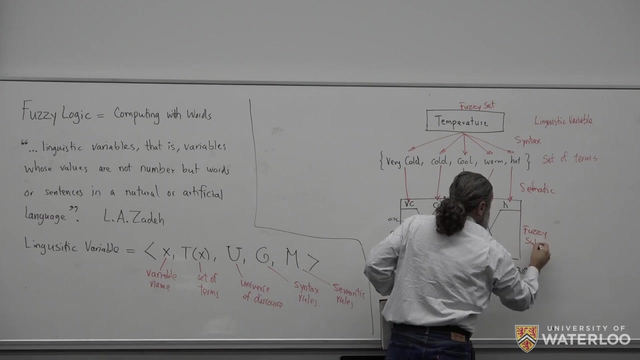 membership functions, and this is my universe of discourse. So this is a set of all variables that I can calculate. So this is actually. this is a set of all variables that I can calculate. So this is actually. this is the fuzzy set and these are the fuzzy subsets. People mistake that They show you a fuzzy. 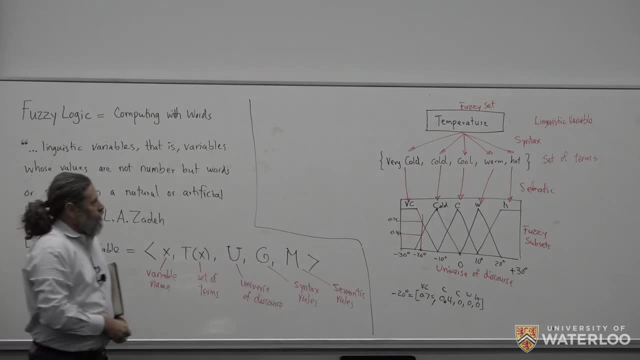 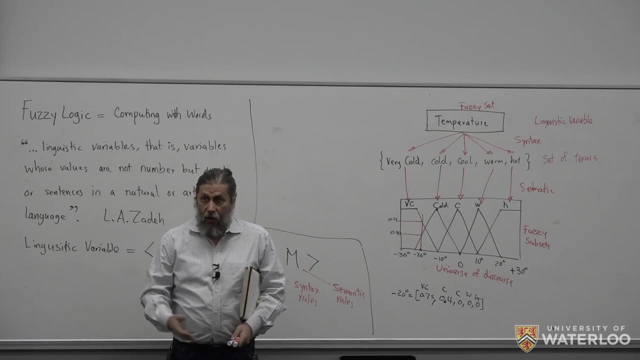 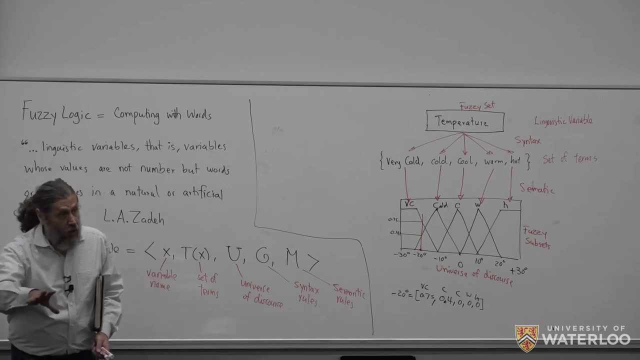 subset and talk about a fuzzy set. So okay, So what? So what You know? You know what you just did by defining a linguistic variable, By giving the variable name a set of variables, A set of terms, some syntax rules, some semantic rules and the universe of discourse. So 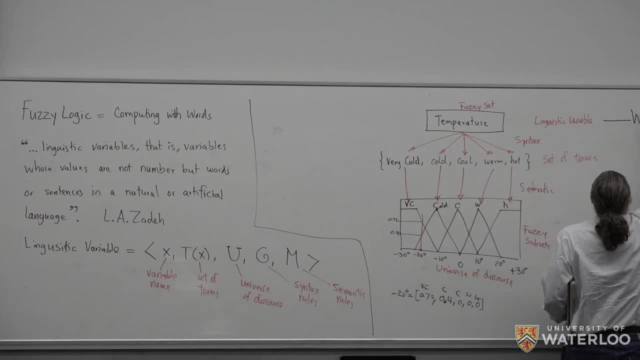 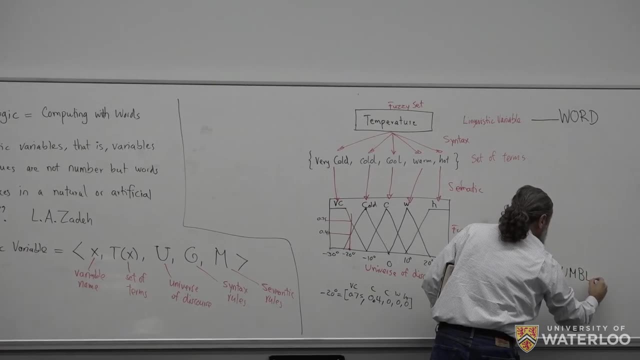 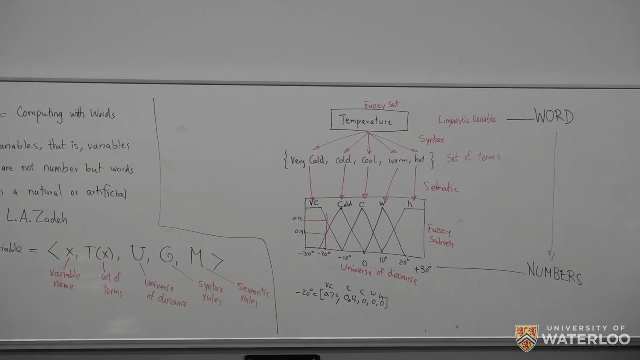 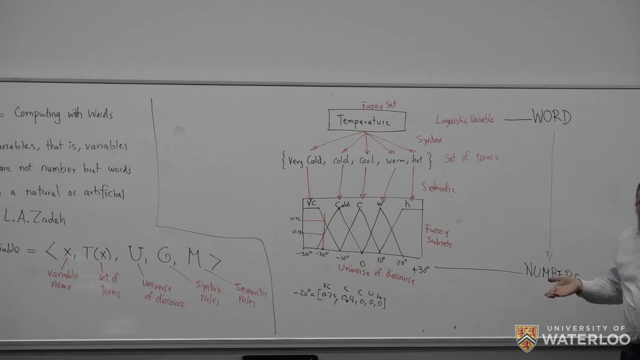 here you have a word, Here you have numbers. This is what fuzzy logic does. Fuzzy logic gives you a bridge between words and numbers. Why? Because at the moment our computers are stupid and they cannot process words. So whatever you give me in. 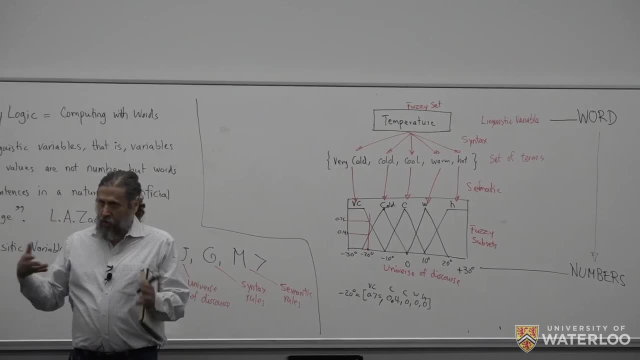 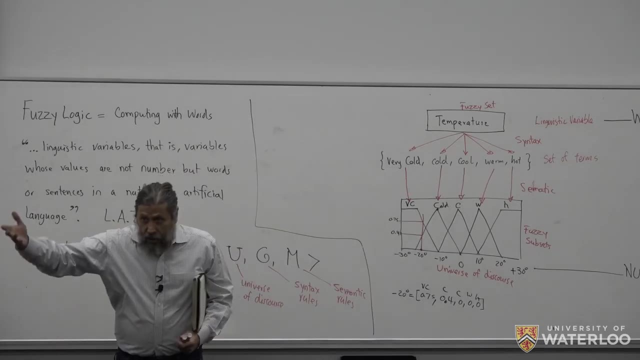 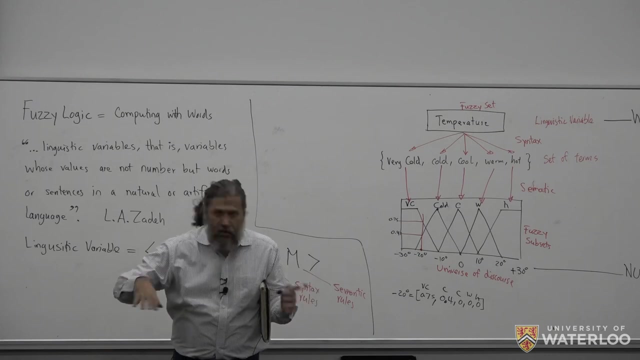 terms of linguistic information and linguistic knowledge. I have to convert it to some numbers such that the computers can process it- And, in general, NLP, which usually we don't include, fuzzy logic, because fuzzy logic is unfound. triple of the AI. 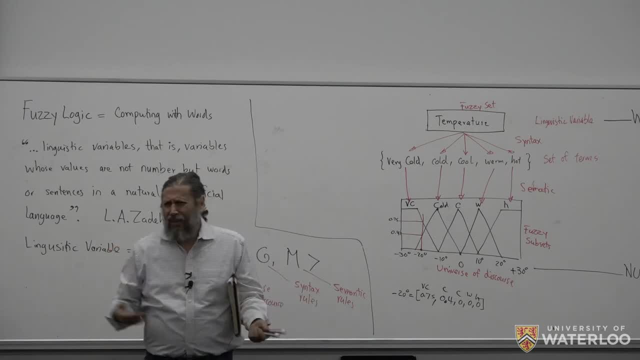 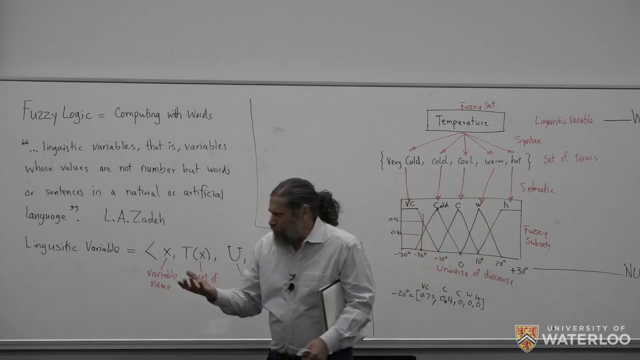 still, many of us in AI don't like fuzzy logic. I don't know why There's some weird stuff going on. I don't know. Maybe it has something to do, I don't know Whatever. So we don't want to see this as part of NLP, and it's not, I would say, because it gives you something. 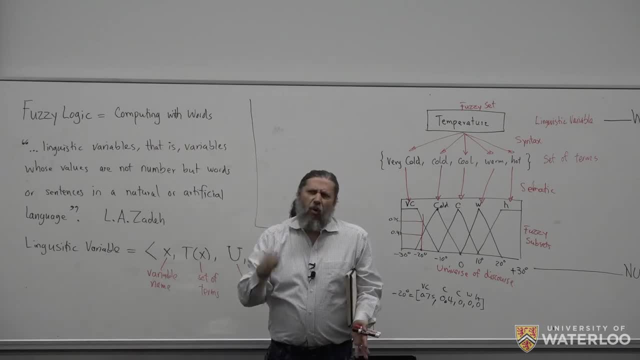 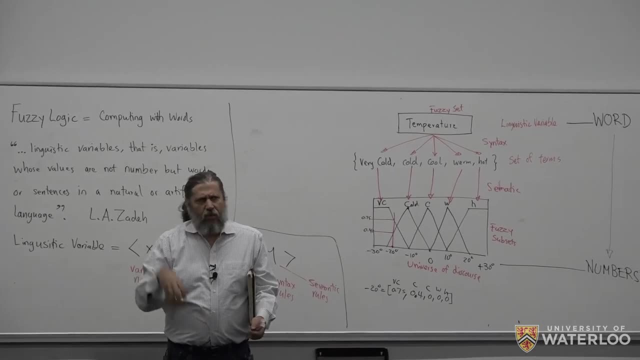 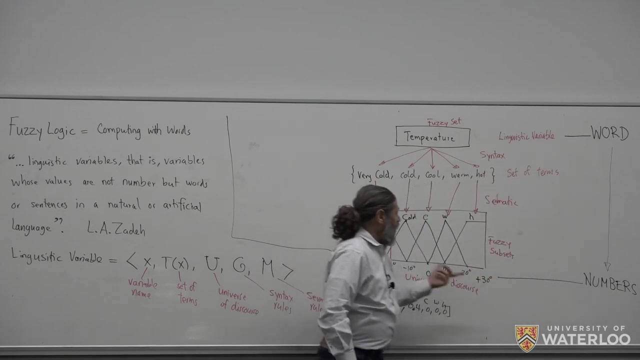 actually quite unique. At the moment, we cannot really exploit what fuzzy logic offers, And because our computers cannot process words. So what, at the end of the day? so fuzzy logic can give? you can be as accurate as you want, and only one thing. 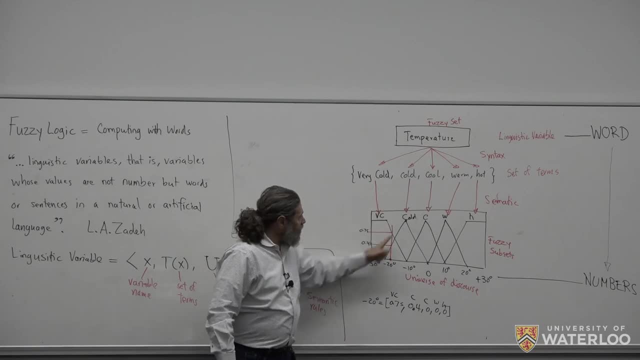 changes The size of these terms, which is these membership functions of the fuzzy subsets. If you want to have a super precise answer, you go with 111 membership functions, not with 5.. We will see an example today that it would cost you a lot of computation if you increase. 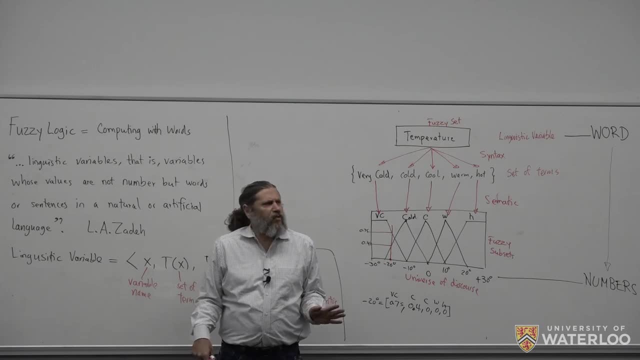 the number, But for the first time, actually, fuzzy logic was one of the first techniques that gave us the choice. how much accuracy do you need? So, no, not much, I just need a rough estimate. Okay, go with 5 or 7 membership functions. No, no, no, I need high, accurate. 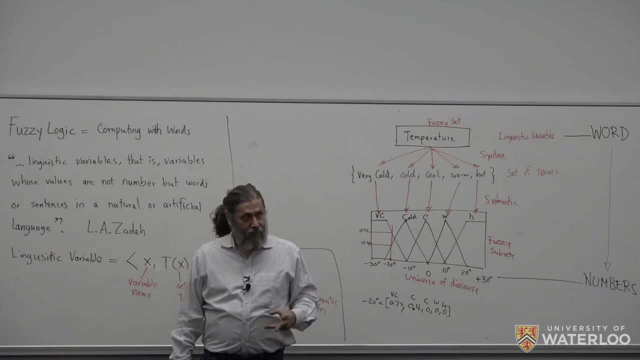 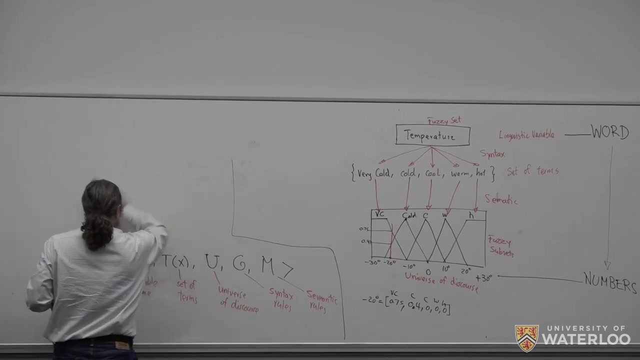 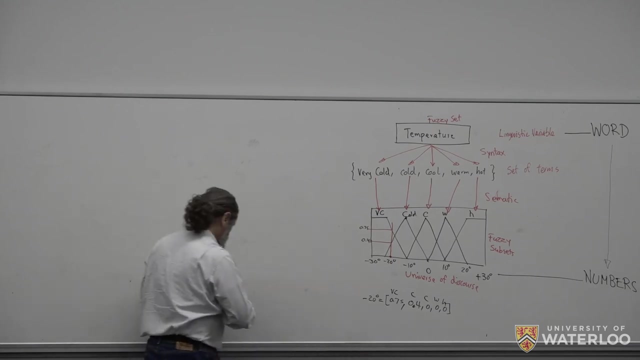 results: Okay, go with 25.. So So. So We said that there was a difference between fuzzy sets and classical sets, which are a subset of fuzzy sets. Maybe that's what people don't like. So, because we know that the classical sets, the yes and no sets, 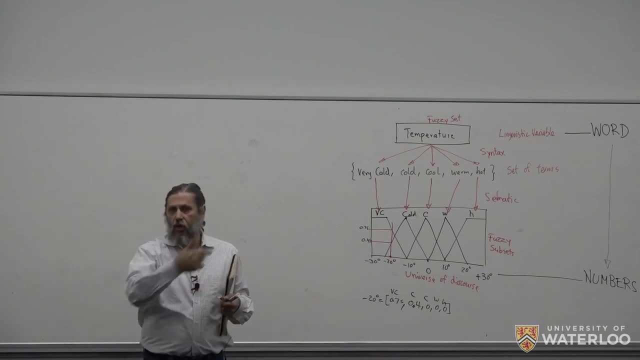 the Boolean sets- the true and false sets are a special case of fuzzy sets And if you are working for 50 years and you're using a theory and then somebody comes and says your theory is a subset of my theory, people get upset. 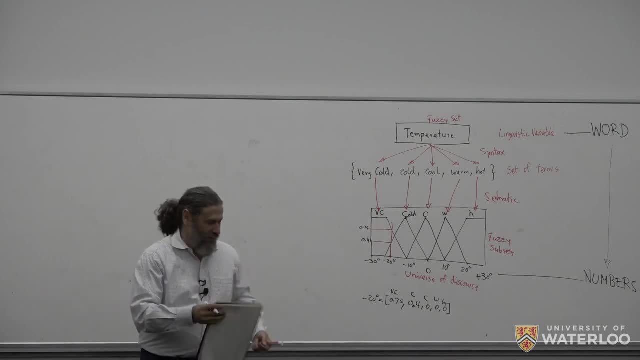 Most of it is ego. We get over it When the guys who invented that died, and after 20 years, and then we realize, oh my God, he was so smart. Okay, We said that the classical set is the set of variable X, such that X of course comes. 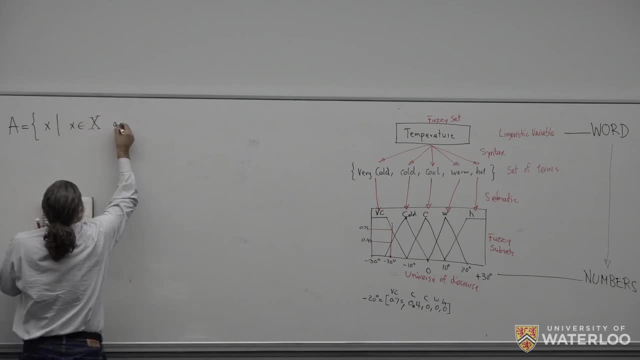 from the universe of discourse. X and X is something. X is delta, X has some property. So that's how classical sets are defined. Anything you come up with is a set. Anything can be understood and formulated as a set. So X come from templates. 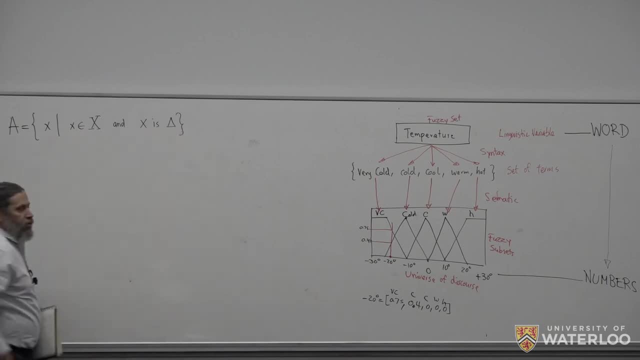 X is temperature and X is very hot temperatures. X comes from the set of old men and X is a very young man. Anything you want. So anything you want is a set. Now, if I want to define a fuzzy set, we sort of hinted to this. 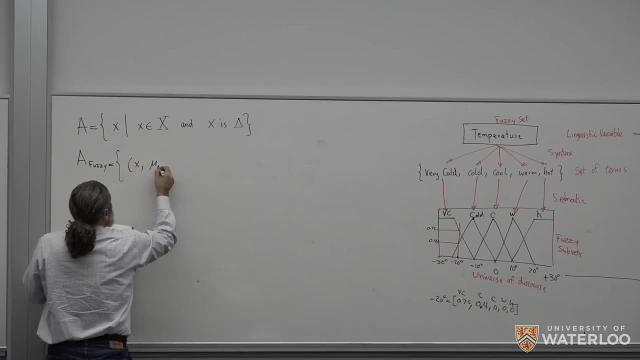 First of all, you cannot just go with X. You also need to give me A membership function- mu of A, mu of X- in the set A. So for every element that you are giving me, you have to give me a number between zero and one. 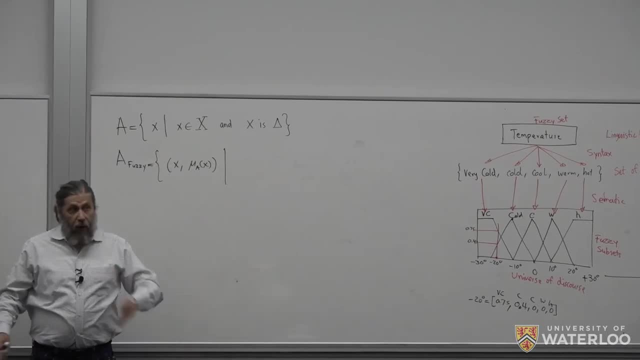 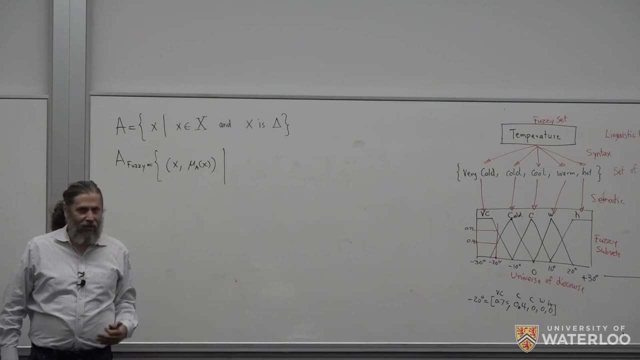 Because here, everything that you list is a member, Everything that is not there is not a member. Why do you think digital technology is so everywhere? Because it's so simple: If I list it, it's a member. If I not list it, it's not a member. 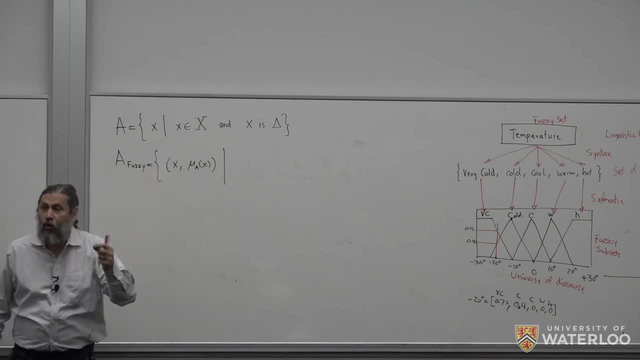 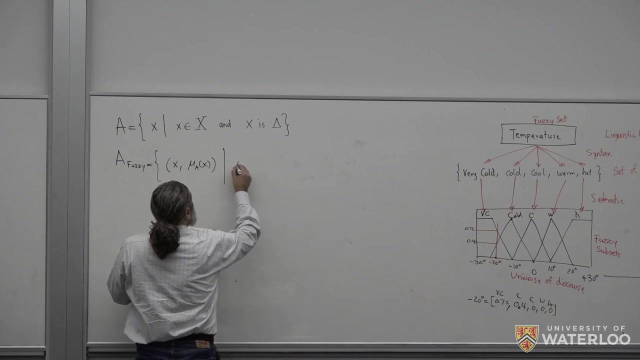 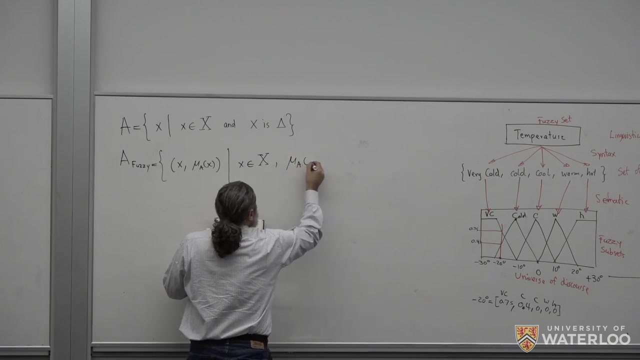 Here. For every X, I have to tell you to what degree it's a member. That must be exhausting, Yeah, but if you want to have a more realistic model of the world, maybe you have to do that. So and again, of course, X still is coming from the universe of discourse. 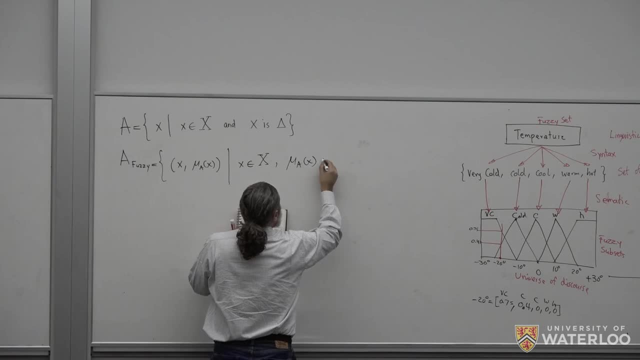 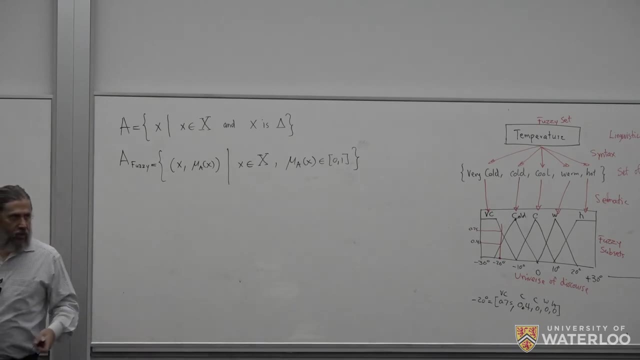 And the membership function mu X of A belongs to X, The closed interval, zero and one, and we talked about this. we violate two rules: Blasphemy, bad people, we don't use this theory, and so on and so on. 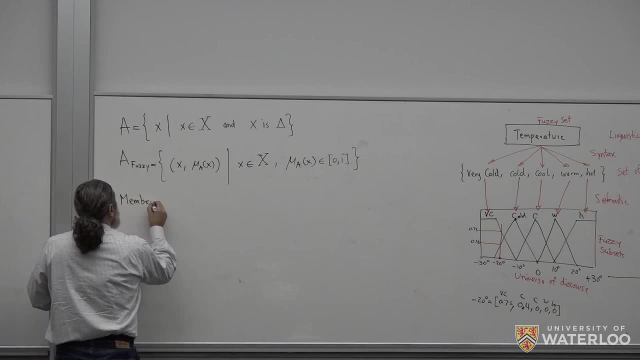 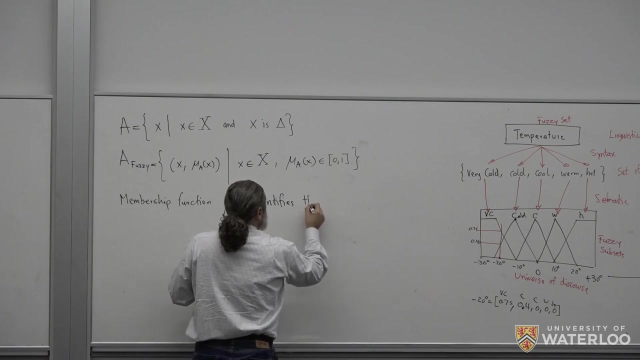 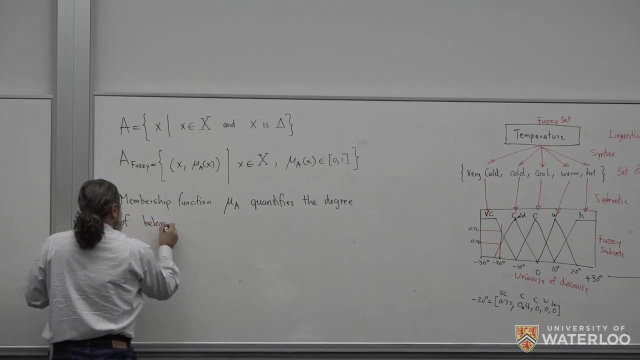 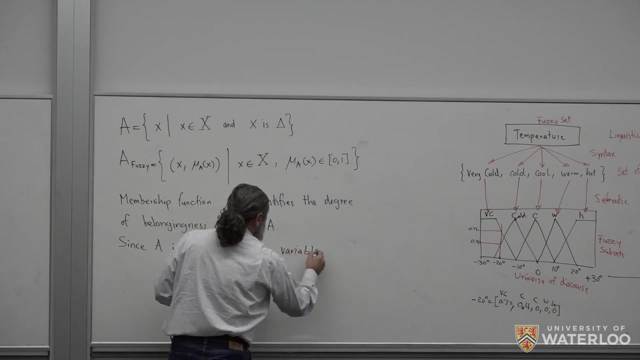 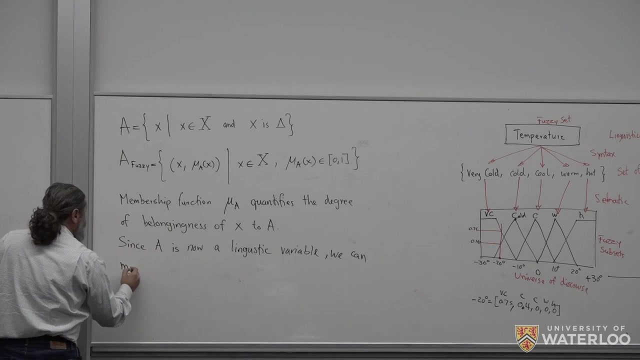 So the membership function, The membership function, mu, A, Quantity, Quantity, Quantity, Quantity, Quantity, Quantity, And that quantifies the degree of belongingness. if this is a word of X to A, Now, since A is now a linguistic variable, we can modify its meaning. Okay, What is that supposed to? 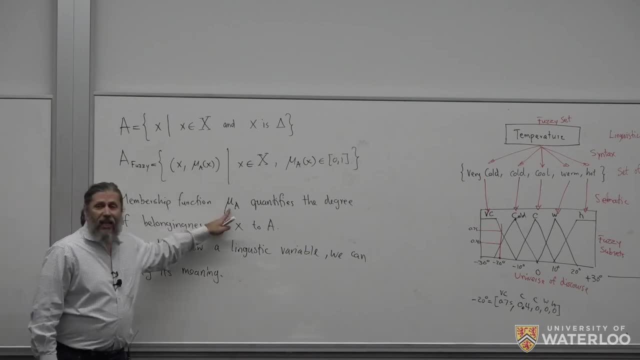 mean. Well, we talked about it that usually that mu A, which was in dual binary logic, Boolean logic, was an F characteristic function and is either 0 or 1. Either you are a member or you are not a member. Mu is a matter of degree, So you can get any number between. 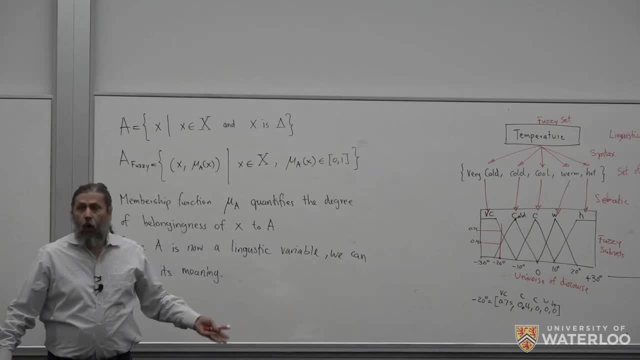 0 and 1.. And if you're looking at the set of old men, hopefully I'm not a member of that set with membership of 1. Hopefully you caught me a slag and say, okay, you belong to the set of old men with a membership of 45%, The rest is open. You can still feel. 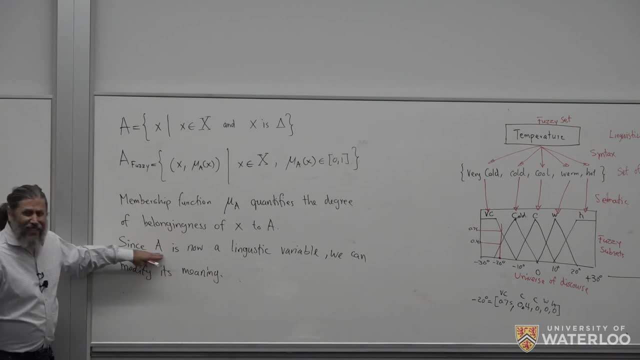 young. So but if that set is regarded as a fuzzy set, then it's a linguistic variable And any linguistic variable can be changed. The meaning can be changed. You say hot and very hot, Old and not very old. Look in the logic. if you have a statement, if 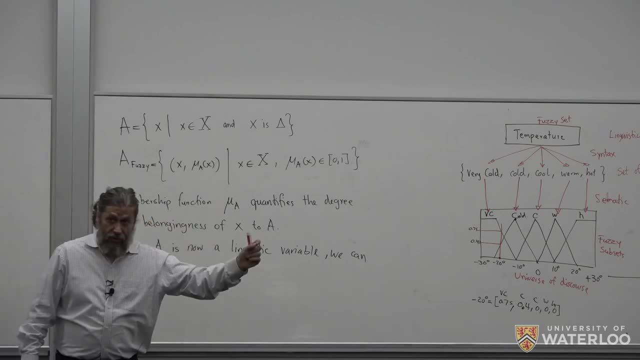 you have a knowledge about old people. that's all you know. If somebody says I know something about not very old people, you have no clue what he's talking about, Because you can only talk about old people, not very old people, not extremely old people, just old people. 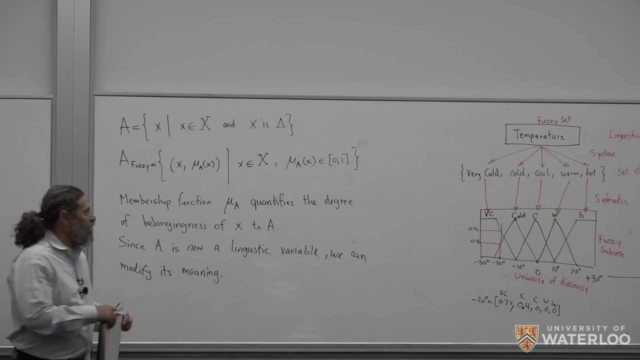 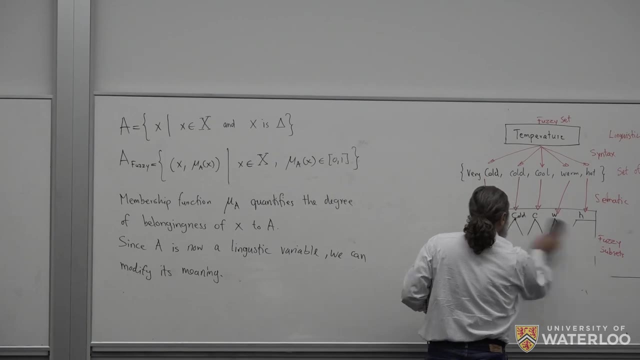 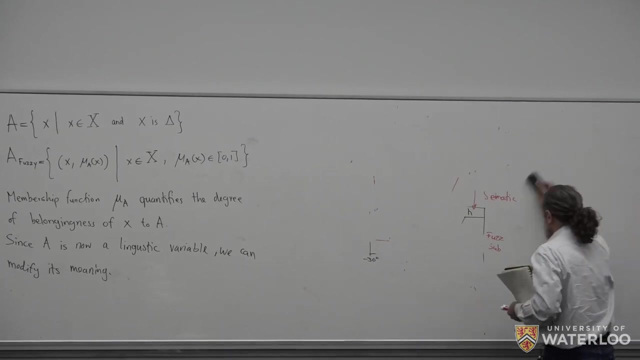 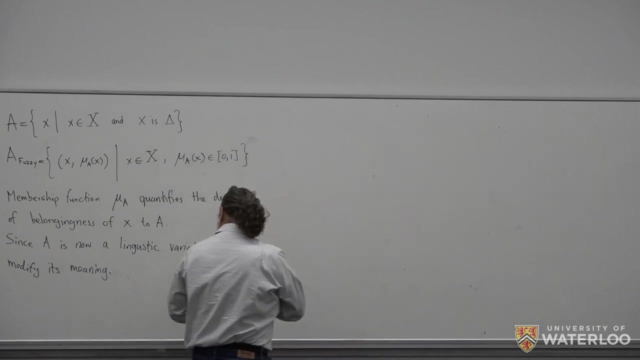 Because we don't have a logic. We don't have a logic, We don't have a logic, We don't have any way of modifying the meaning of those words because they are not in the classical logic. they are not linguistic variables, They are binary functions. Okay, So if I look 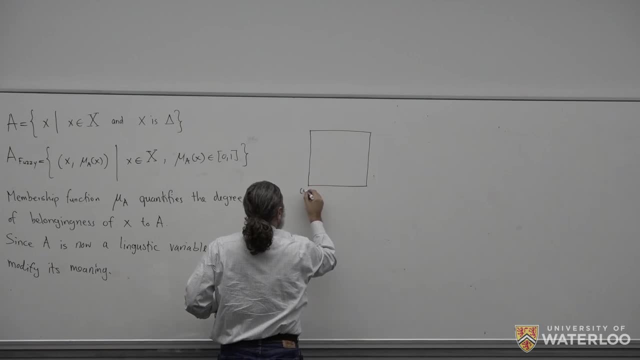 at this, Okay, At my 00101001,. let's say: this is my A, This is my fuzzy set or fuzzy subset. Whatever that means. It means sunny day, It means a young woman, It means bright light, It means 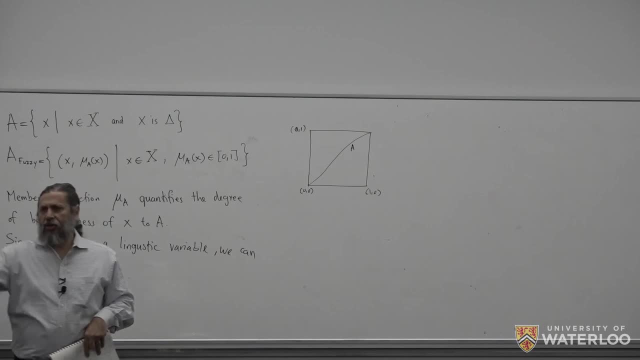 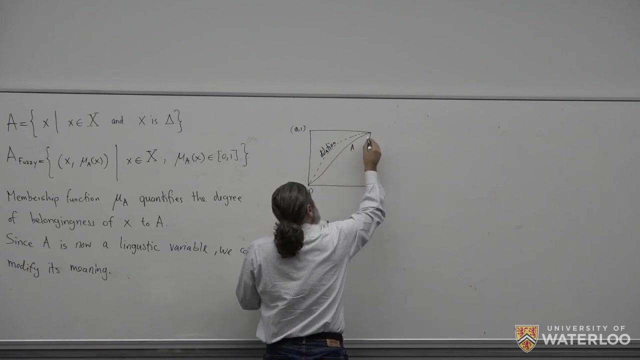 hot temperature. Whatever it means, It doesn't matter what it means. We can dilate this function, So dilation. Or we can concentrate this function, So concentration, And then hopefully that means something. Okay, Okay, Okay. 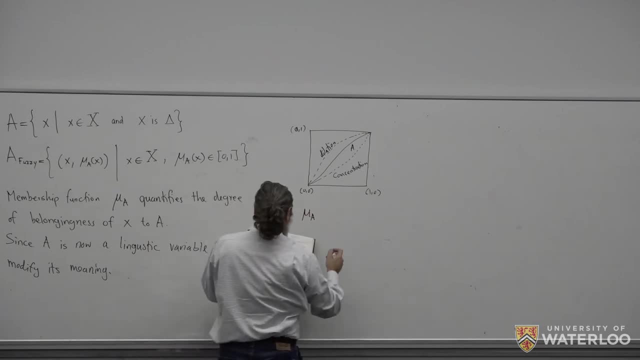 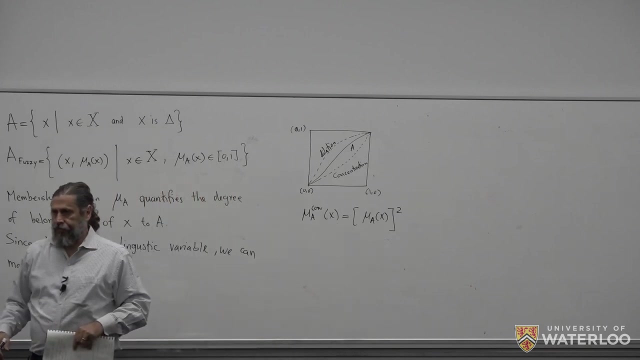 Okay, Okay, Here I have mu A, So mu A concentrated of X will be, for example, mu A of X raised to power 2, because the numbers are between 0 and 1. If I raise it to 2, I suppress them. 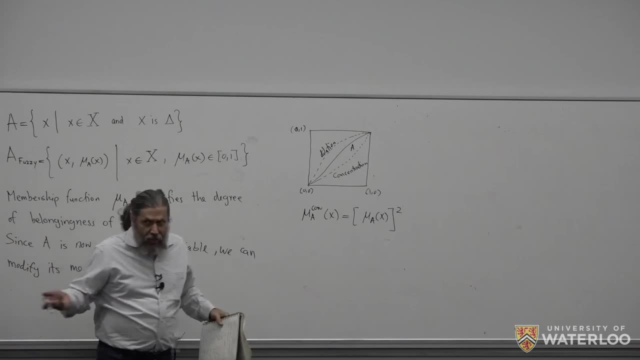 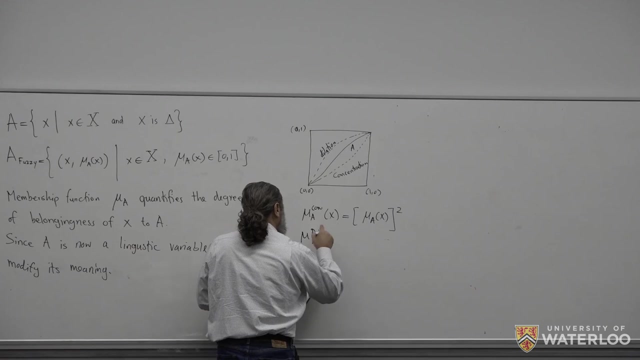 So I compress them So big deal. What do you think probability is? You just count, divide by number of total frequency. big deal. But see how much we do with that philosophy- a lot. So then the mu of A dilated dilated of X would be mu of A of X raised to half. 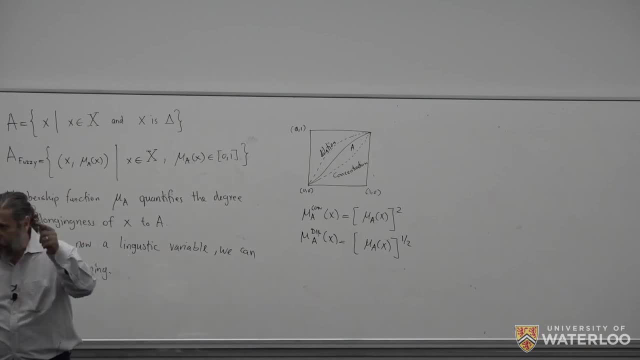 So then, because the numbers are between 0 and 1, if I get the square root of that number, the numbers will be higher. So I dilate the values. So, okay, what does that mean? Okay, So let's say mu of A, mu A is known. 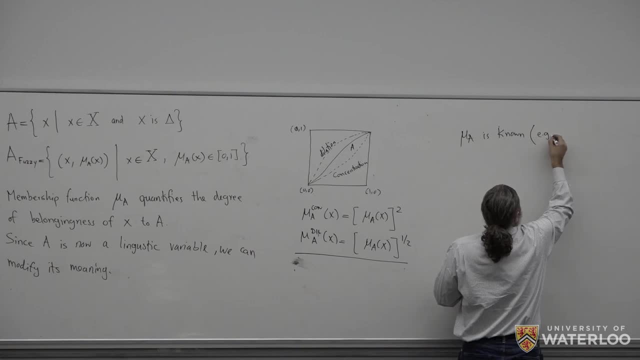 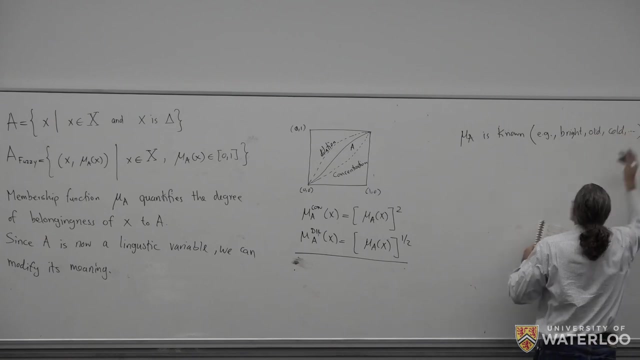 For example, bright cold, bright, old cold, whatever adjective you want to use. So you know, mu A, You have some measurements, You know what is the perception of people: Who is an old man, Who is an old guy? 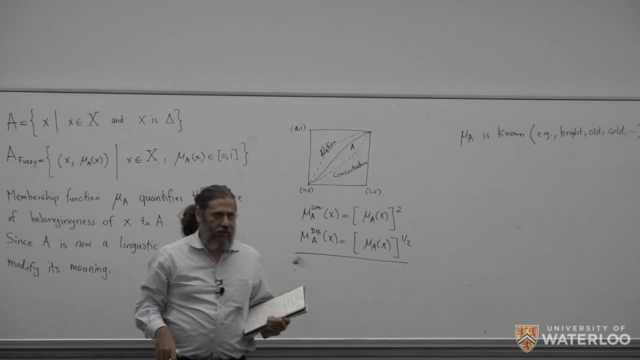 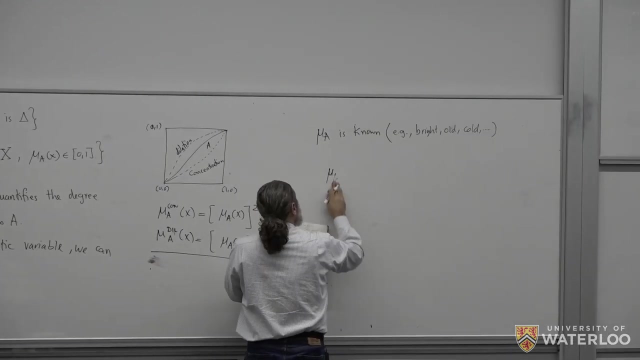 You know what is the perception of people: extremely cold in Canada, Minus 55, that's extremely cold. So you know that. Okay, If I know that, what is the membership of? sorry, what is the membership of very A? 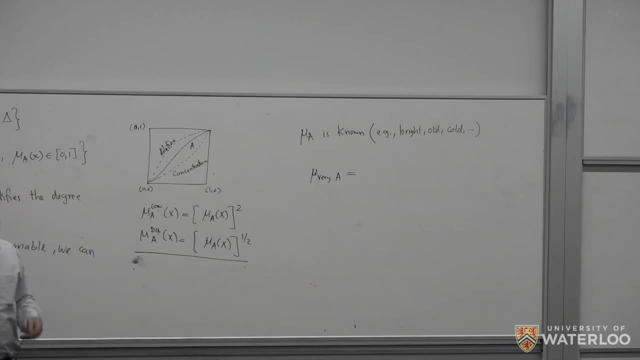 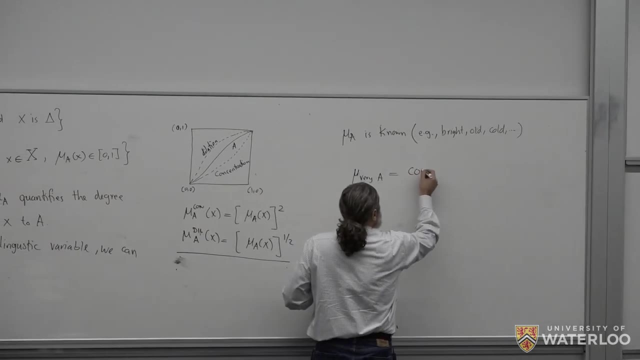 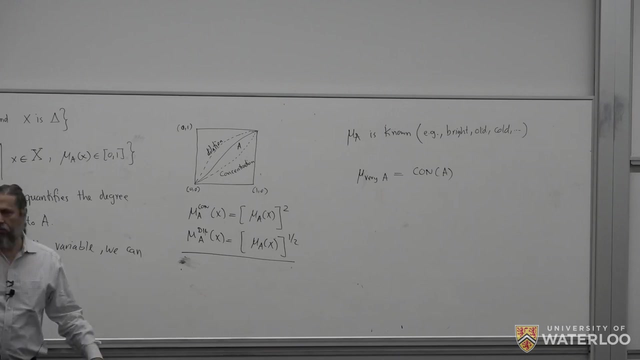 whatever A is So very bright, very old, Very cold. What is that? membership? You can do it as the concentration of A, So our concentration being defined this raised to power 2.. Why raised to power 2? It works. 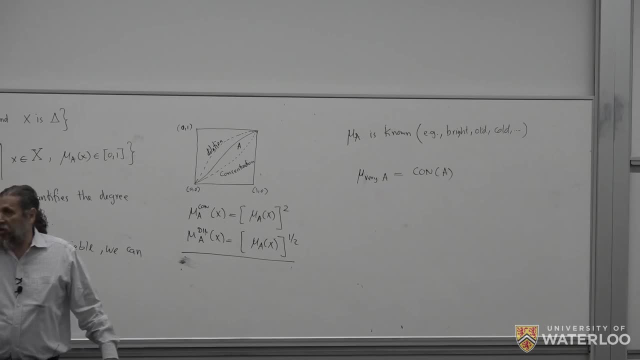 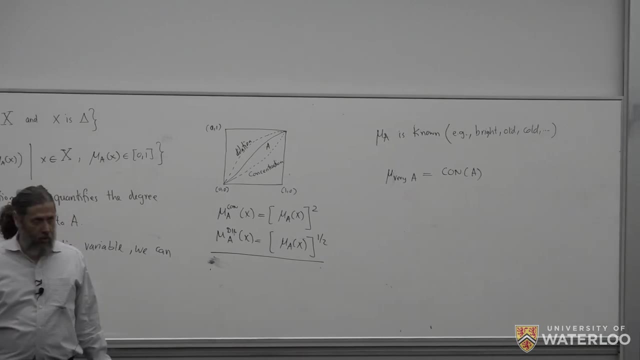 It doesn't contradict my intuition, I'm going with it. Deal with it. But it could be also 1.9, yeah, or 2.1, yeah. What's your point? So you have a lot of degree of freedom, yeah. 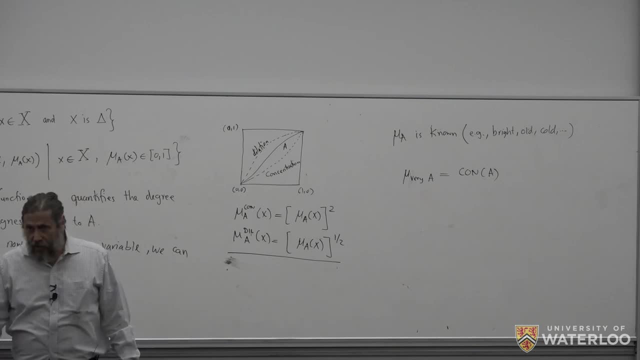 Like the reality. In the reality you have a lot of degree of freedom. Get two people together who agree what exactly means to have pleasant temperature. Is it 21?, Is it 22?, Is it 23?, Is it 24?? 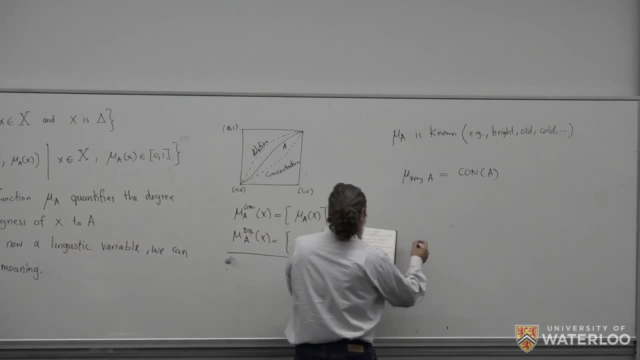 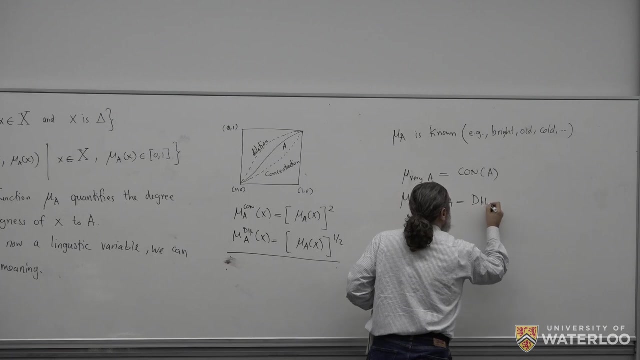 There is a lot of vagueness. What is the membership of more or less A? Okay, Well, that could be the dilation of A, Dilation of A More or less A. What about? what is the membership of very, very A? 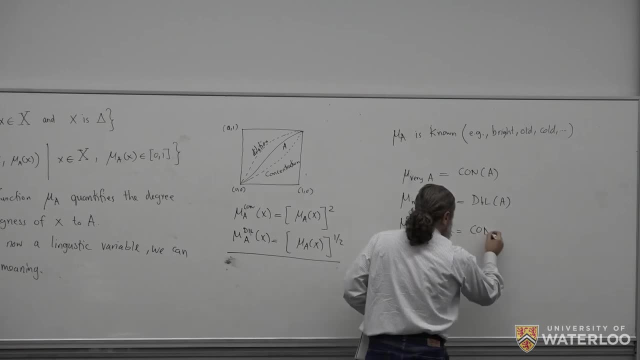 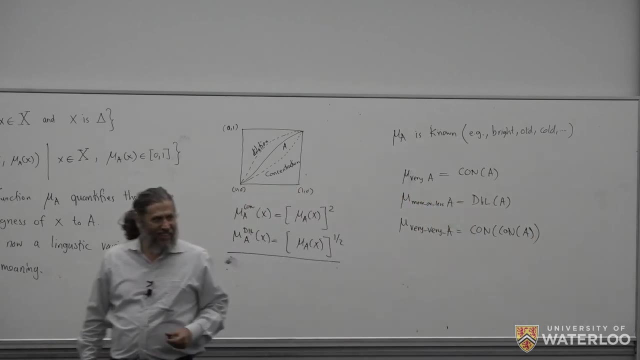 Well, it could be the concentration of concentration of A. So what is very, very old? So I take it power 2.. So if my membership to the set of old people is 80%, my membership to the set of very old people cannot be more than 80%. 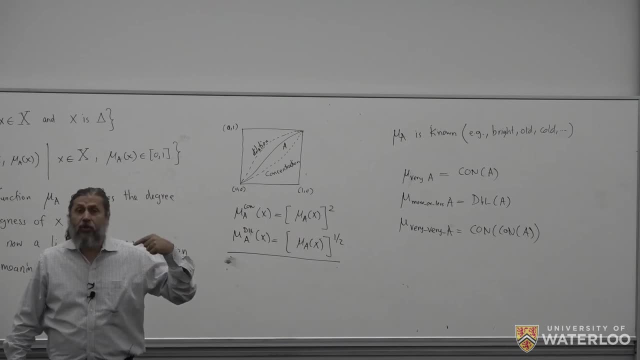 It has to be less, Okay, And my membership to the class of very, very old people has to even be less than that. So it's all about subjective perception, Of course. What did you think Fuzzy logic is about? how can we model human thinking? 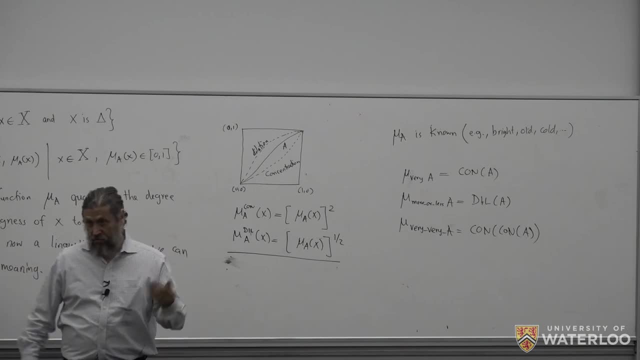 And human thinking is a mess. It's a lot of ambiguity, a lot of granularity, a lot of vagueness, a lot of subjectivity. I say this: You say that Nobody can agree. We do some. statistic Is 23,, 23, the perfect temperature. 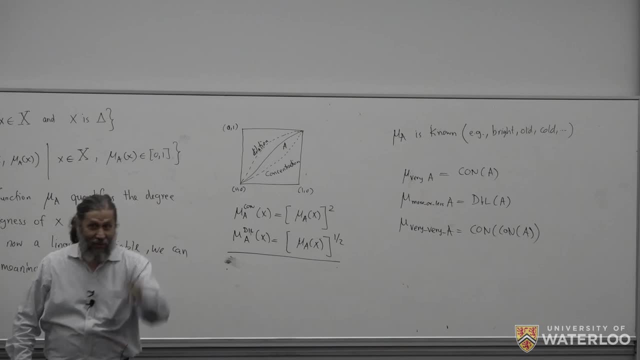 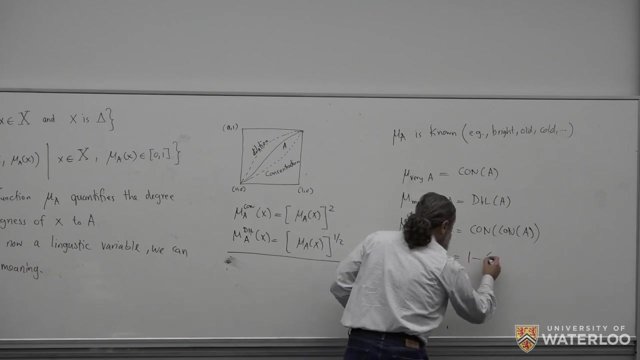 Plus minus 80%, 8 degrees. So a lot of variation. So what about the membership of not very A? Well then, I would go with 1 minus concentration of A Not very A. So I'm slowly getting at an idea. 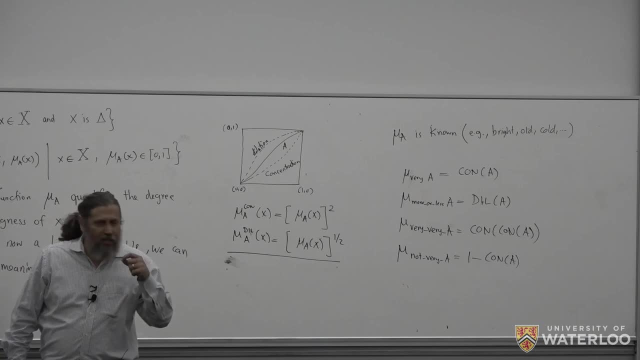 Oh my God, If I understand normalized functions as fuzzy subsets, I get a lot of flexibility. I still don't know what it's good for. I can write it on the board and just feel good about it, But if this is going to be useful, we have to be able to do something substantial with. 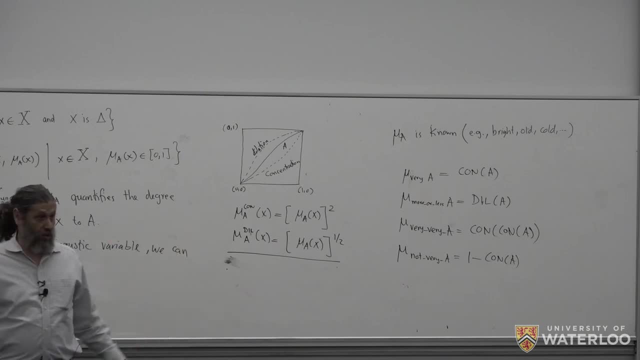 it. If I cannot do I don't know, function, approximation, classification, some sort of learning. if I cannot do that, I don't care. I did. But it looks nice And it's amazing that suddenly from old I can say very old, more or less old, very. 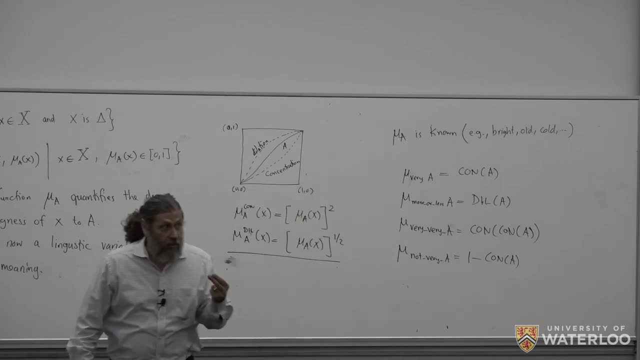 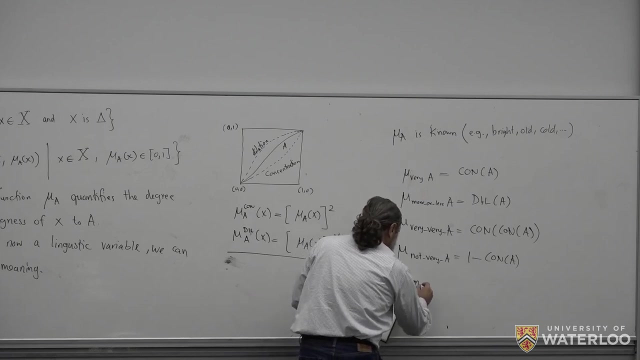 very old, not very old From logical perspective. that was a revolution in the 60s, that suddenly you can do this. What about the mu of more A, More A, for example? you want to say older, Not the set of old man, the set of older man. 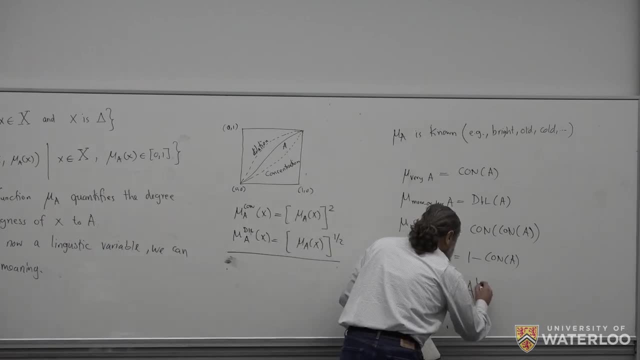 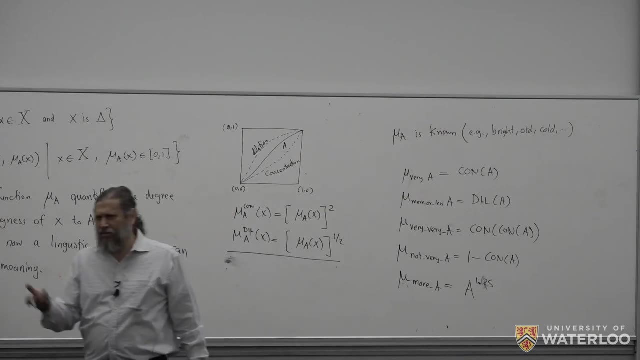 So well, you could take A and raise it to the power 1.25.. Where do you get that number? I don't know. I didn't go out at weekends and sat down and played with numbers. This is one of the major critics to fuzzy logic. 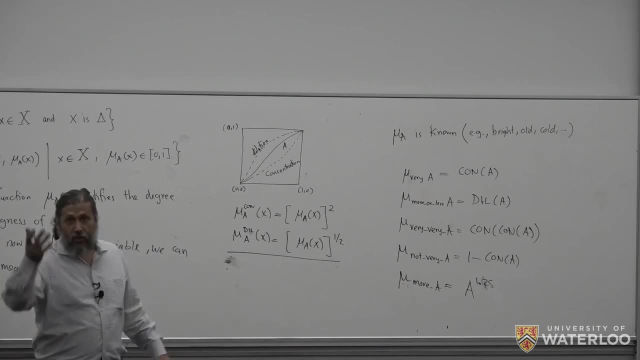 Where do you get those numbers? Where do you get your numbers? Okay, What is the mu of less? A. Well, I can go to the other direction. A raised to the power 0.75.. Whatever the membership is, So we can play with this. 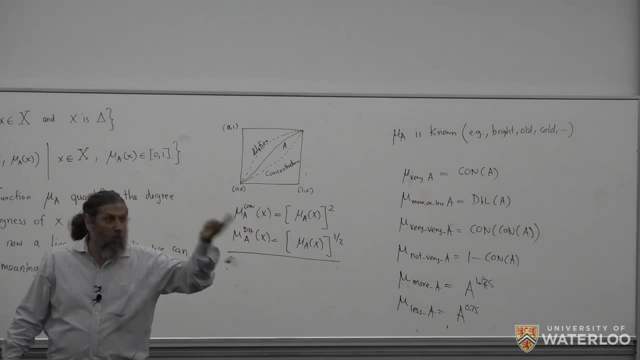 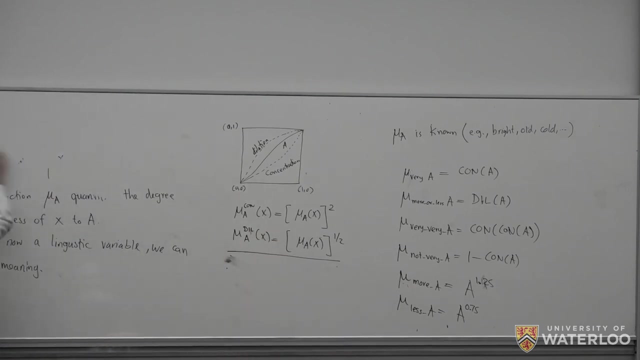 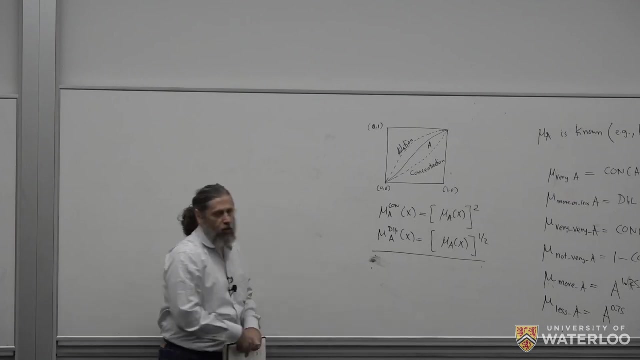 Which, at the moment, I have no idea where are you going with this? So what? So what? Well, Most likely we can do something useful, but then I have to go back to. I have to go back to Aristotle again. 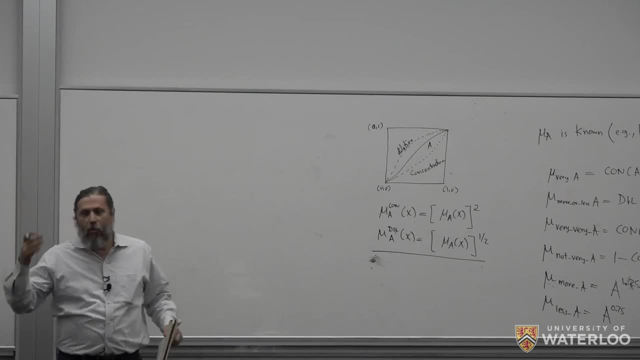 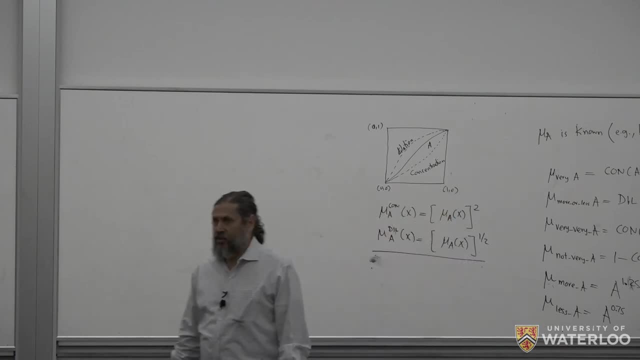 Where is it coming from? Just kidding, Let's go back to the Duncan experiments. It makes sense. So, because I know it has to be more or it has to be less, I can come up with 1.15.. Still okay. 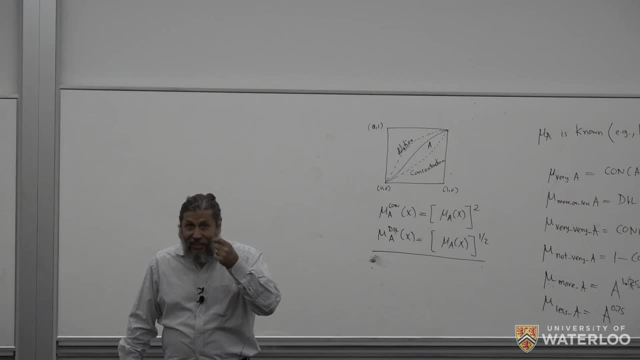 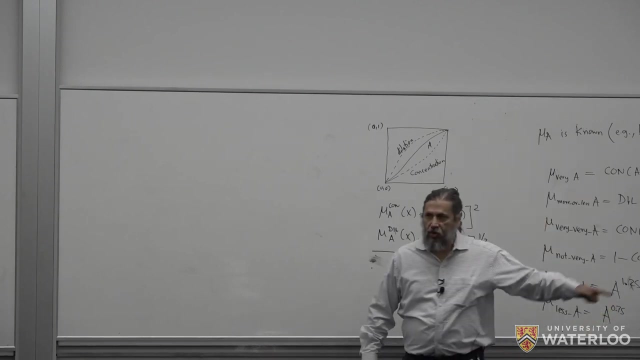 It's one of the critics to fuzzy logic that there is no deterministic way of getting those things established. So there's a lot of them. Yes, there is a lot of them. Yes, You mean mu A of X. Yes, I mean mu of A. So what? 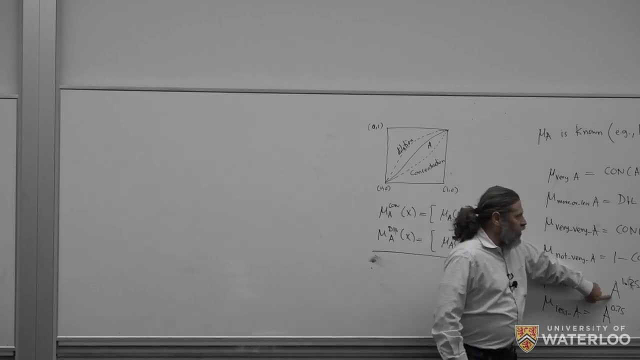 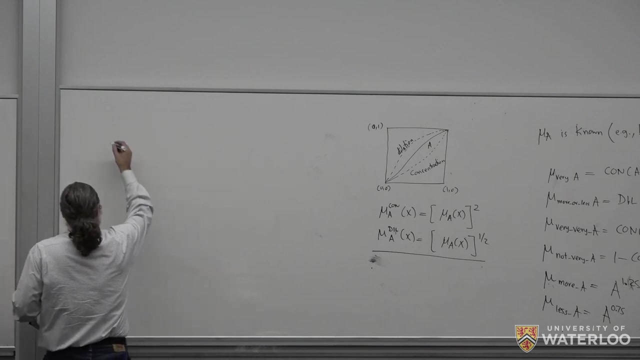 why I wrote it that way? because some people do that, So I should actually write mu of a, but I just did it that way Because a fuzzy subset is represented through its membership function. So, going back to the roots, modus ponens. 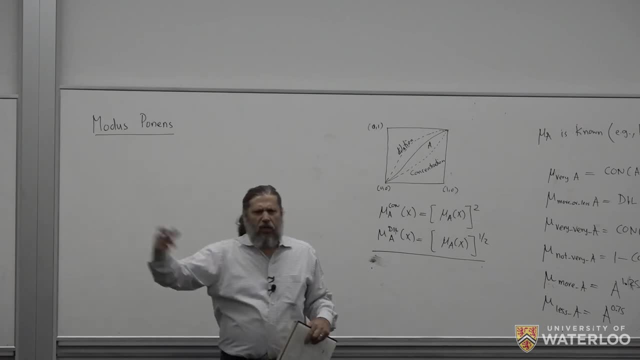 Now we want to get serious. For almost 2,000 years we didn't have anything but modus ponens. There was no AI, there was no SVM, there was no deep, there was no shallow. It was just modus ponens. 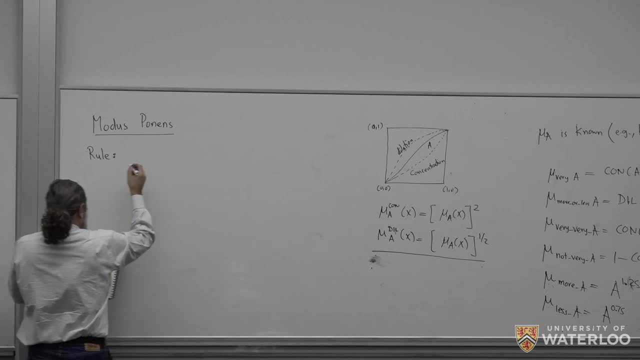 So you have a rule And you say: if A is true, then B is true. Where does the rule come from? Well, many centuries painful life. whales swim from Hawaii islands to Alaska, 5,000 kilometers, not eating anything over three to four months. 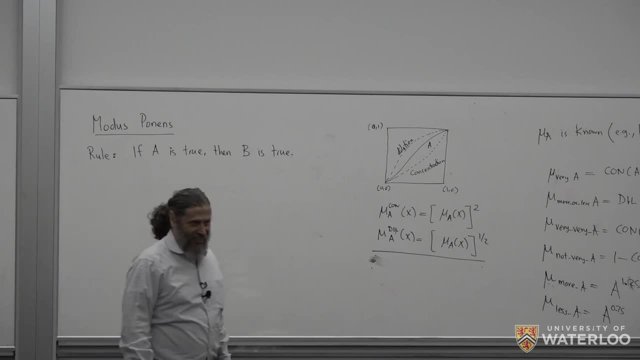 to get there in May because they know there will be food. How do they know If there is a spring there is food in Alaska? OK, They figured it out over millions of years. There are some rooms And they get there barely surviving. 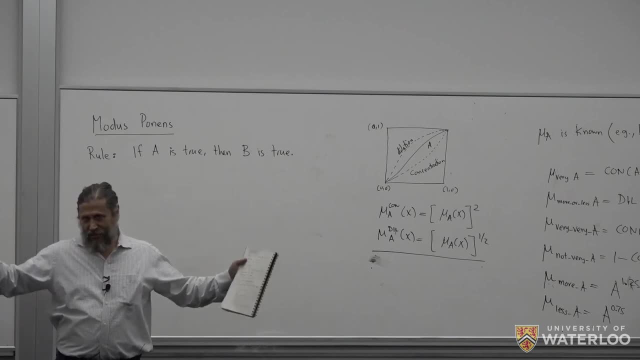 And then there is abundant of herrings. Oh my god, they are delicious. Two months they eat and eat and eat and they head back 5,000 kilometers toward Hawaii. We have a good life Observation, So you have a rule. 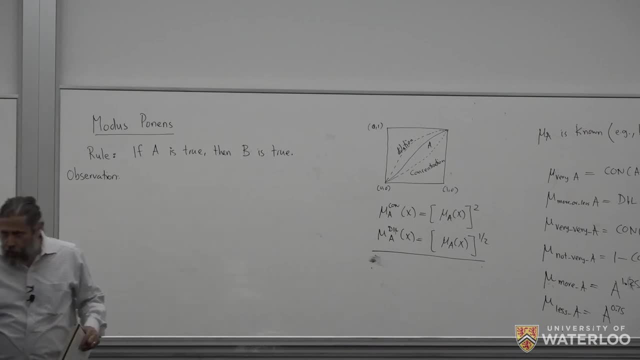 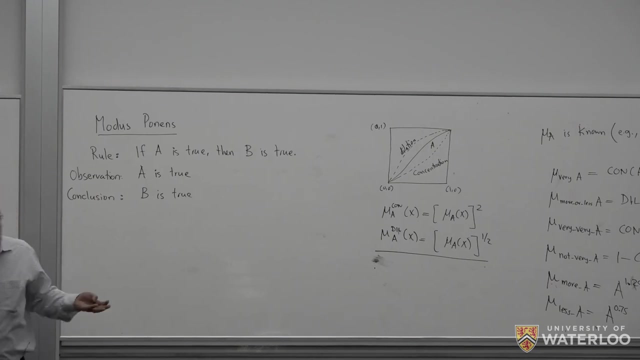 Because of life experience, you have a rule And then today you make an observation and you see that A is true And then you do a conclusion. You say B is true. Our philosophy, basically for 2,000 years, was based on this. 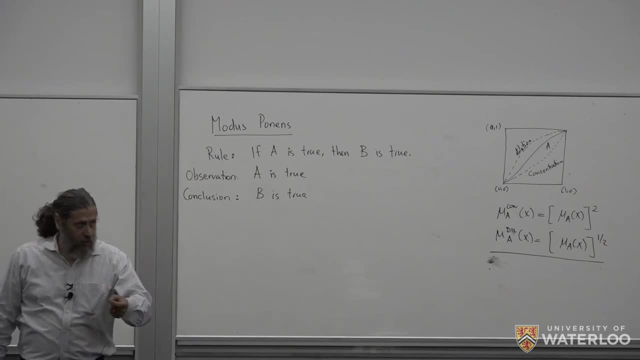 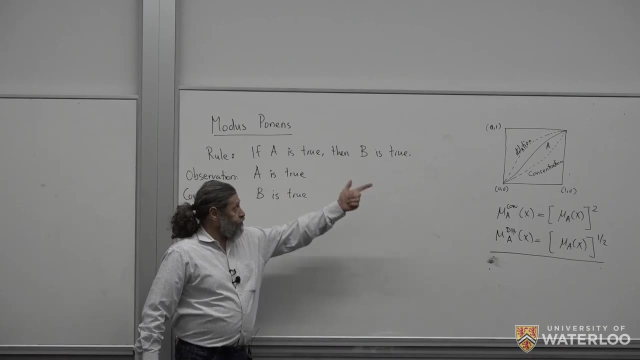 Modus ponens. You have a rule. You make observation. Based on the observation that has to be compatible with the reality. you make an observation And, based on the rule that you are using, you reach a conclusion. If students study, they will be successful. 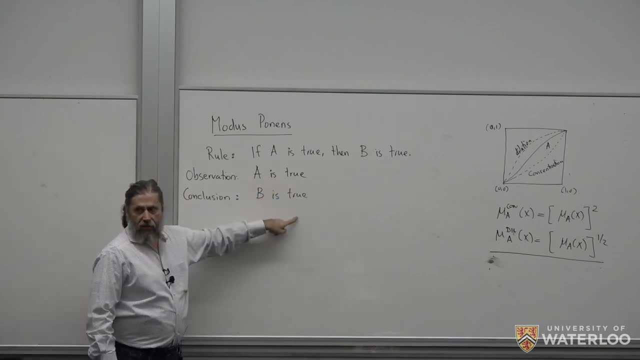 Students are studying, Students will be successful. OK, OK. OK, OK, Sounds cheesy, But this is one of the rules. Is that a rule, Or is it something we have invented? I don't know. So there is also another one, which 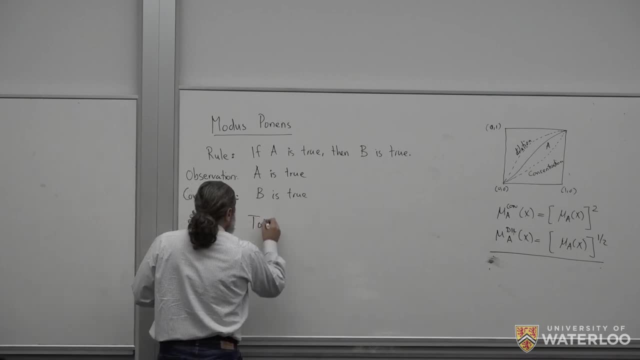 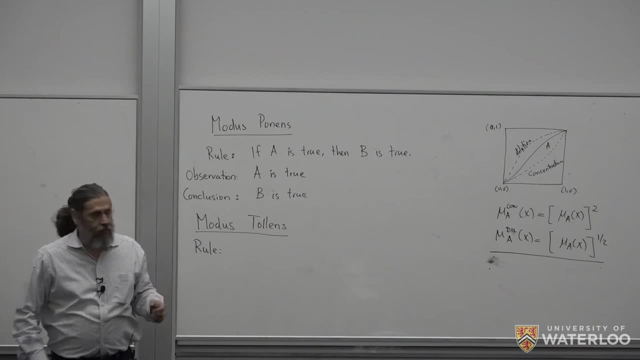 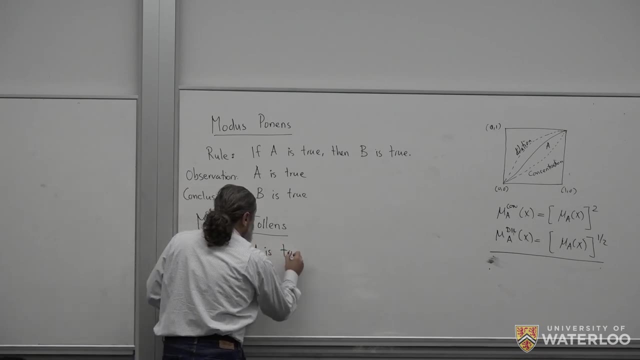 You have many rules. You have many rules. So rule: If A is true, then B is true. Some people want to make us believe that you don't need this anymore because we have deep networks. I love deep networks, but we still need this. 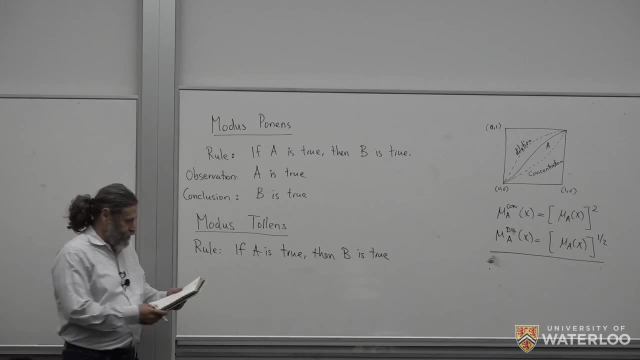 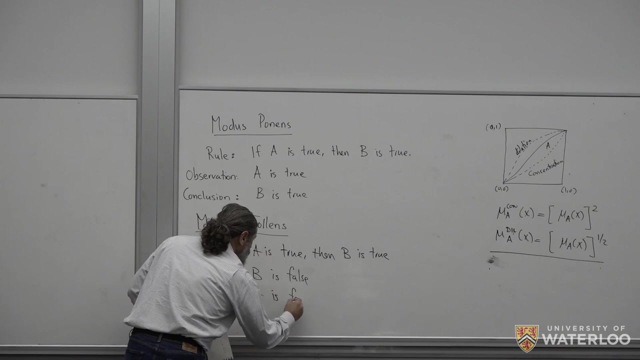 If you want to do comprehensive AI, you still need this. OK, OK, OK OK. Then you observe B is false And then conclusion is: A is false. Rule is: if students study, they will be successful. Students are not successful. 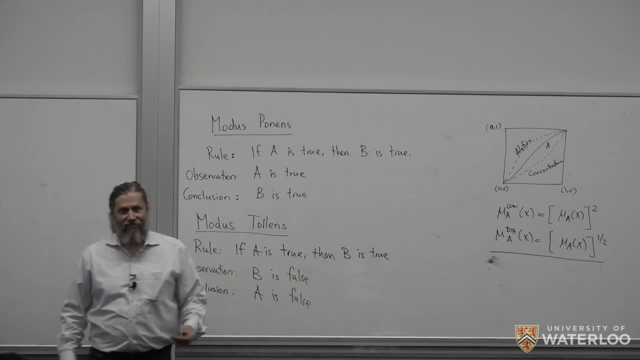 example, Students did not study. Sounds simplistic, isn't it? So? one of the things is this: You can say: if A is true, then B is true. That doesn't mean that you know. This is the only thing that you know. You don't know If you use Boolean logic, you don't know What happens. 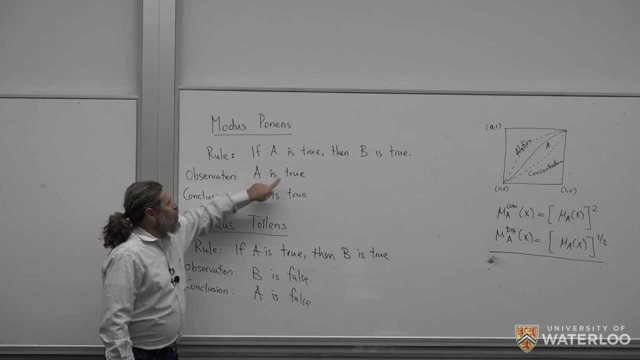 if I the observation is not A is true, The observation is very A is true. So you have the observation: if somebody is old, then Alzheimer's is very likely. But then I make an observation: somebody is very old. I cannot make any conclusion. Don't think about yourself. You can make conclusion. 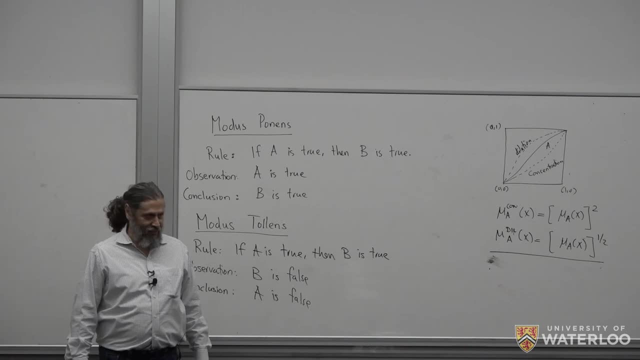 I can make conclusion. Computer cannot make any conclusion. Because my rule is for old people, not for very old people, Because everything is a matter of yes and no. There is no gradient. OK, I thought AI is about function approximation, Wasn't. 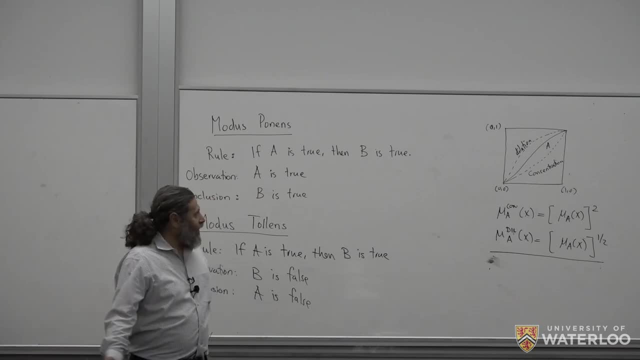 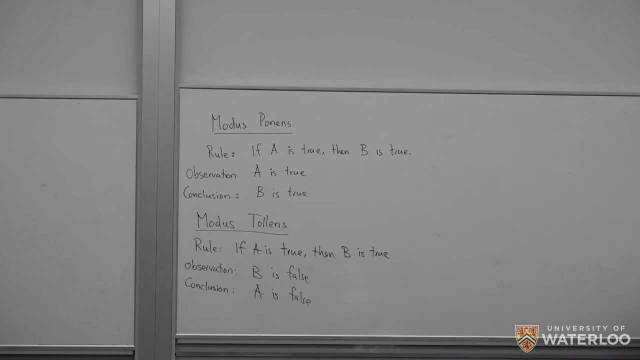 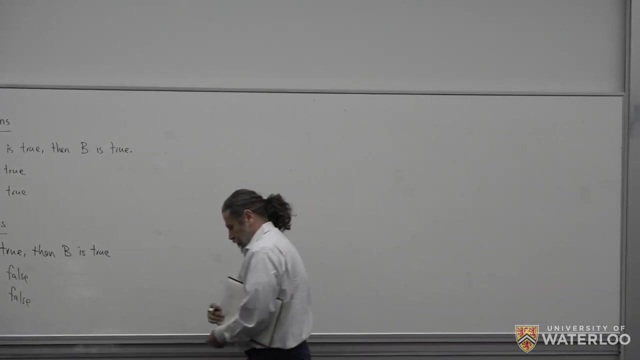 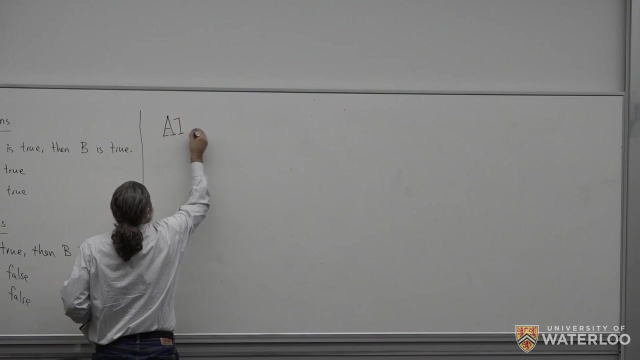 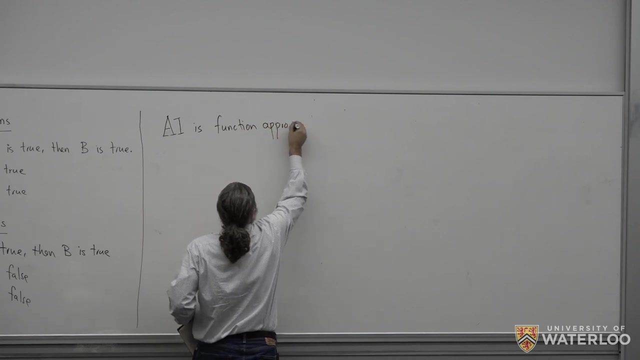 it. We said that many times: AI is function approximation. Yes, sure, Yeah, everything is function approximation. OK, logic is function approximation, So AI is function approximation. Now we can use decision trees, DTs, for function approximation. 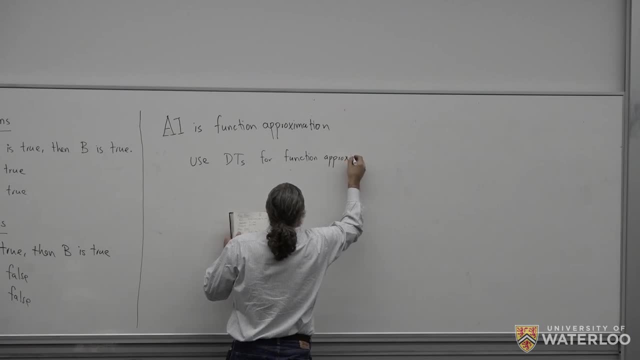 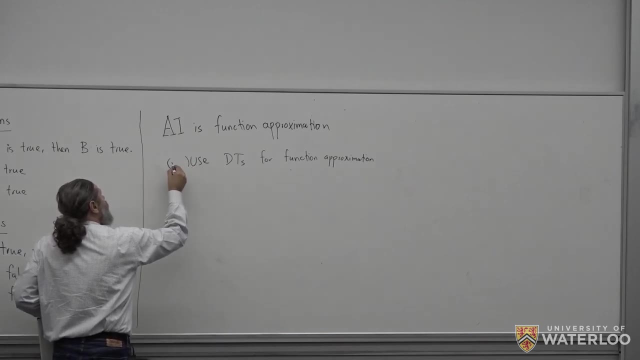 So we can use- some people may say misuse- decision trees for function approximation because they are not really known for that type of functionality. Yes, Sorry, That rule. is it both false? Is it both true? And then should be in the. 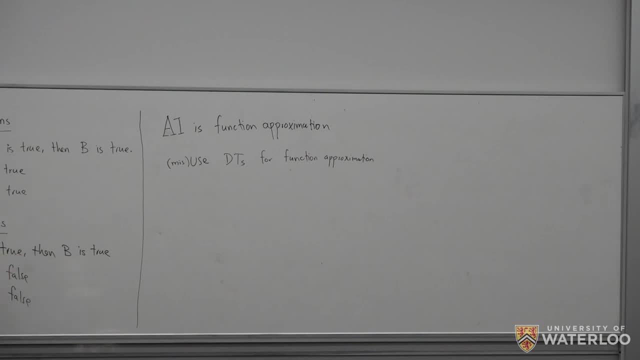 So no, This is the same rule. If A is true, then B is true, Then you observe that B is not true, Then you have to conclude that A was not true. So the premise was wrong. We don't usually use modus tollens a lot. 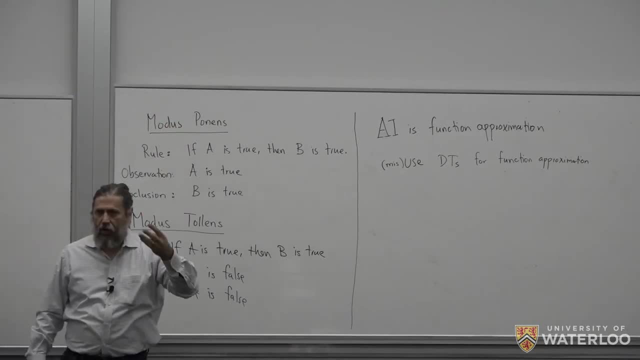 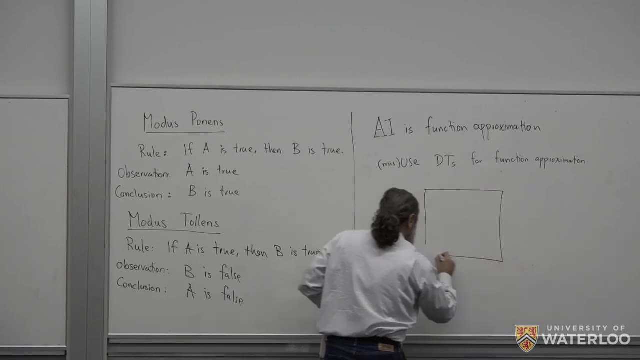 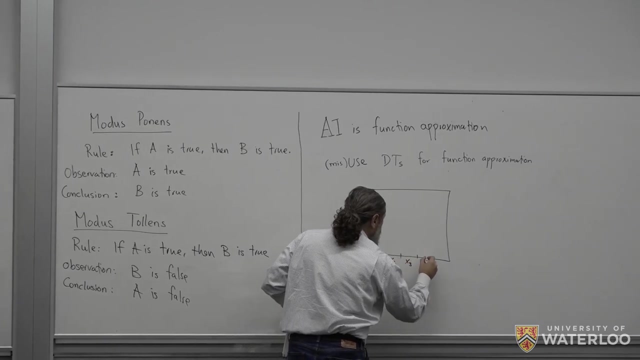 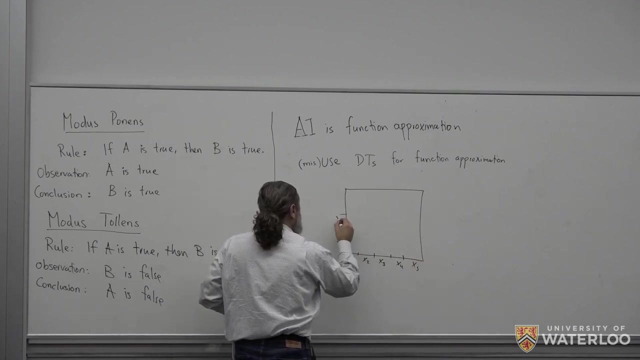 Most of the time we work with modus ponens, which is more aligned with our logic. So, if you have a space X1, X2, X3, X4, X5. And I have Y1, Y2, Y3, Y4, Y5. 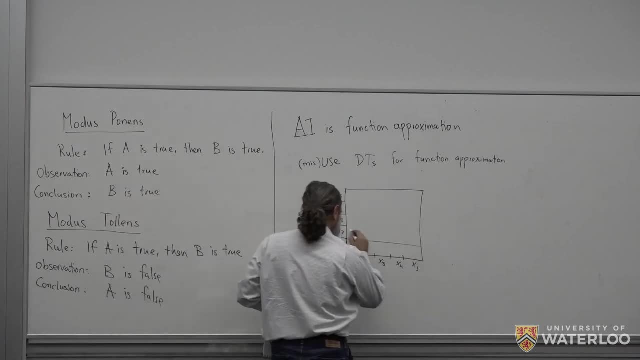 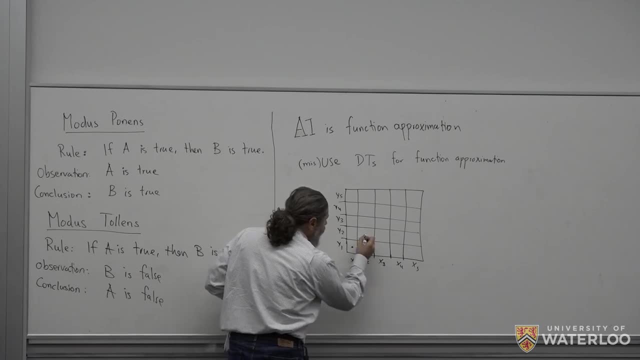 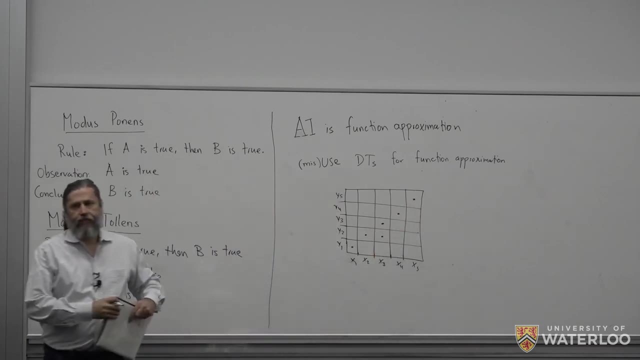 you basically find a point inside one of this squares, Because decision trees are discrete. So I said, if X1 is this, Okay, Okay, X2 is this, and X3 is this, and X4 is this, then Y is this, Y is Y1.. Y is Y2.. And so on. 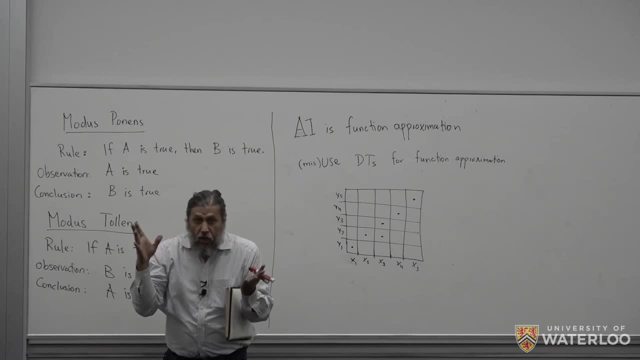 If you could, if you could, if somebody had magical power and would show us the actual function that describes the relationship between in and output, which is all we are after with AI. what is that magical function that describes the relationship between input and output? 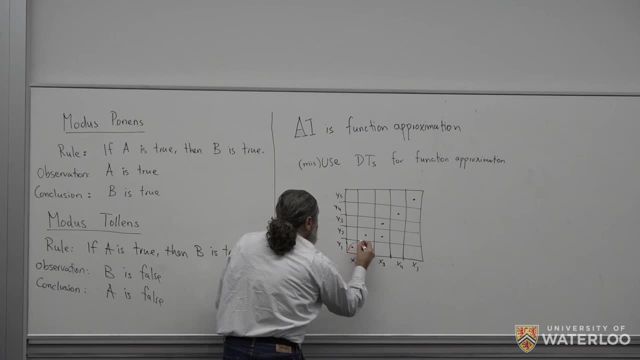 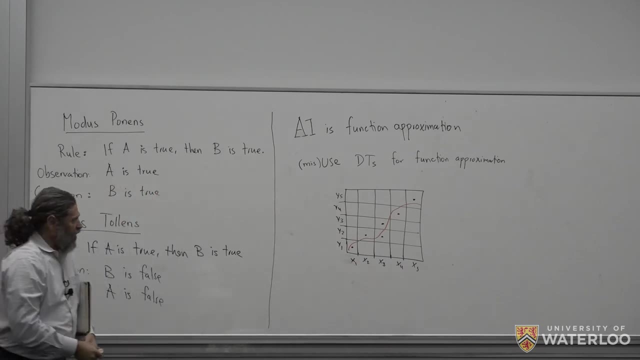 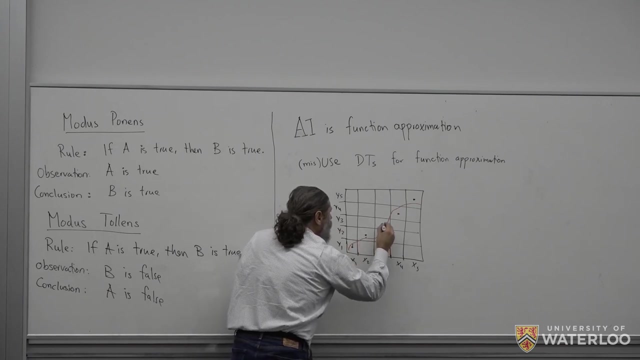 If somebody had that magical function, you would see that you are getting something like this, And if we could get this, you would, of course, see that you have a lot of error in your approximation when you are using decision trees, Because decision trees give you discrete value. 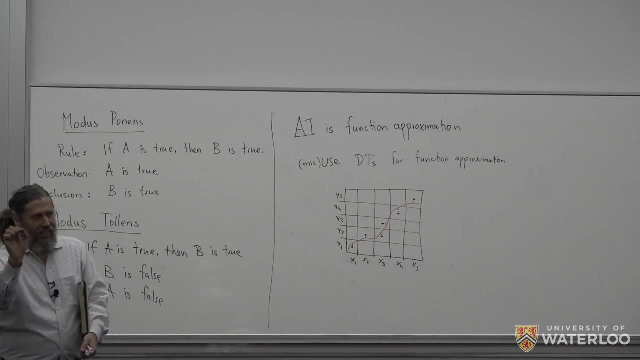 Let's say I simplified. Let's say, in the center of this I have those squares, But the function, the actual function that describes the relationship between temperature, humidity, wind and whether the tennis club is open or not, is a very complicated function. 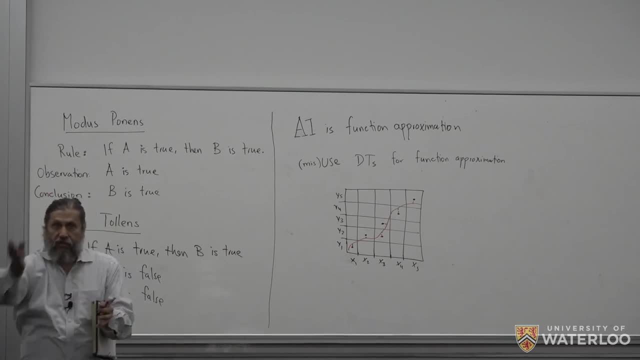 It's a nonlinear function. It's a function with a lot of curves, So if I use decision trees for the function approximation, it would not be a good approximation. It's a very complicated function. It's a very complicated function. Why not? 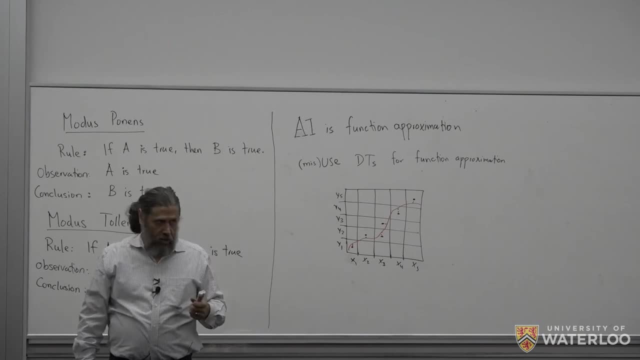 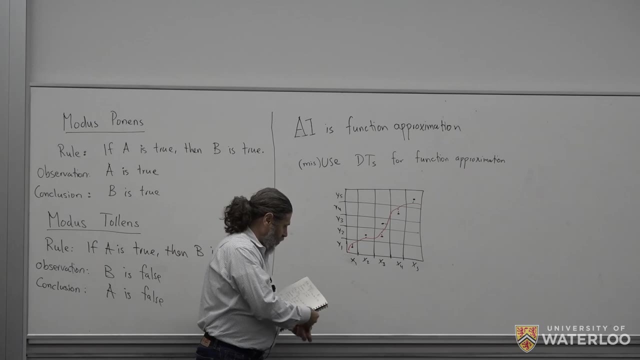 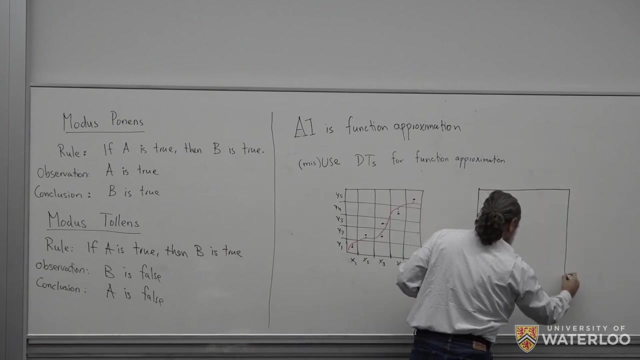 Because they are discrete. Phasologic is not discrete. It gives you value between 0 and 1.. So the expectation is that this is going to be much more accurate. So if I draw the same thing, if I give the same problem to phasologic, then I get something. 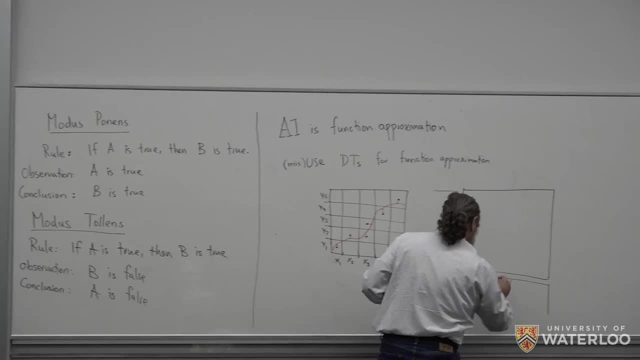 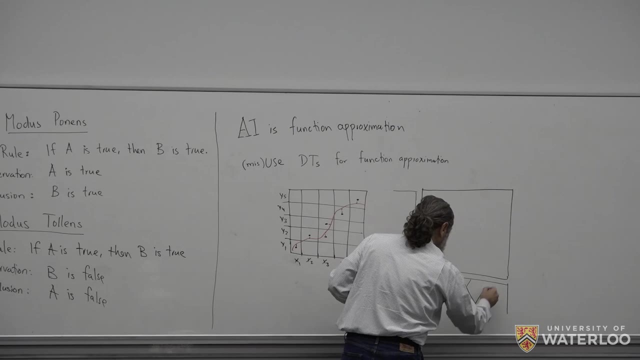 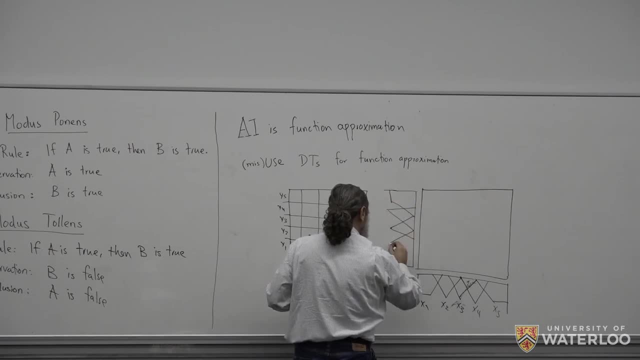 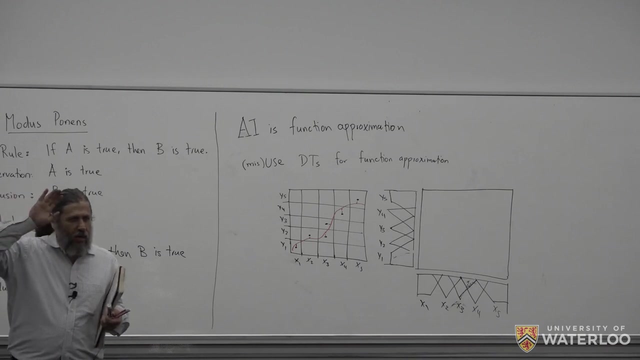 And here I have y1, y2, y3, y4, y5.. So now I'm not discrete valued, I have functions that move between 0 and 1.. So now I want to come up with a. it could be understood this way, not that it is only. 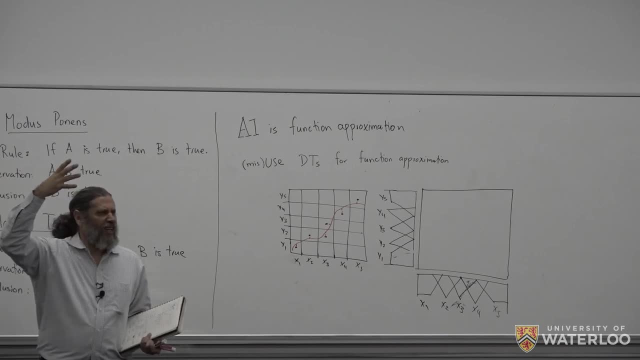 this way I want to come up with a version of decision. So I want to come up with a version of decision trees that can work with numbers between 0 and 1. Not just discrete values, yes or no? Is it either a square or is it a circle? 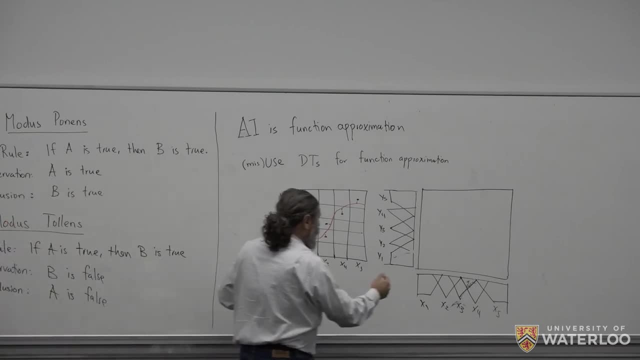 I don't care what else it is. Now, if I draw roughly, don't take this too seriously because I'm not trying to really be accurate here. So if I draw the same function, If I draw it, I try to somehow draw it to same function here. if I approximate this with fuzzy logic. 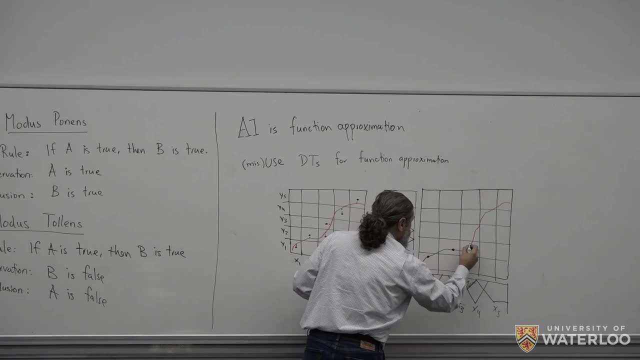 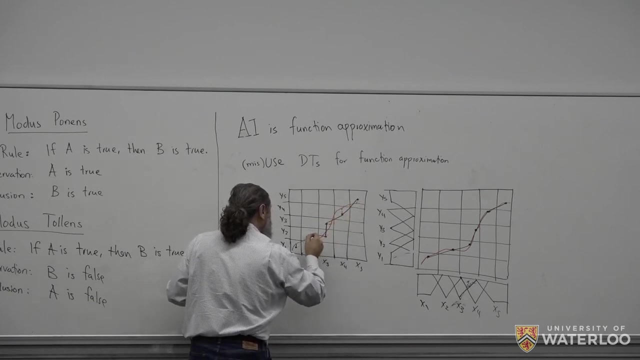 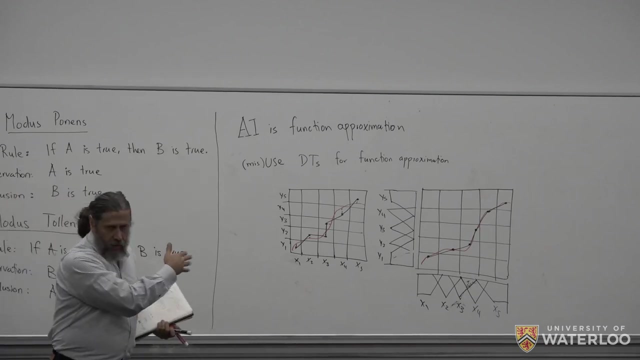 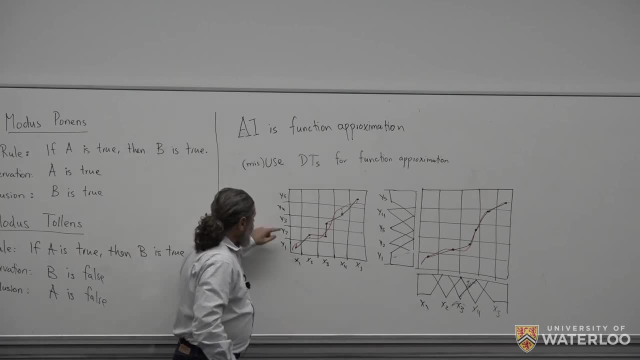 I'm just making at the global level, making the point that if I go from scalars to functions, I gain more information. Of course you do. If you go from one number to a function, of course you do. Yes, we do. but how are you going to process functions? 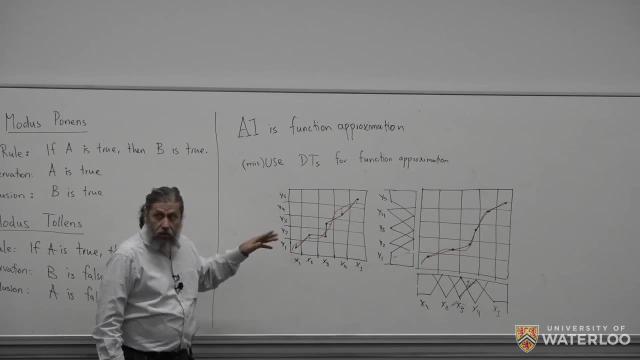 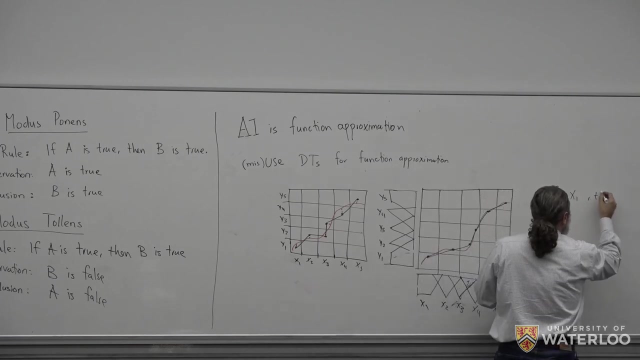 Because every function that we have is operating on scalars, so it's not that easy. That's the magic of fuzzy logic. So, which means here? so you are processing rules, you know, like this: If X1.. Okay, If X1 than Y1, right. 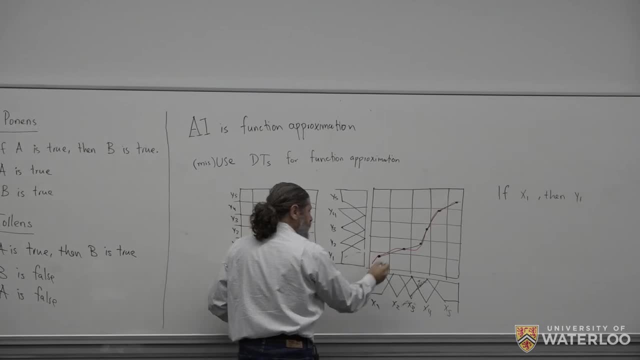 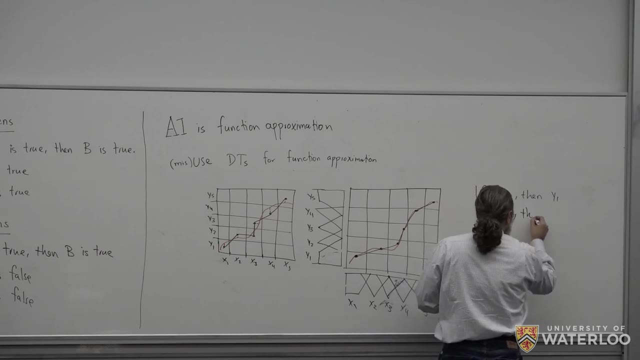 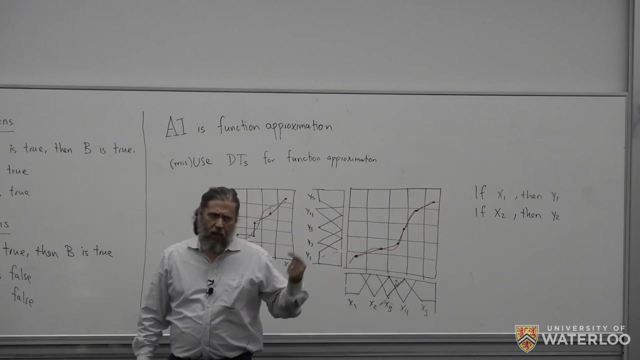 So if X1 than Y1, you process it. you get a point. If X2 than Y2.. If X2 than Y2, so you get a point here. Hopefully we can go through an example to see how that works. 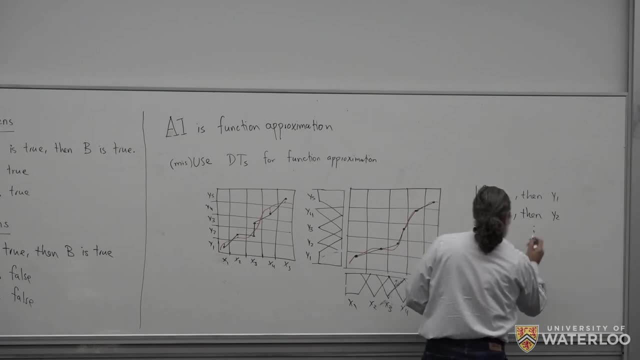 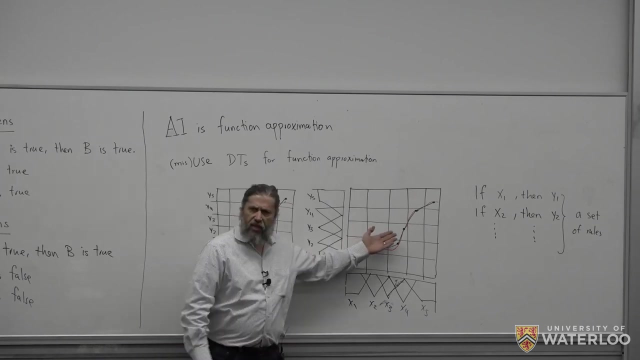 So and so on, And so on. So I need a set of rules, A set of rules Which is- nobody sees. this actually, All you see, somebody gives you a set of rules. Or, even worse, nobody gives you rules. 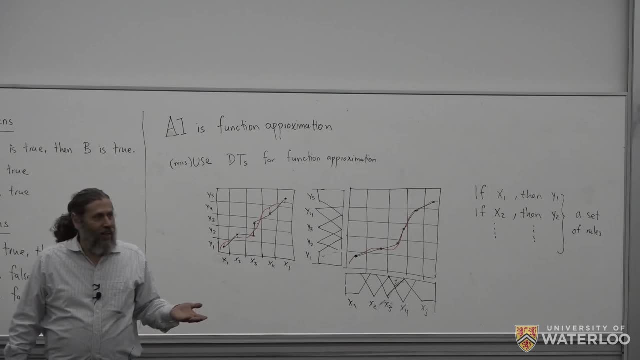 You still get that Excel file with some numbers in it. Okay, How can I, How can I extract rules, some numbers? Well, easy, K-means, Apply K-means, Get the clusters Construct, function around them. Voila, You have your rules. It's very simple, It's not really difficult. So what? 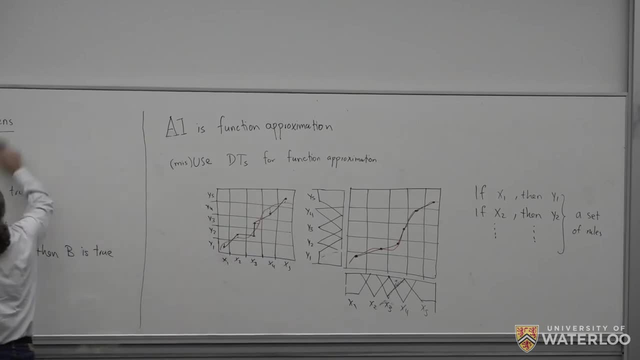 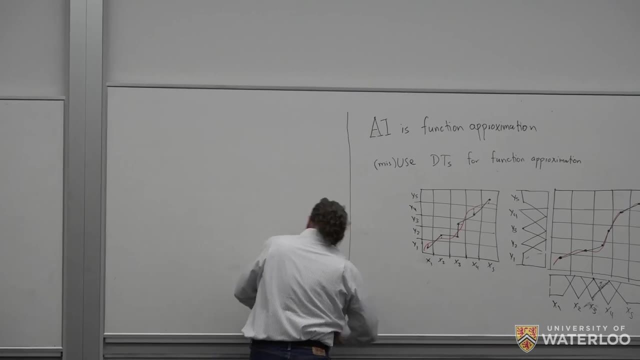 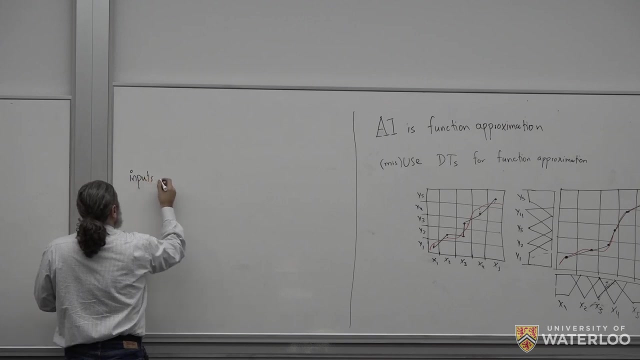 does that mean? How can we use this in a systematic way? This is very high level. So your inputs come in, whatever the inputs are, Then you get the first block. In this first block you do some sort of coding. This coding is usually happen. 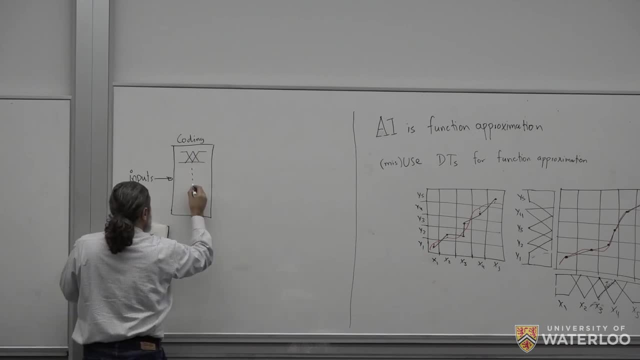 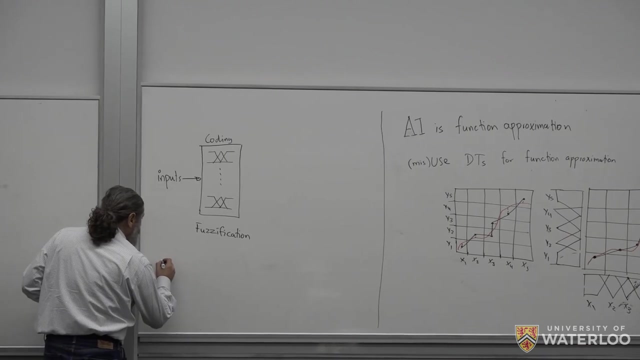 in fuzzy systems with some sort of membership functions. So the input comes in and you put them through some membership functions. This step is called fuzzification, So you fuzzify your input. The example was that we said: what was it? Cold temperature? No, It. 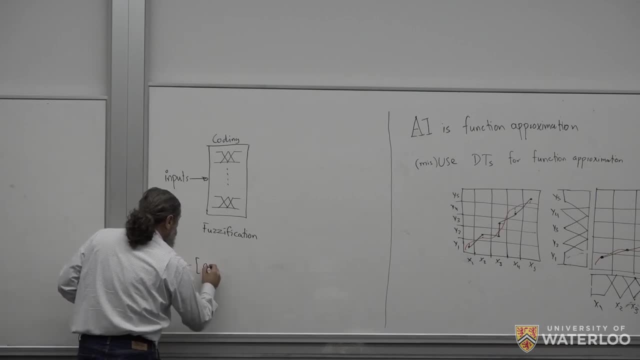 was minus 22 degrees was 0.75.. Let's make him happy: 0.25, 0, 0, 0. That's the encoding. So minus 22 degrees become encoded as a vector, In this case five numbers, because I chose five. 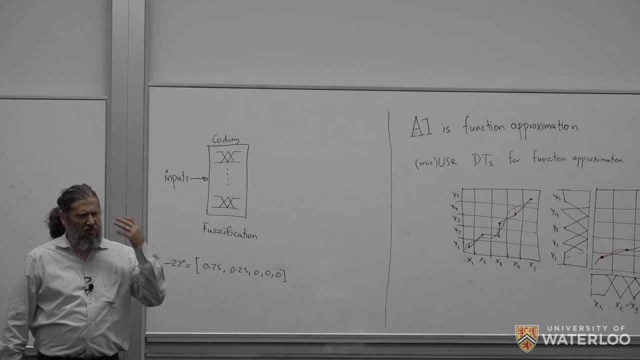 membership functions. Why did you choose five membership? I don't know. I felt like it. I can do 7,, 9,, 11.. So that's the encoding part, which means you don't deal with minus 22 anymore. Minus. 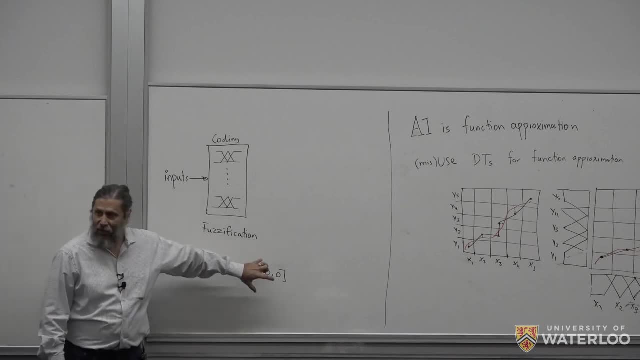 22 degrees is for you now this vector which shows how nasty things can get for fuzzy systems because you have to process a lot more information. The first 20 years we couldn't actually do any fuzzy inferencing because there were no hardware for that. 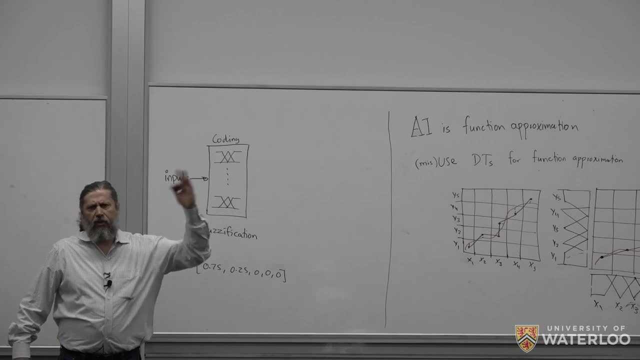 And you couldn't run it on a regular PC until there were some Japanese companies. They came up with hardware and then suddenly you could buy a car that could process 10,000 rules per second. Nowadays it's not a problem, You can do millions of rules in a second. 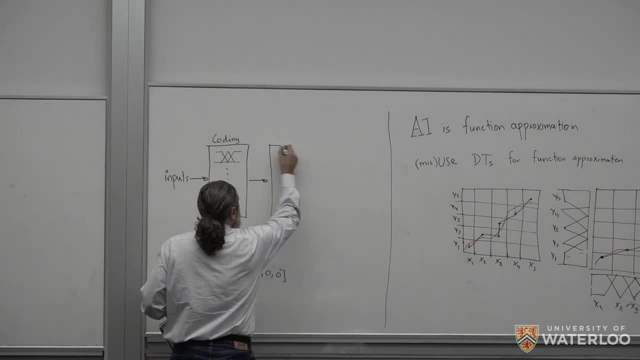 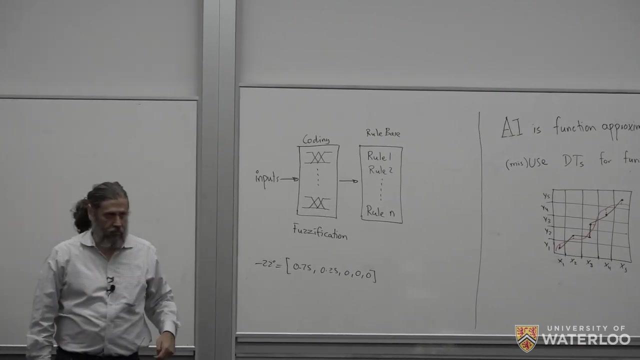 So after you code stuff, you go somewhere that you have a rule base. So you have to check that out. You have rule number one, rule number two, rule number N: If X1 is this, then Y1 is this. If X1 is this and X2 is this and X3 is this, then Y3 is this. If you 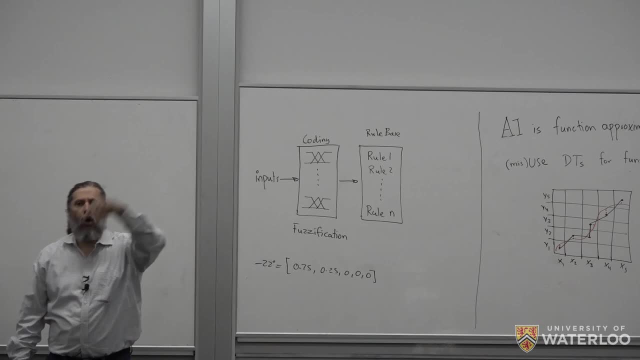 eat unhealthy and you smoke and you are old and there is history in your phone. you need to look at the code and see if it's the same as the code you're using. To evaluate the code that you're using, you need to look at the code that you're using and you need 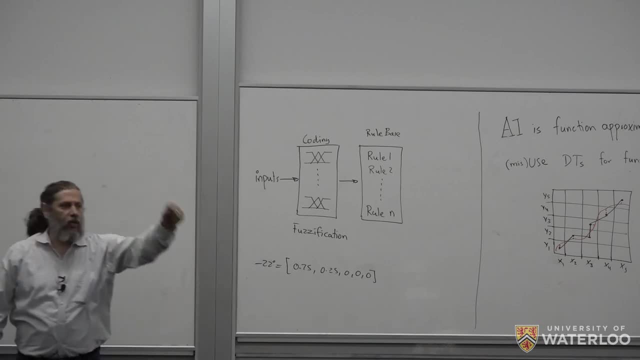 to remember that there are various code мн and code ln that you need to own And you will have to pay attention to that. The code is issued every week. There's normal code and there's family, then you're susceptible to this type of diseases is a rule, so I can put it. 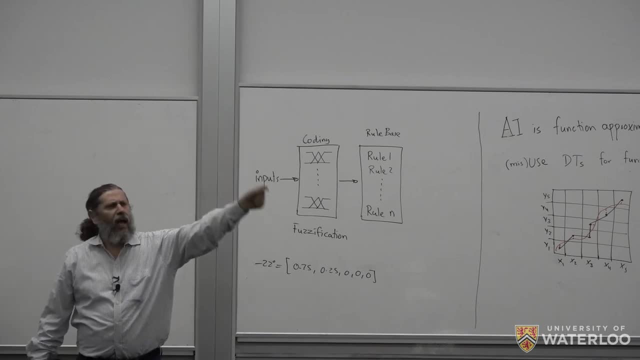 If the government mess up, there is political conflict and the oil price goes down, then the stock market behaves this way. So rules, apparently those rules are not straightforward and apparently they don't take one variable, they take many, many variables. 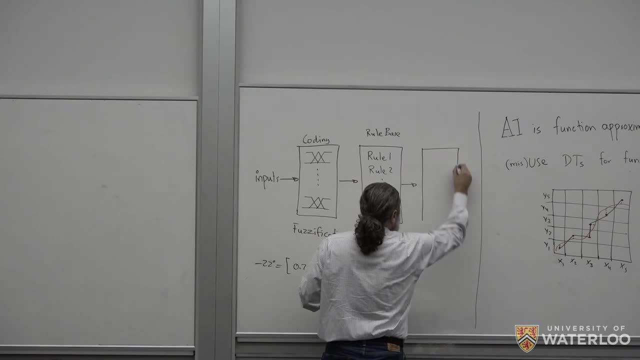 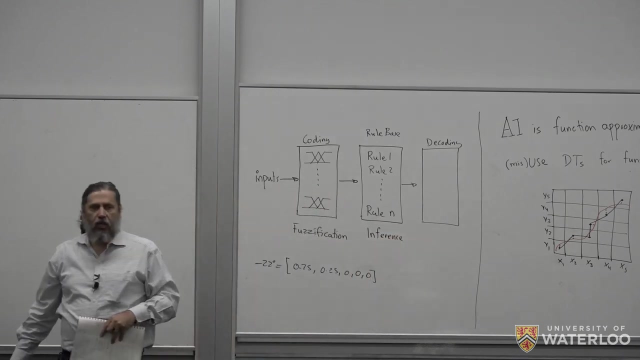 And then the last part is a decoding part. So this part, by the way, we call it inference, which is a magical word that actually was dying when, in 1965, fuzzy logic emerged. And then fuzzy logic basically revived the word inference. 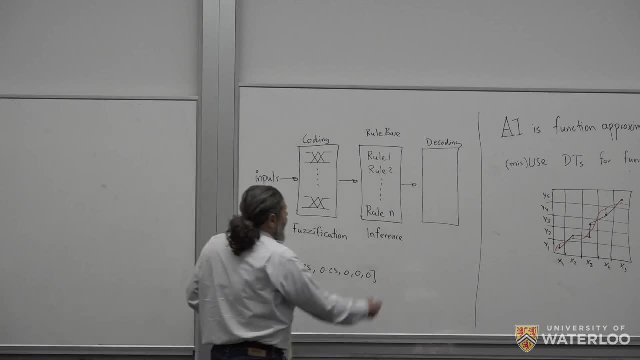 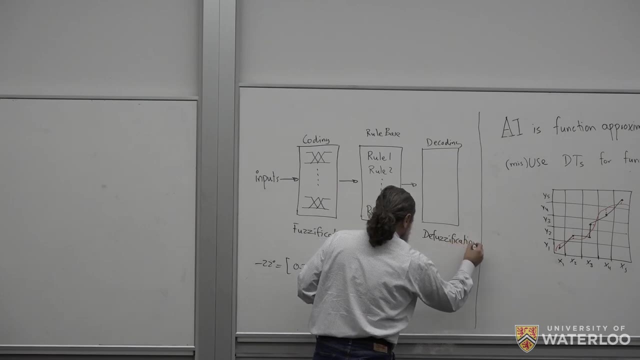 You can infer knowledge And decoding- we call it de-fuzzification- and in the de-fuzzification you have multiple membership functions and in the de-fuzzification, what it does basically gives you a combined value. Okay, 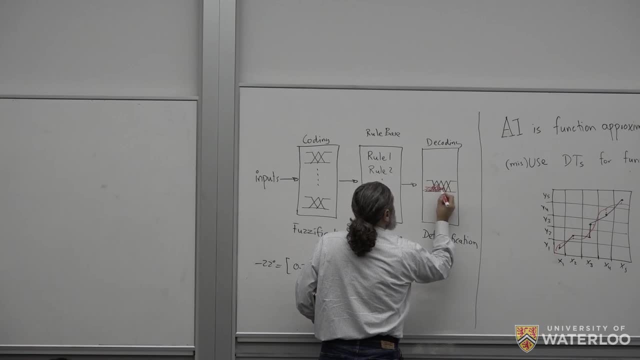 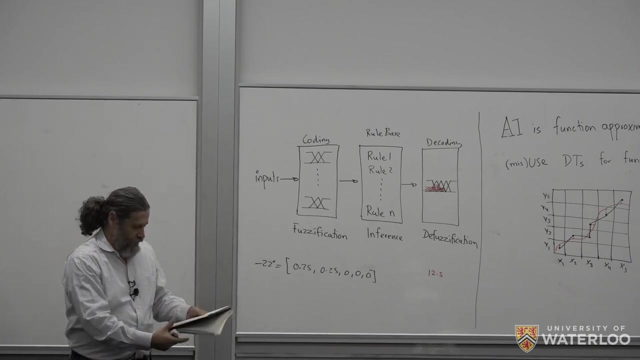 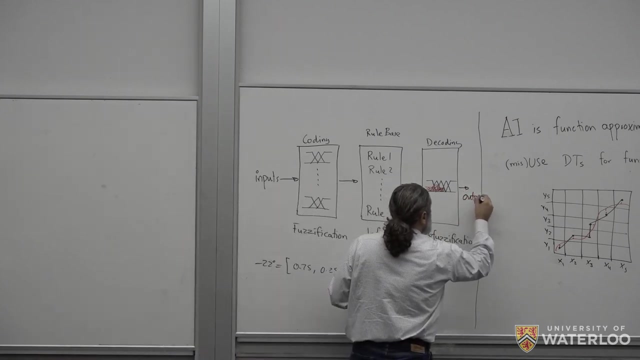 So you have a function of the output function and says this is your answer, and you get some number, whatever, I don't know: 12.5.. You are controlling something, whatever that is. So this would be your output. 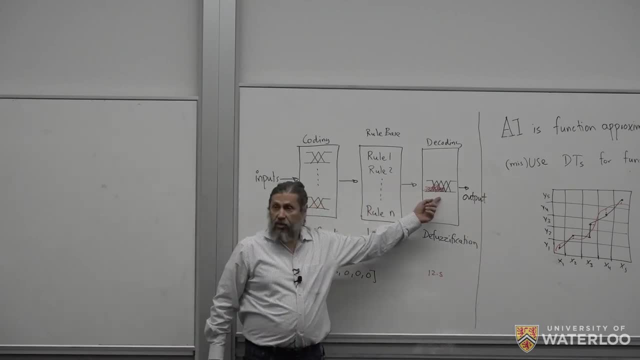 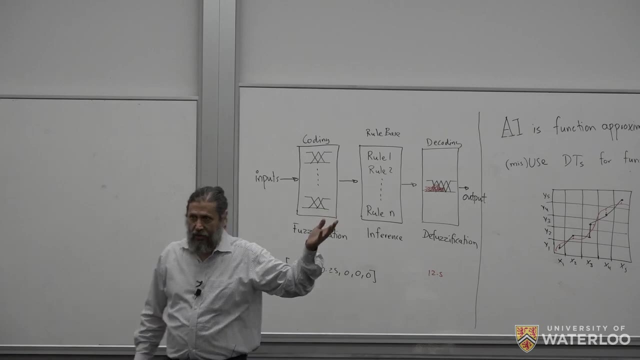 So actually the output of a fuzzy system is a function like this, But since our computers don't understand that, we have to convert it to a number, So we use some tricks to convert the caught surfaces underneath functions into a number. Okay, 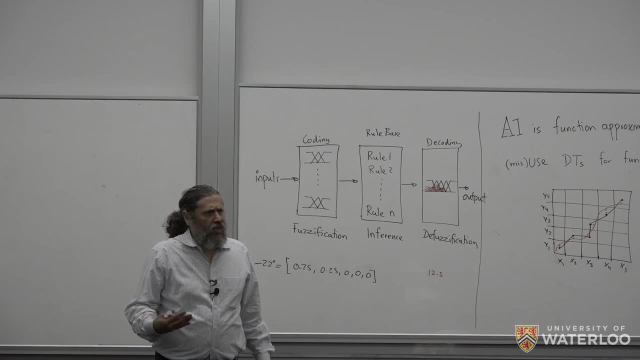 So I want to have an engineering example for this. How does this work? Especially because the most successful application of fuzzy logic was control. Okay, So designing controllers, What do you have learned? The P controller, PID controller. So now I challenge you. 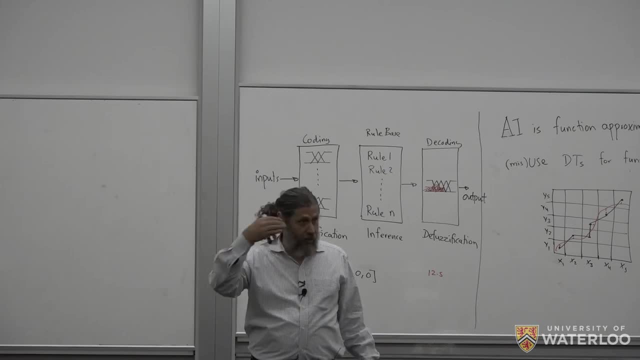 Any problem, pick any problem. this weekend we come, I get a MATLAB or Python compiler, you get a MATLAB or Python compiler, somebody else grabs a problem to control and I give you a perfectly designed controller with fuzzy logic in five minutes. 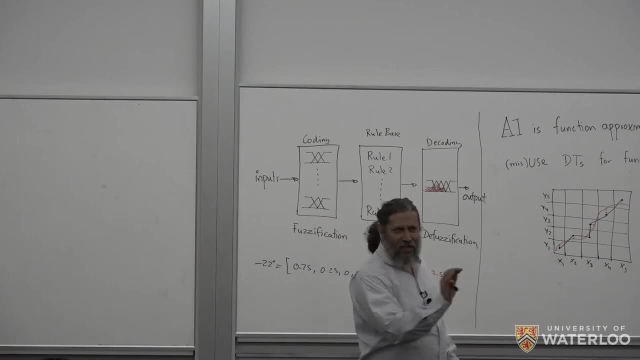 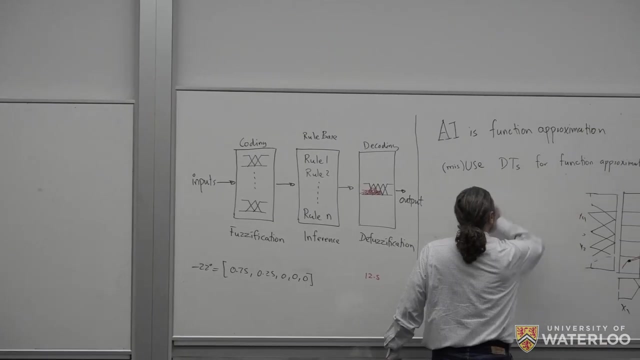 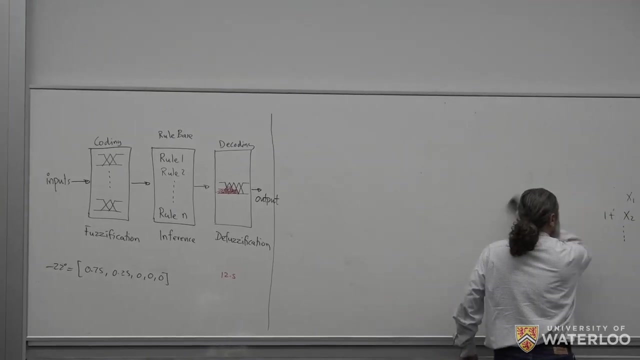 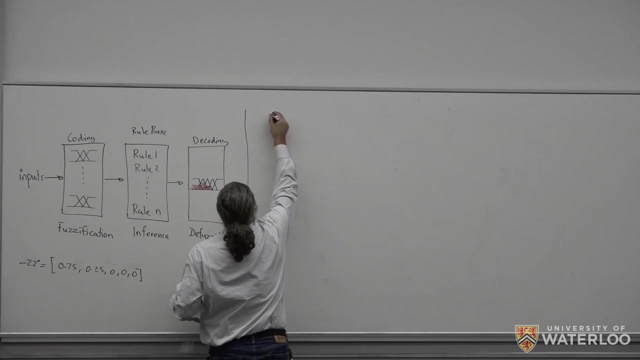 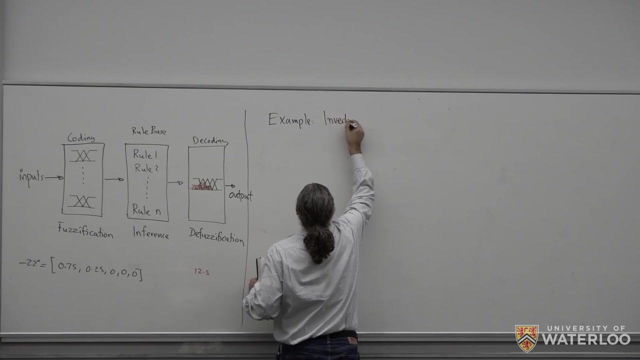 Smooth, Nice, It's amazing. As an engineer, you cannot not love fuzzy inferencing. So how does that work? So example: Okay, Okay, Okay, Okay, Okay Okay. This is the card. So by looking at this, 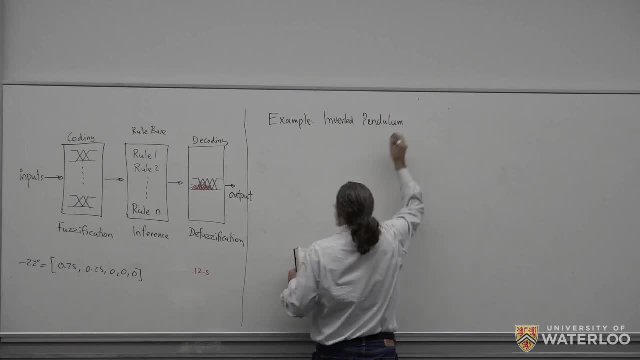 Of course we go back to inverted pendulum. We didn't really do anything with it. reinforcement learning, which is defined the reward function. But we didn't do it because the design of reinforcement learning is a pain in the neck. You cannot in five minutes on the board. 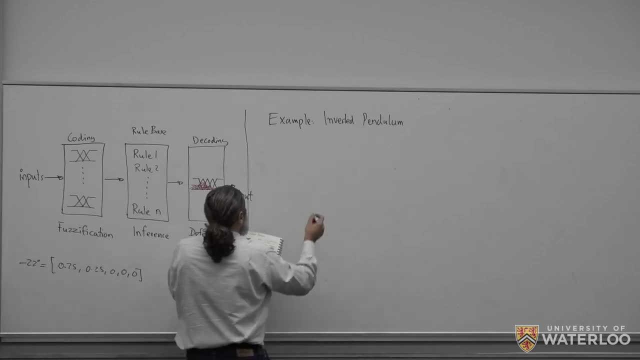 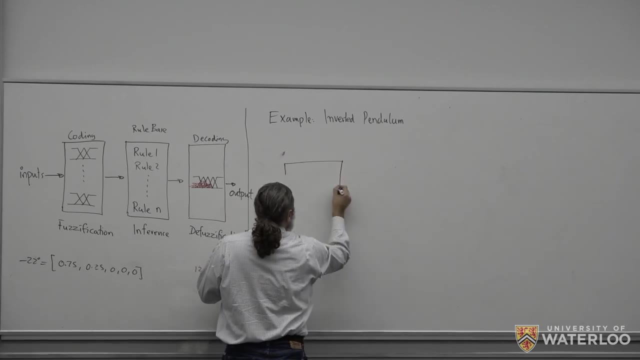 So it takes some time, So we didn't go into it. So again, I have a card, Thank you for attend card. I have a card that can go back and forth and my pendulum is here and the pendulum can go to the left or to the right. Problem analysis: what are the inputs? First, the 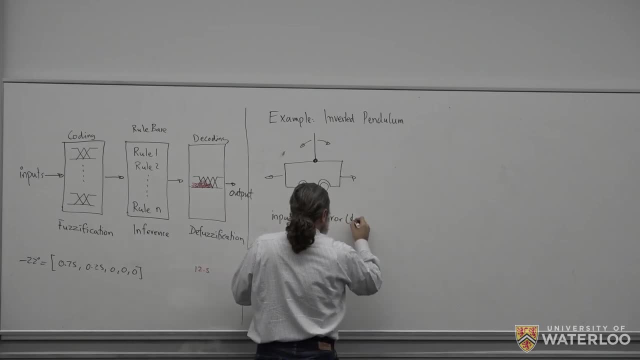 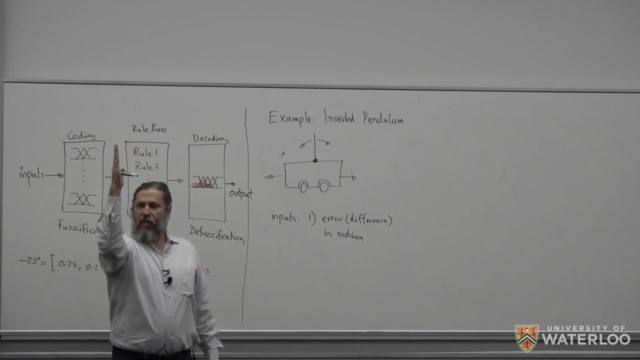 error, which is the difference in radian. Anything that deviates from zero or 90 degrees- if you want to put it at 90 degrees- anything that deviates from zero or 90 degrees is an error. I want to keep it that way. 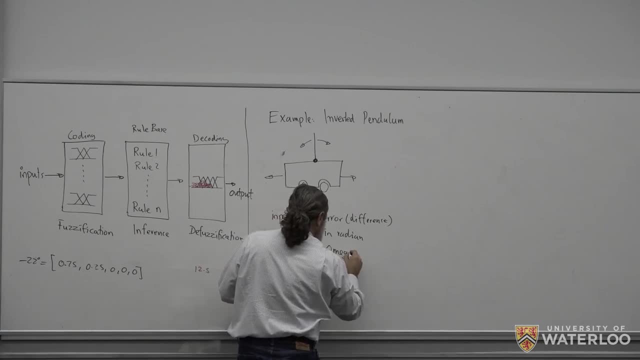 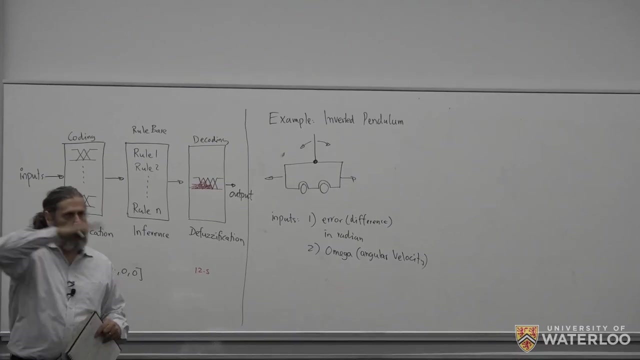 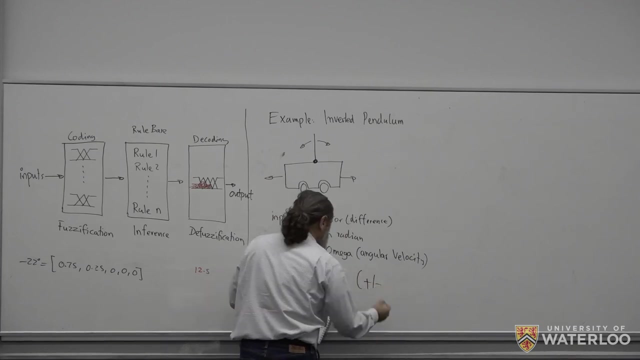 Second, omega. Omega Or angular velocity, Because there is a velocity in that. So the angular velocity, how fast is it falling? Then I need to know output. What is the output? The output will be, let's say current Plus or minus for direction: 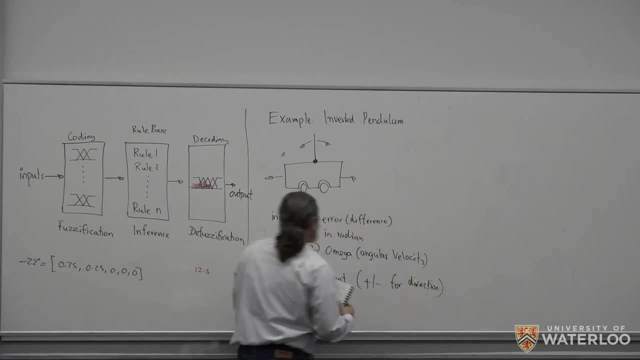 0. 0.. So I want to either put plus and I go to the right, or minus some small amount of AMP plus to go to the left. So I want to control the pendulum: Go left and right, So I know. 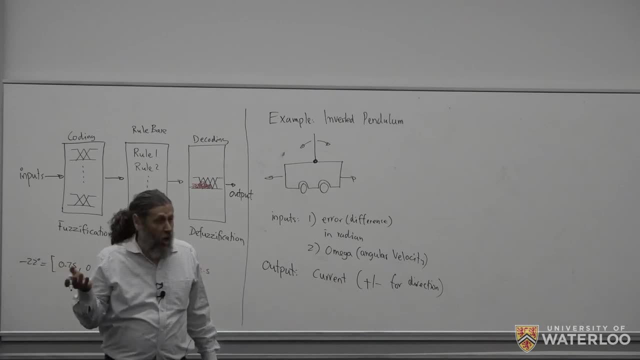 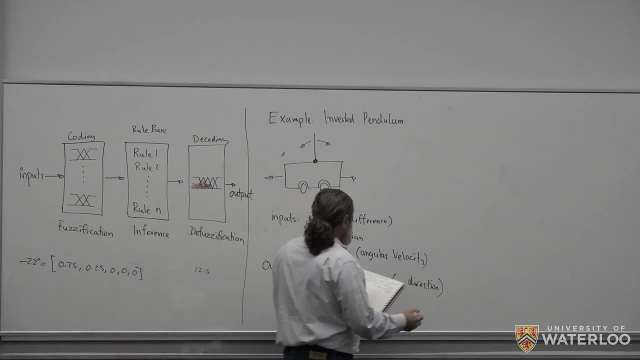 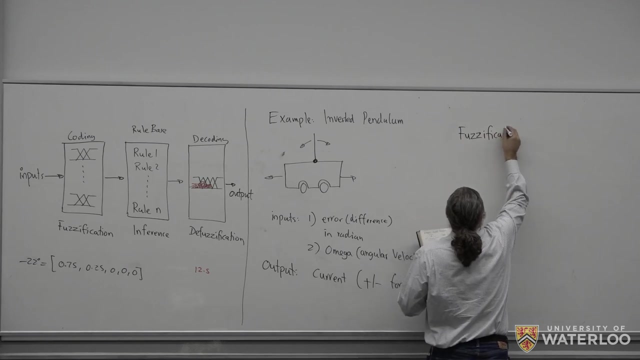 my inputs. I know my outputs, which is the beginning of every AI project. What are your inputs? What is the output? 0. 0. 0. Okay, Then the first step is phasification. So what is the error? The error is something. 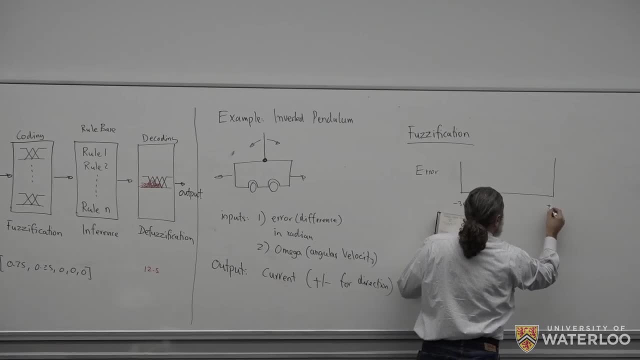 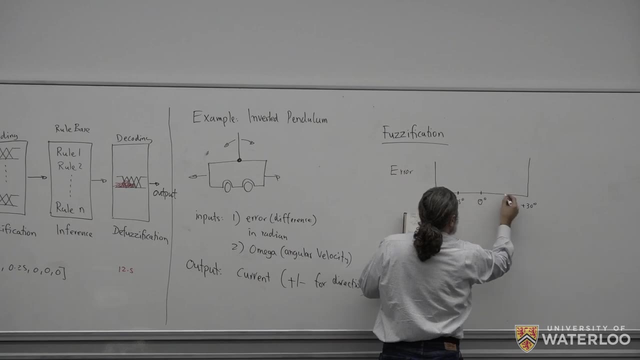 that goes, let's say, from minus 30 degrees to plus 30 degrees and in the middle is zero degrees and here is minus 15 degree, here is plus 15 degrees. So I'm assuming if you go minus 30 degrees or 30 degrees, this is too late anymore, so we cannot save it. It's. 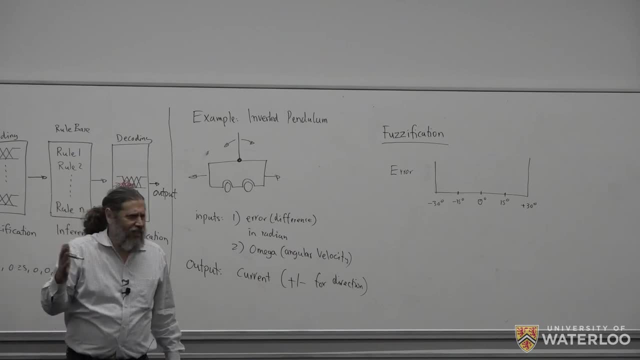 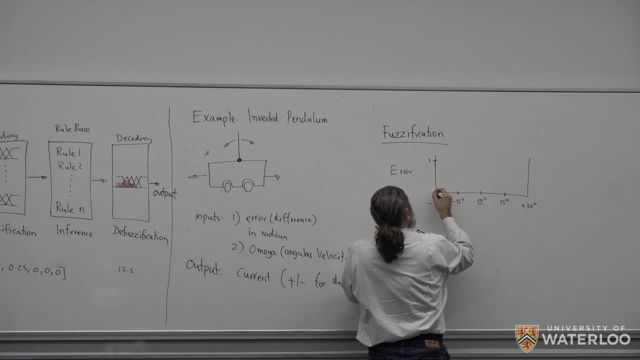 gone, Actually, around 27 degrees is then too late, And this is, of course, one, and this is zero. This would be for us zero, Zero error. Then this would be for us negative, small and 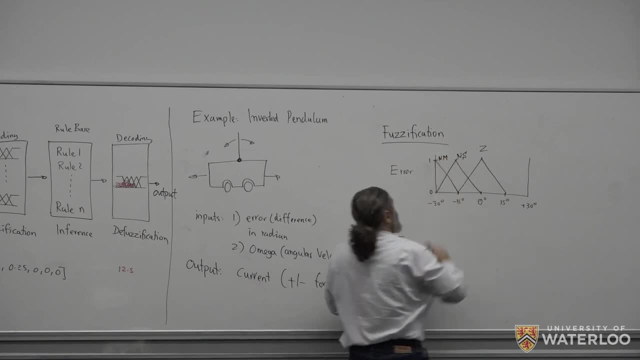 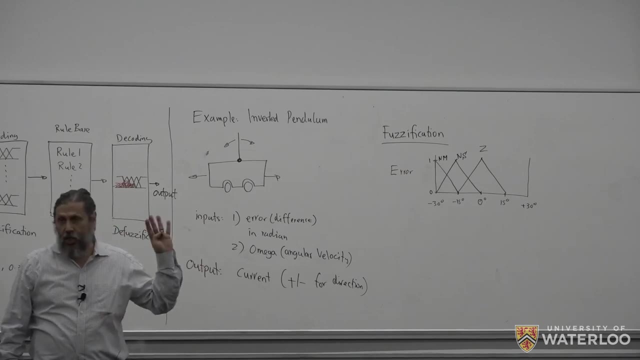 this would be for us, negative medium. I'm intentionally using those acronyms or abbreviations because very common in engineering design of phasicontroller: Z for zero and S for negative small And M for negative medium and B for negative big and so on. On the other side, I go and 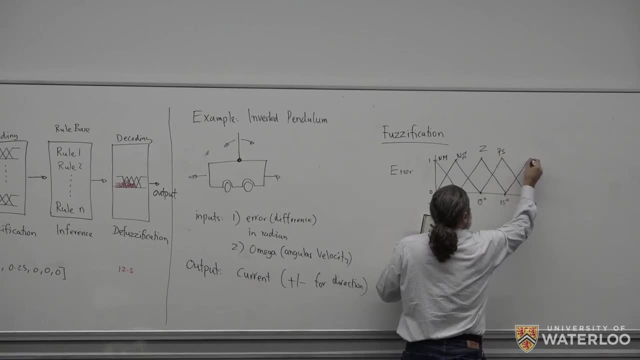 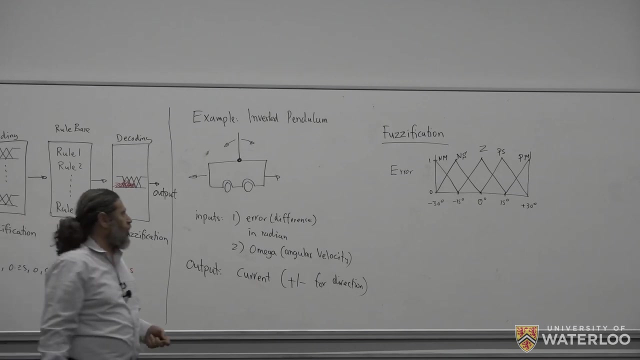 I have positive small and I have positive medium. You're just putting a label on it. So this is the set of terms of the linguistic variable. So I have to put a name on it such that I can work with it. So put any name on it. So zero for me is anything. 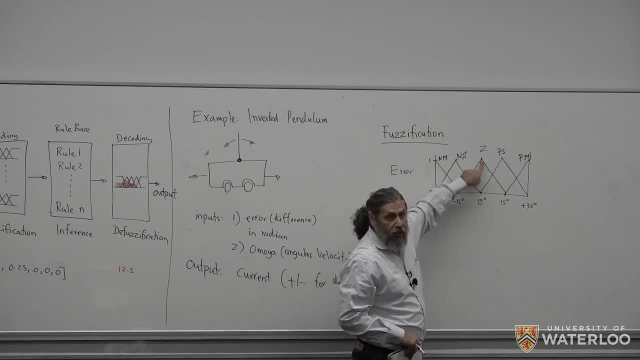 you see, if really is zero, the membership is 1.. If it is minus 1 or plus 1, it's still regard as zero, with a likelihood or membership of 0.999.. So that's the tolerance that we want to have. Then we have the other input, which is angular velocity. Let's say angular. 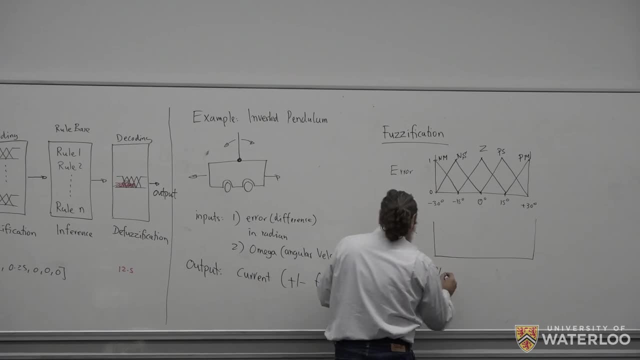 velocity goes from minus 2 degrees to negative medium. Then we have the other input, which is angular velocity. Let's say angular velocity goes from minus 10 degrees per second to plus 10 degrees per second, And here in the middle is 0 degrees. 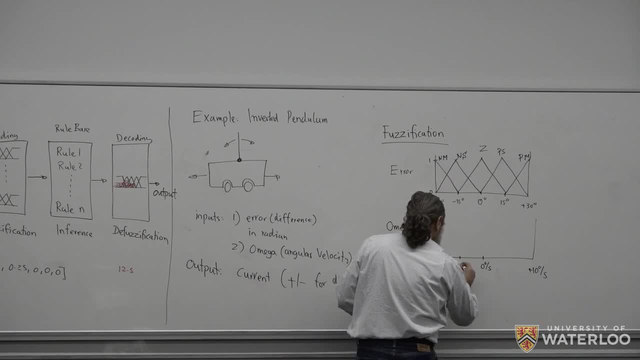 per second, And then we have here minus 5 degrees per second And here I have plus 5 degrees per second. So what is the angular velocity that I measure? And I do the same thing. I do the same thing: 1, 0.. I want to keep it simple. So 0 is this And this is. 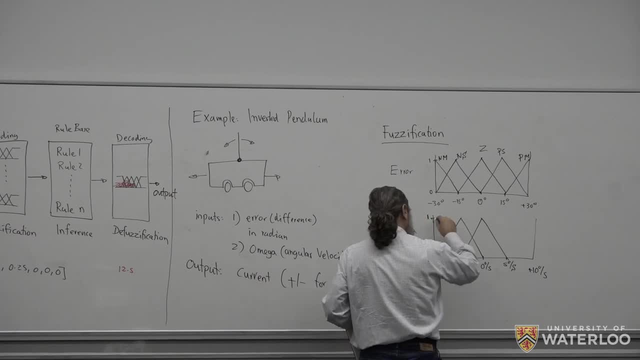 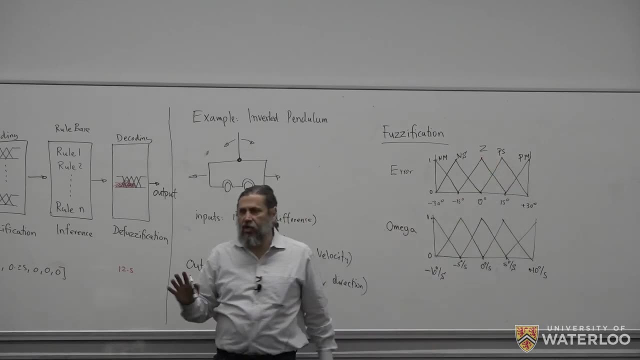 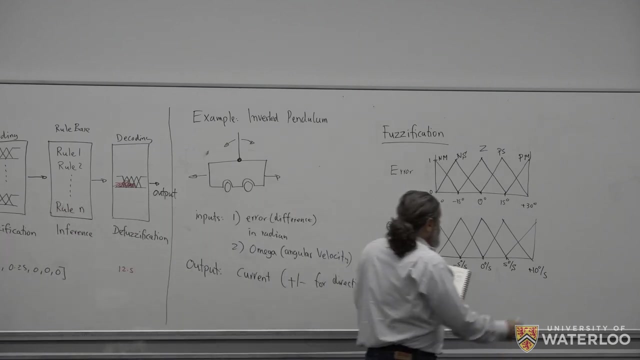 negative small, And this is negative medium. This is positive small, This is positive medium. I'm keeping the labels the same just for sake of simplicity, Because they are numbers, And then I need the current as my output. So how do I get the current? Well, I have. 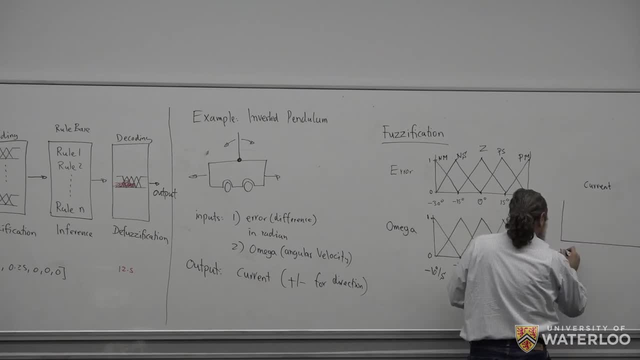 how should I control? I need a current. The current goes from minus 10 milliampere to plus 10 milliampere. In the middle is 0 milliampere, And then here I have minus 5 milliampere. 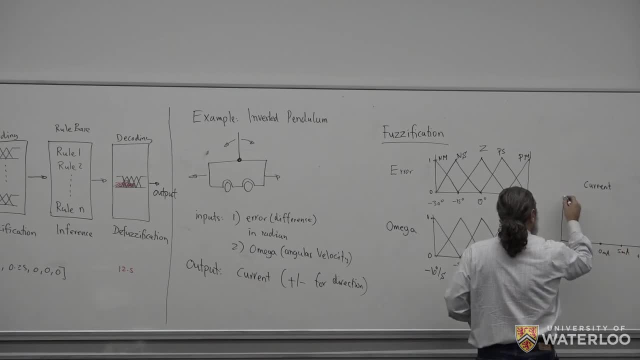 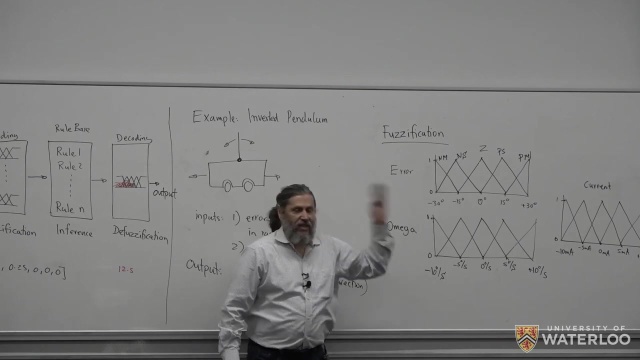 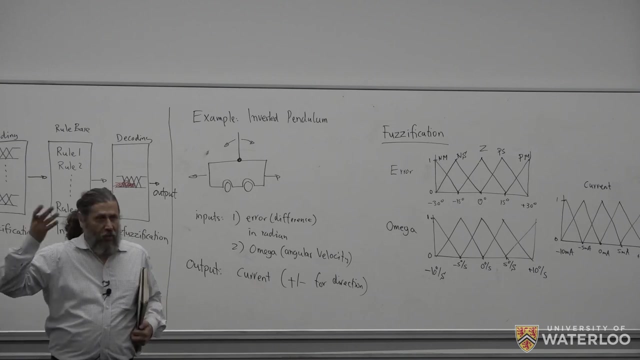 Here I have plus 5 milliampere. Everything's symmetrical. This is 0, 1.. And 0 is again this: Negative, small, Negative medium. Positive, small, Positive medium. I'm keeping the labels the same, Okay, So what? No, I don't know what you want from. 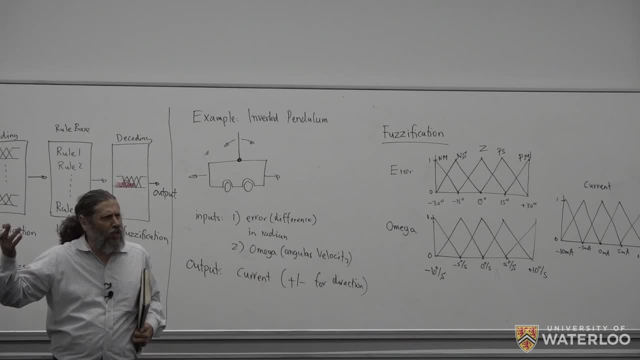 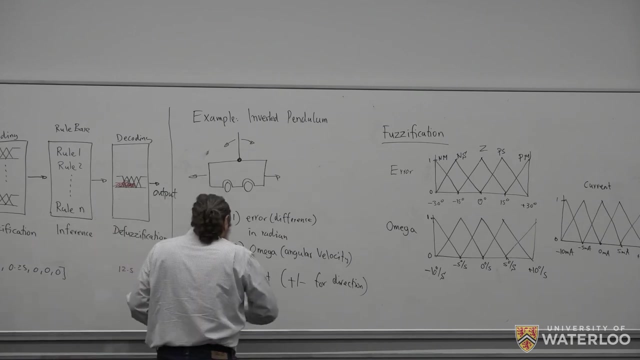 me. So what is? when I was working with PID controller, I knew what's going on. I had some equations, The world had a structure. I was a happy guy. So at the moment I'm confused, I don't know. okay, what, what? Well, we need somebody of experience. 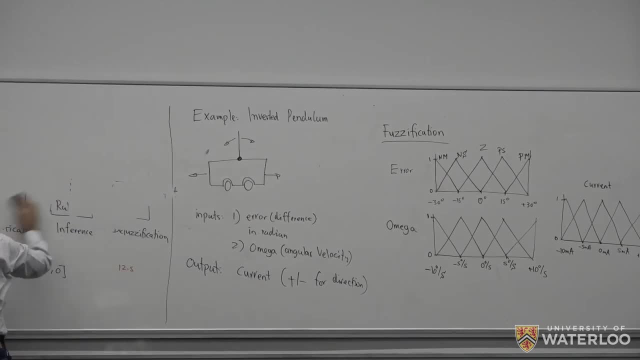 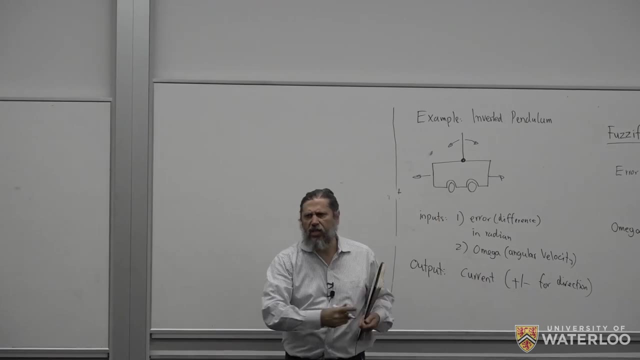 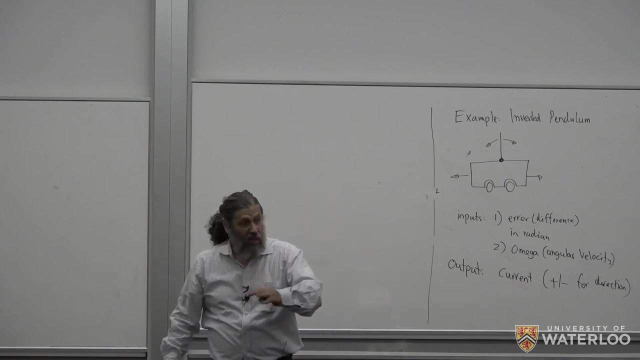 Who can give us some rules, Because fuzzy logic does not work without some rules. So let's say we have no clue how to get rules And a senior engineer comes and says: look, relax, You are new here. I give you some rules this time, But next time you have to figure. 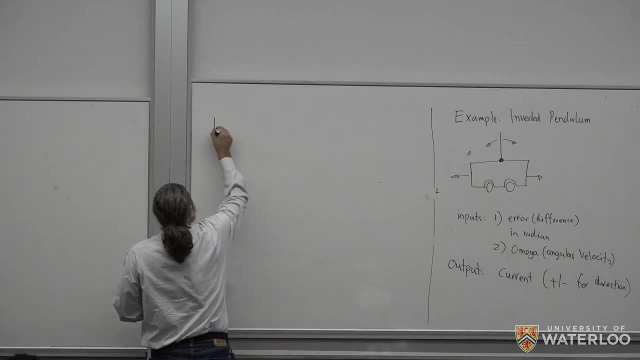 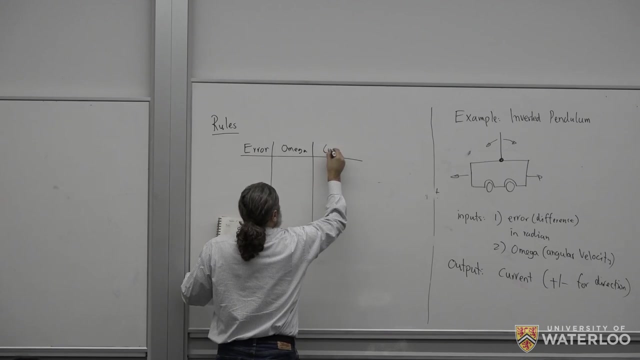 it out yourself. So what are the rules? The senior engineer will give us some rules And he will give us a small table and say: look, this is the error And this is your omega And this is the current, The output. If your error is 0 and your omega is 0, then the current. 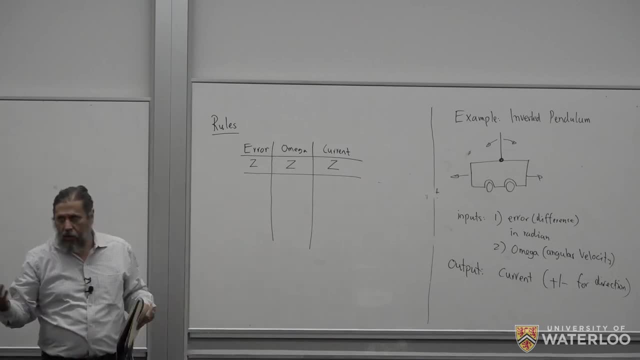 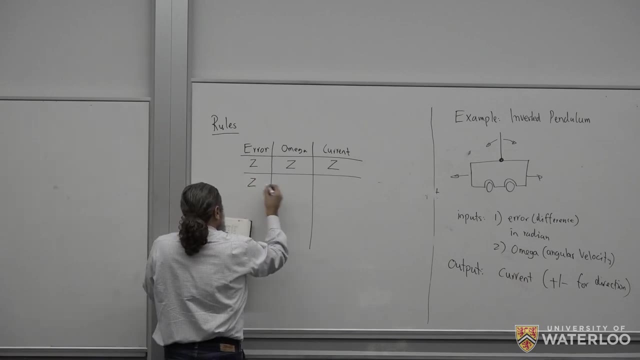 is 0.. Is that clear? You are a smart guy. You say, yeah, I get that. There's nothing to control, Everything is okay. If the error is 0 and the omega is negative medium, then the current should be positive medium. So it's falling. this way, You have to go in the 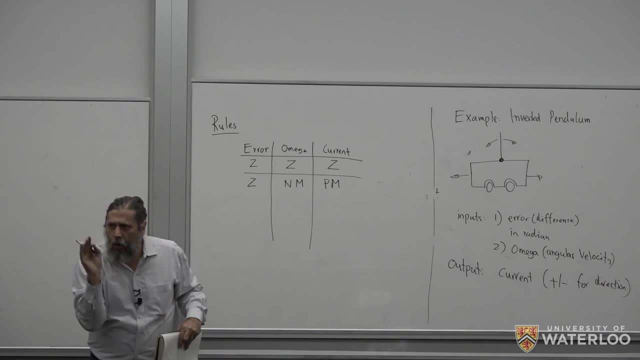 opposite direction, With appropriate level of current. So if it is falling fast, you have to push, If it's falling slow, you have to push a little, Which we will control with the level of ampere. So is it 5 milliampere or 10 milliampere? In which direction? 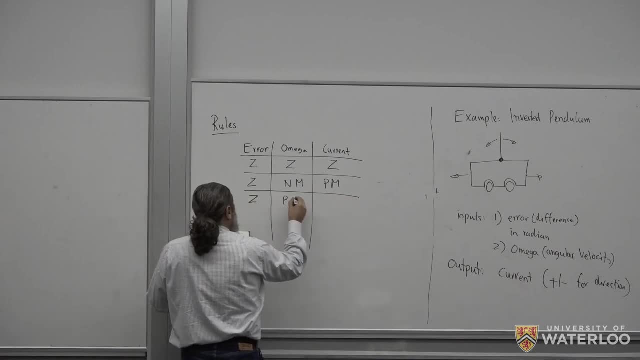 If the error is 0, but the omega is positive- small, then the current will be negative- small, Because again, we want to work against that. In the opposite direction, If the error is positive- small- sorry, positive medium- and the omega is 0, then the current is negative. 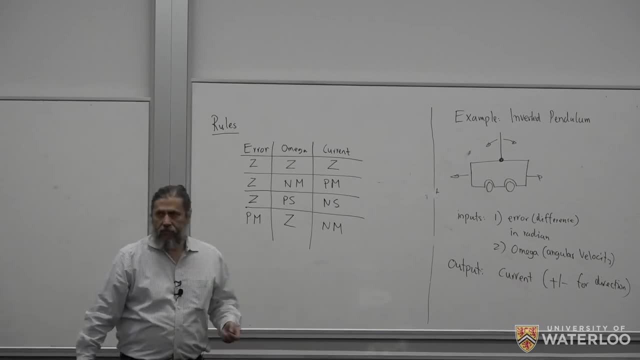 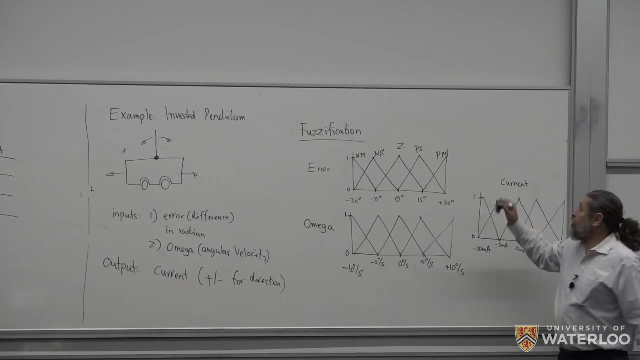 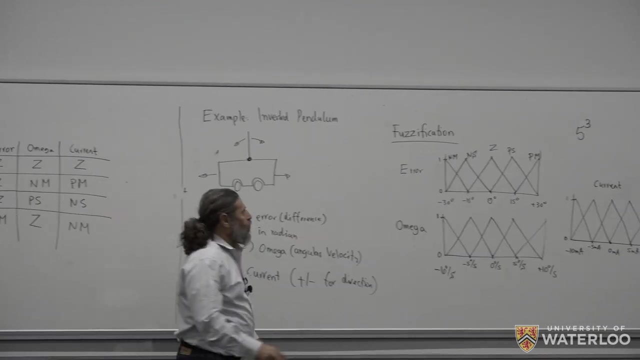 medium And the senior engineer tells me: look, you know how many rules should I get for that problem? Can anybody tell me How many rules do I get for this? How many rules are there? Five, Five cubes, Five times, five times five. So if this is negative medium. 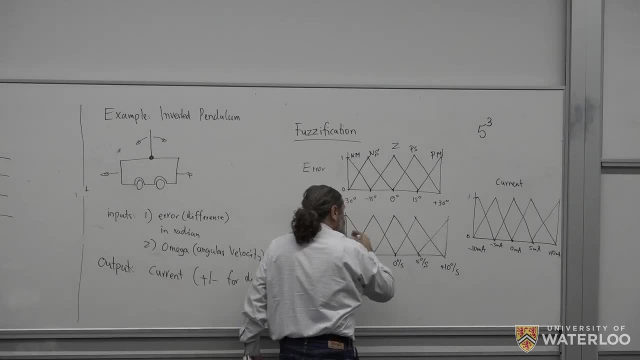 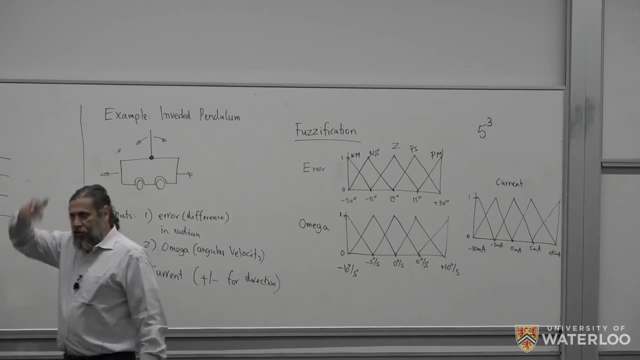 this can be this, this, this, this or this, And in any case this can be this, this, this, this or this, Just for negative medium. So it's five times five times five. So I: 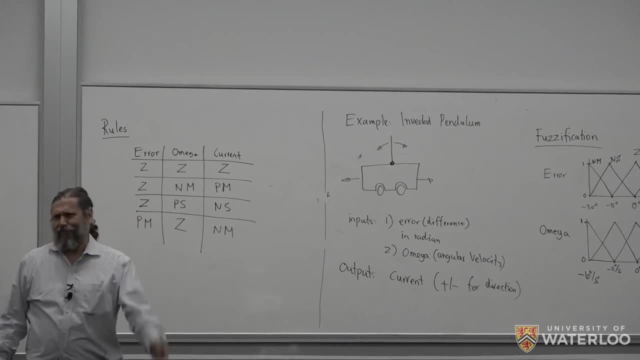 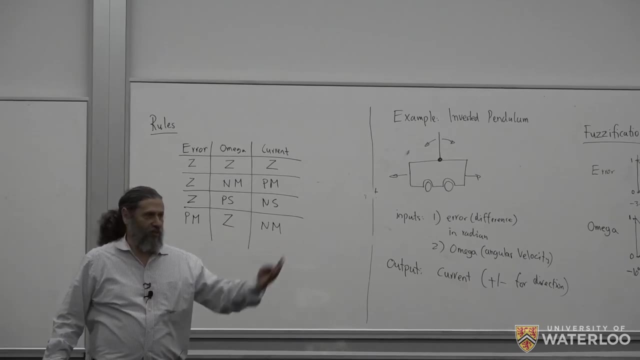 have a lot more rules, but the guy gives me just four rules And I say you should be fine. That's a risky business. But I don't have a choice. I'm new in the company, I have to figure it out. So next time I will write a program and I will get all rules And some. 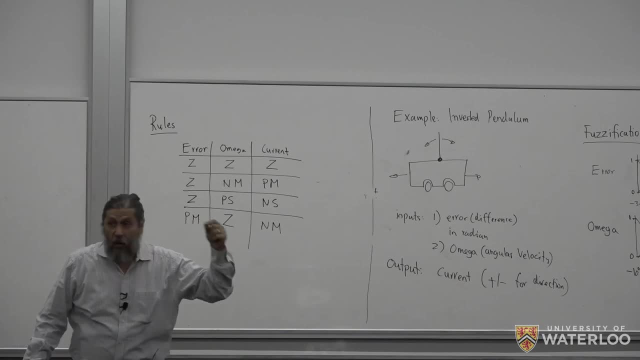 of them are don't care rules. Some of them are theoretically possible And some of them are not, but practically don't make sense. So okay now, and the senior is taking care of us, the senior engineer saying: you know, 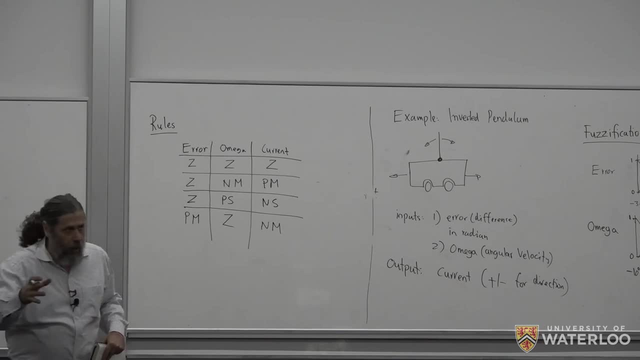 I give you an example: calculate this and then I come back tomorrow I can take a look and see what you did. And he says: look, I give you input measurements. the error is 27 degrees and the omega is minus 1.5 degrees per second. 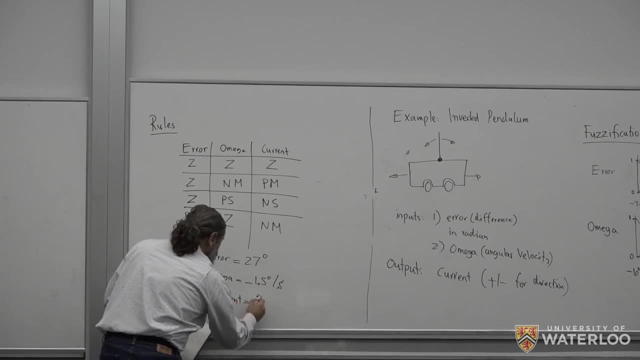 What should be the current? Okay, now, this is an engineering problem. Okay, now I understand the world. Now I'm in my element, Okay, Good, Okay, So I have input, I have to calculate the output, but I don't have any equations. 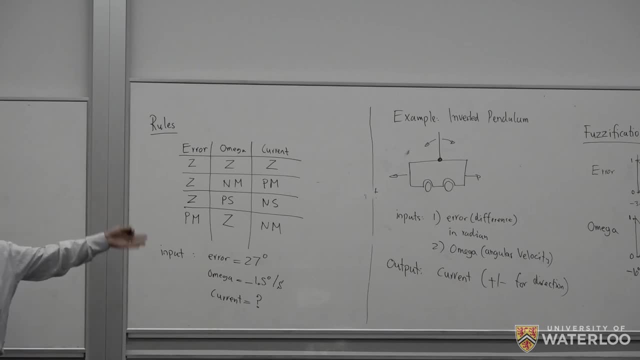 I don't have PID controller, I just have some weird looking functions that some people call fuzzy subsets. And he gives me one rule and say: look, process these rules. I want to make the life really easy for you. I know, if you really want to infer knowledge with fuzzy logic, you have to process all 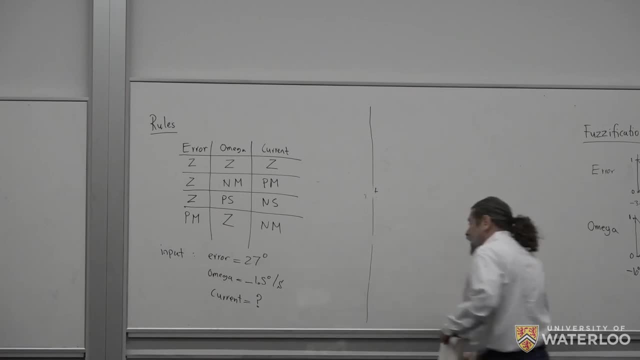 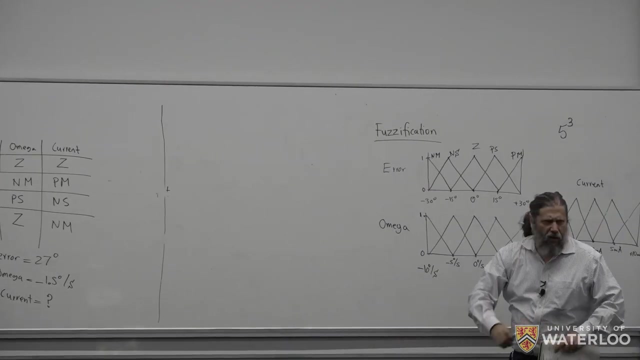 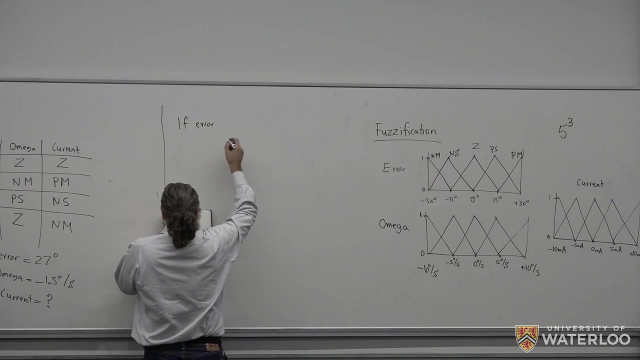 rules at every iteration. So if you make any measurements you have to process five cube rules every time to make sure that your controller stays stable. But he is not tough on me. He says: look, this is the rule. If error is positive, medium and omega is minus 1.5 degrees per second. 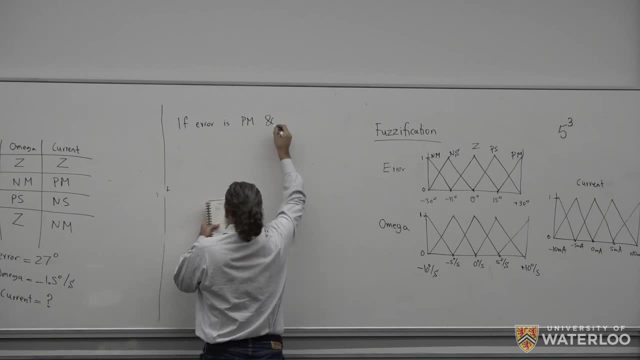 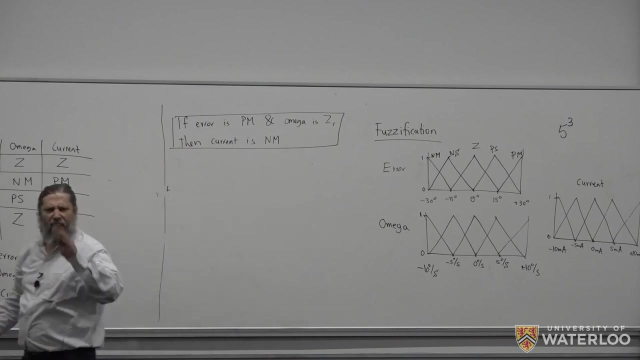 Okay, That's the rule. That's the rule. Okay, Omega is zero, then current is negative medium. This is the rules that the nice caller gives me. Say: don't worry about the rest. I know that you have five cube rules. 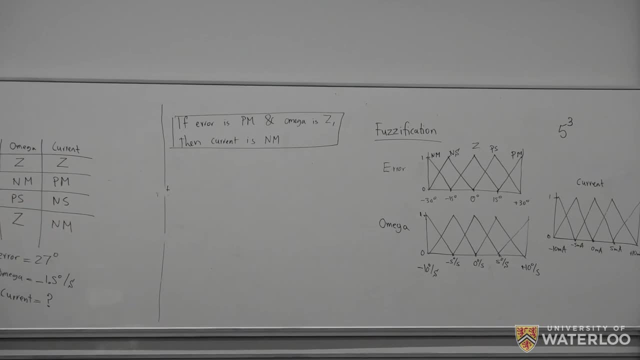 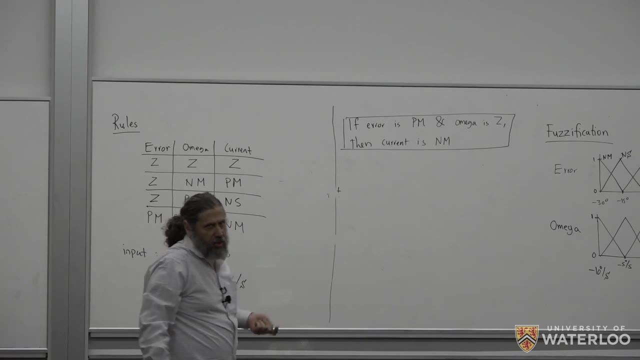 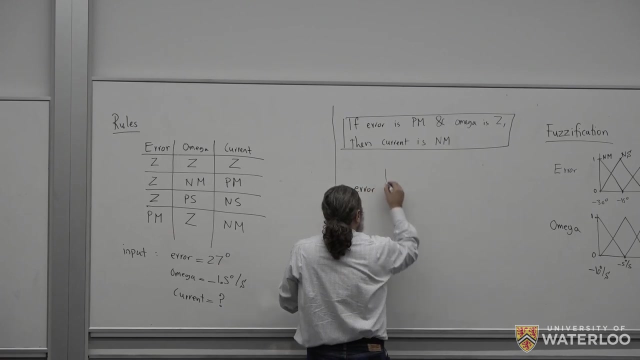 Just show me that you have understood the problem by processing one rule, Because if you can process one rule, just put it in the full loop and you process all five cube rules. It's not a big deal, Okay. So if you look at the error, 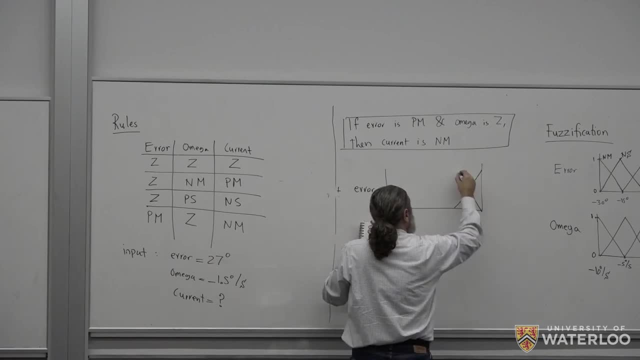 So if I look at 27 degrees, 27 degrees will be somewhere here, Right, 27 degrees will be somewhere there. And I will cut these two functions, And you see that I'm not drawing the other ones, Because for this rule they are irrelevant. 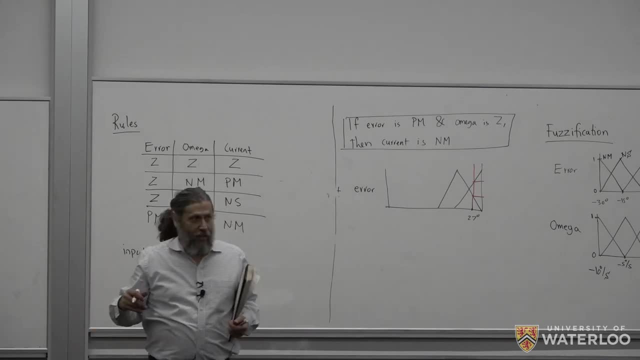 We say that they are not firing. So if I get a rule, some of the rules will fire. If I get- sorry- If I get a measurement- For this measurements Not all of those rules are applicable. They don't fire all at the same time. 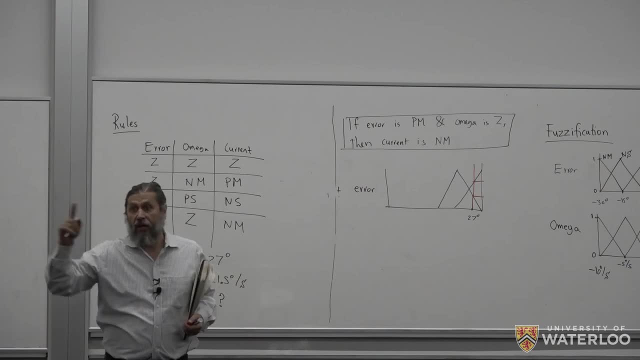 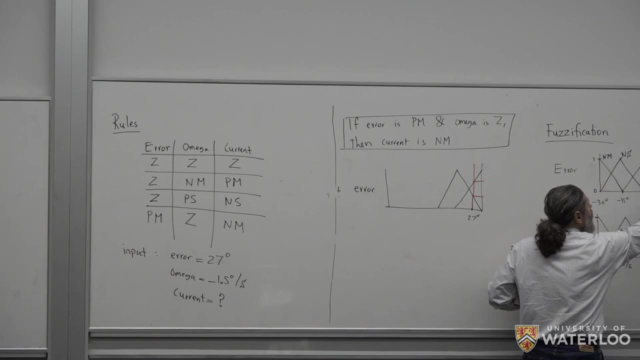 Some of them are applicable And we call them: they fire. So I'm just looking at these two last ones that are applicable, Because I'm looking at 27 degrees. I don't care about negative, medium, negative, small and zero. 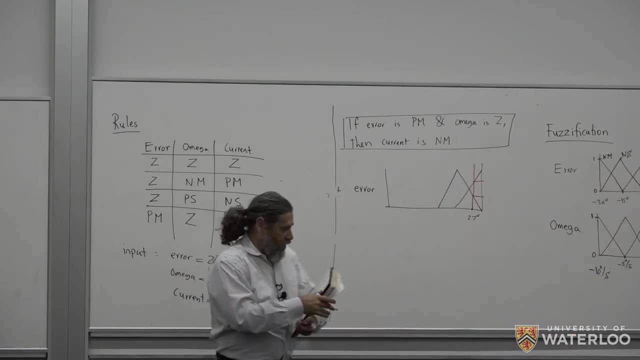 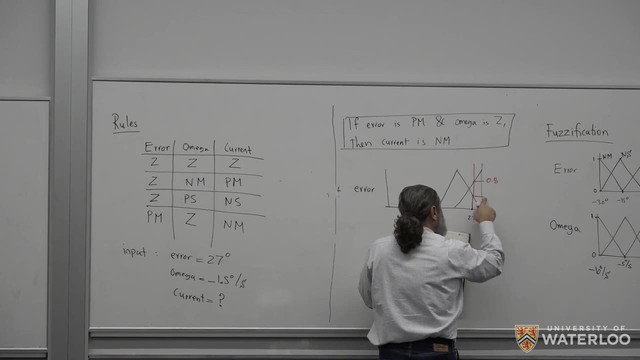 Because they do not affect. They are zero for my calculation. So Let's say this is 0.8.. And this one is other rule. So because you said positive medium, Positive medium, Positive medium, This here is positive medium. 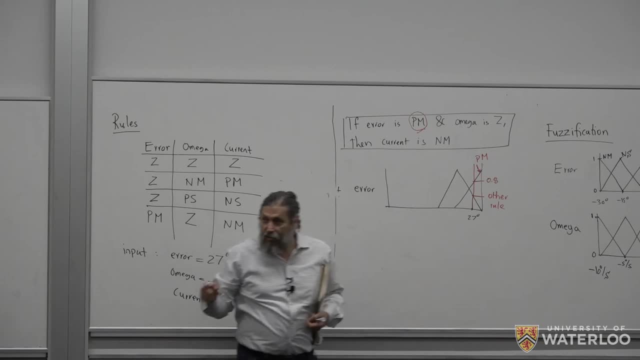 I'm not dealing with positive small Because the guy did not give me any rule for positive small. I could deal with it, But he didn't give me the rule. I don't know what happens for positive small. Then I look at the omega. 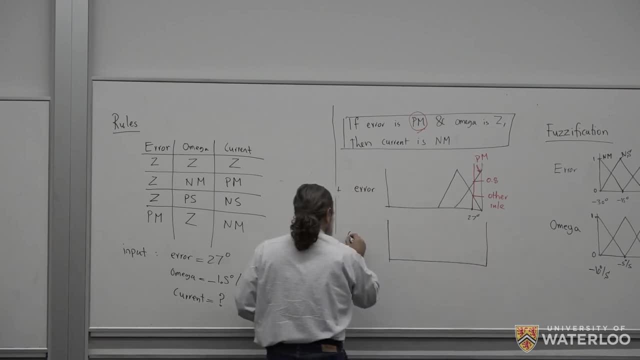 And I get these two membership functions Because Minus, Minus, Minus, Minus, Minus, Minus, Five, Minus, Sorry, No, Minus Minus 1.5 degrees per second is somewhere here. 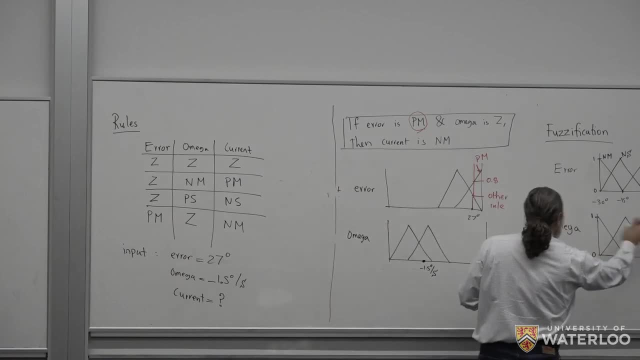 So what is this? This is negative, small and zero And if I cut this two, Omega is zero. I'm interested only in this guy. This guy is the other rule That I don't have it. And this guy is the other rule. 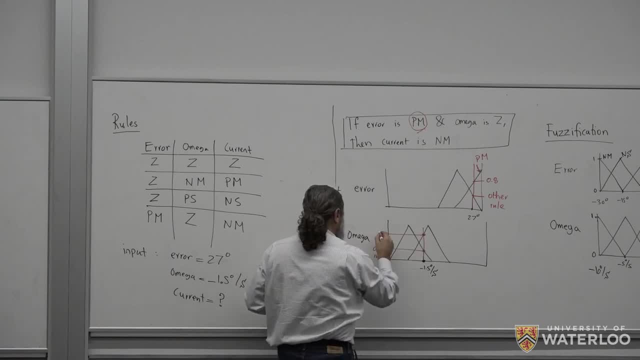 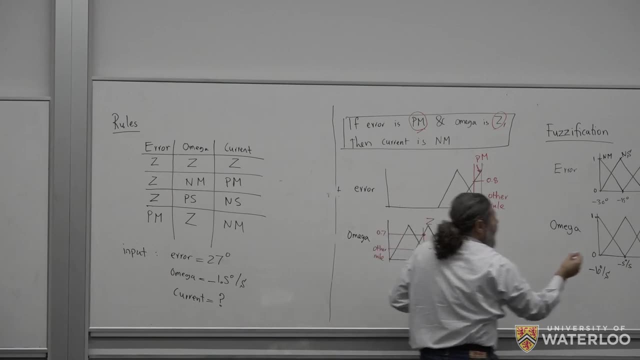 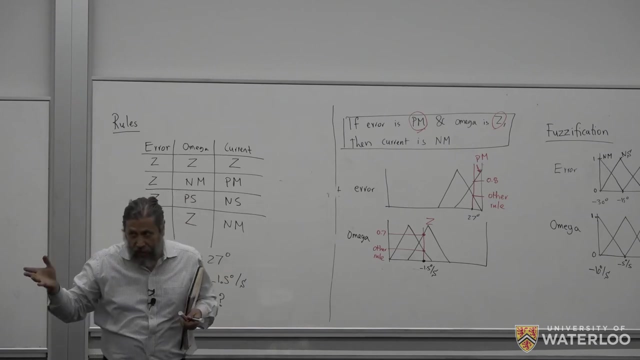 And this guy, let's say, is 0.7.. So this is 0.. This is the 0 and this is the 0. So we are doing manual inferencing, processing just one rule. In reality, you have millions of rules. It gets really nice if you have many rules and they are nicely. 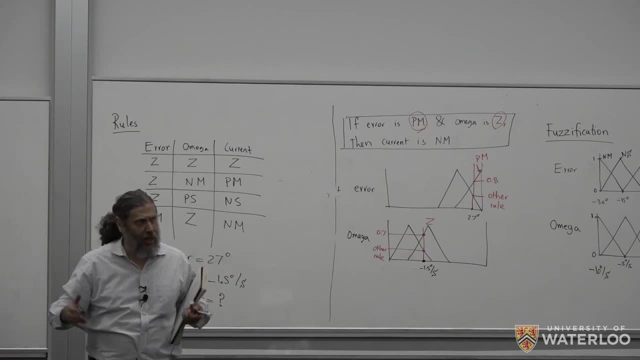 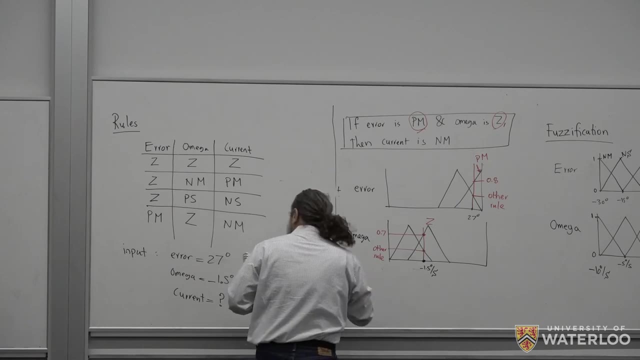 designed and you have multivariable hyperdimensionality, It gets really sophisticated. So you said: AND, AND in fuzzy logic is equal minimum. You can do it other way, but to model, to mathematically model the logical, AND we use minimum. 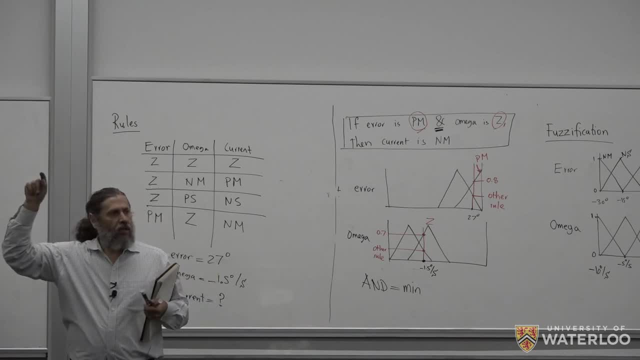 Why False and false is false, So the minimum of 0 and 0 is 0.. True and true is true, So the minimum of 1 and 1 is 1.. False and true is false because the minimum of 0 and 1 is 0. It makes sense. 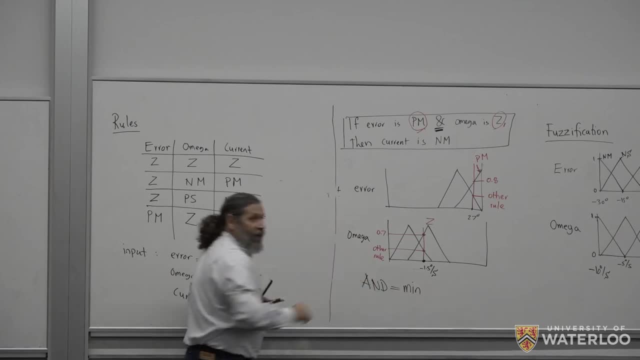 Ok, So I use minimum to model AND So, if error is positive, small and omega is 0,. 0.7 is about minimum of 0.8 and 0.7 which is 0.7, which means modus ponens, the 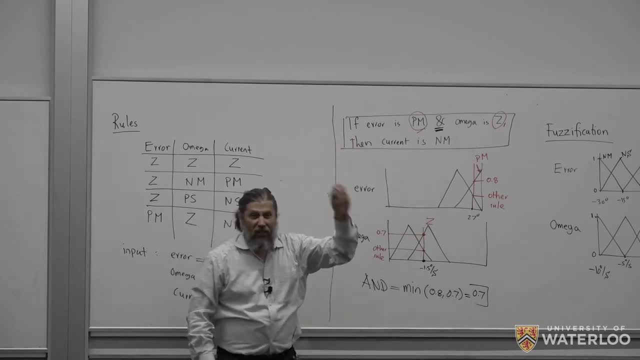 observation that if error is positive, small and the Omega is 0,. this observation is not true and false. in fuzzy logic It's true to 70 degree, 70 percent, So a degree of 0.7.. Oh, 0.7.. 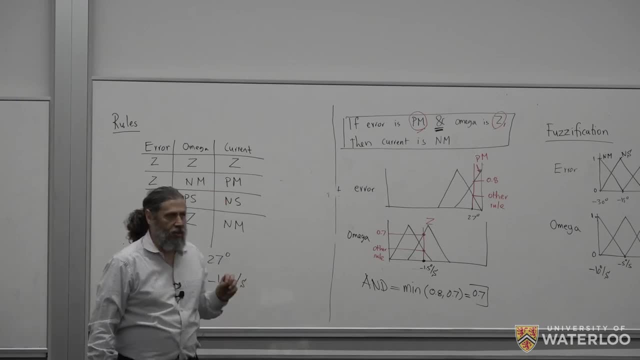 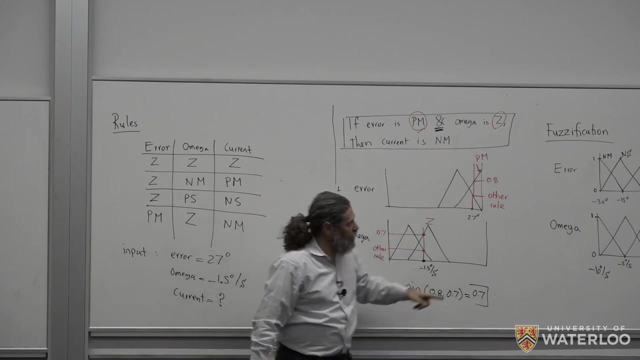 Ok, let's go. Ok, let's go 0.7.. It's not 100% true, It's not 100% wrong. OK, But now for my controller. I need to calculate the current And the rule tells me the current is negative- medium in this case- And the negative. 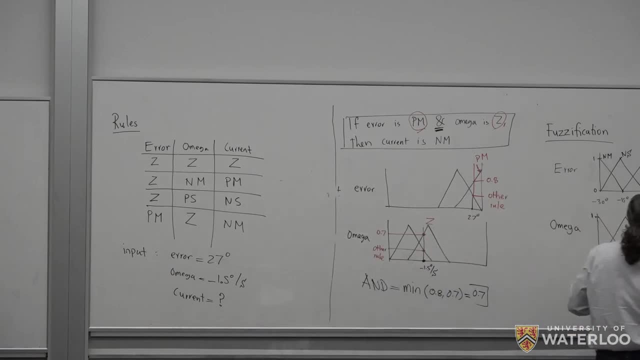 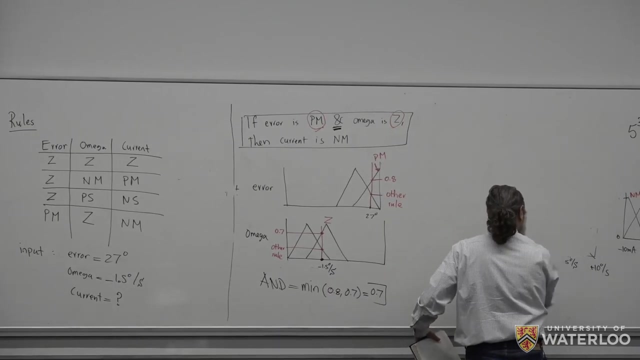 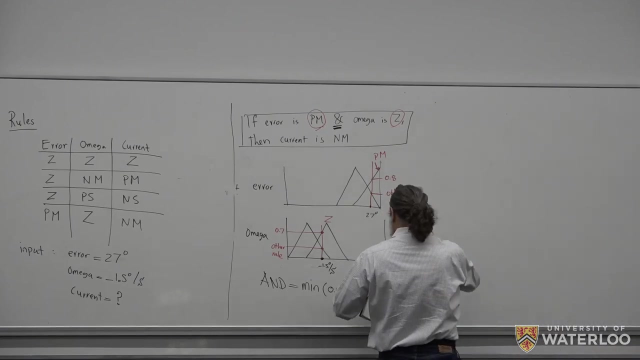 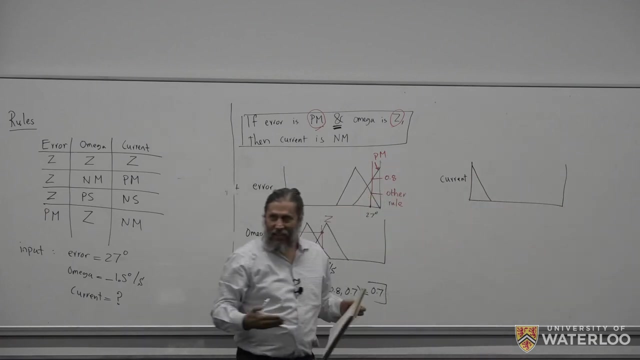 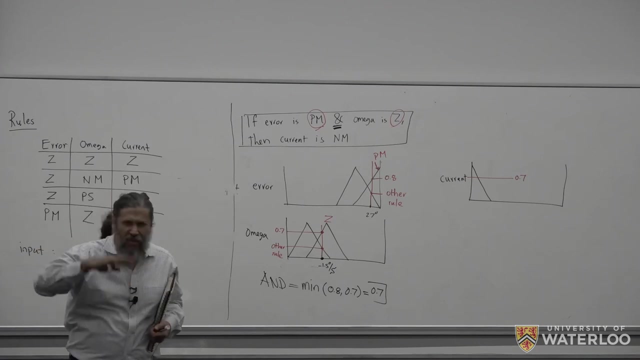 medium. where is negative medium? This is the negative medium. So now I have the current, OK, And the negative medium is this, And I don't care about the rest because I don't have a rule for the rest. And now I caught this at 0.7.. If the premise is valid at 0.7, what I'm 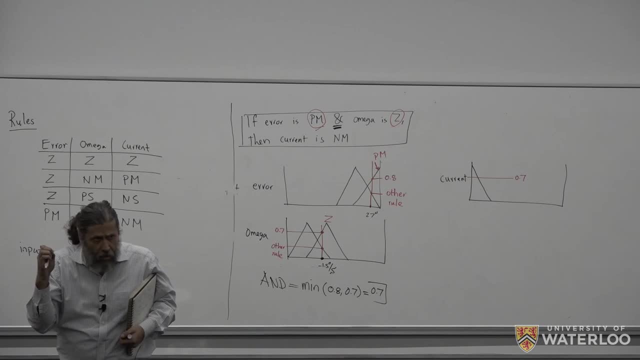 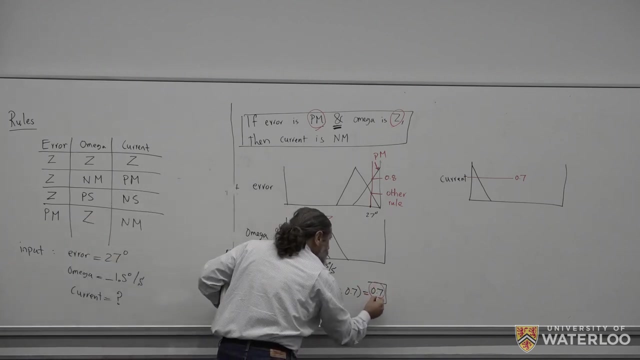 measuring is valid to 70%. I can only conclude also with 70%. I do not have magical powers, I can only work with numbers that I get, So I will cut it with 70%, which is, if error is positive, small and omega is 0, so then it's 0.7, then the current is: what was it? 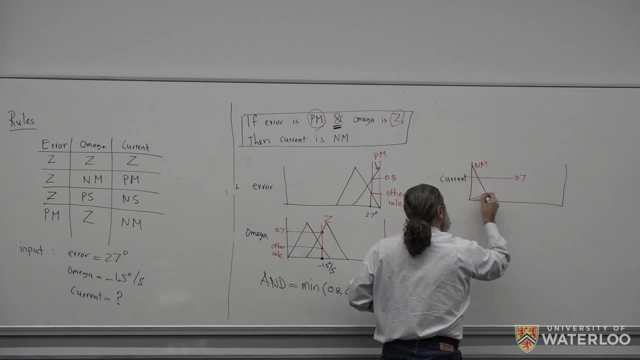 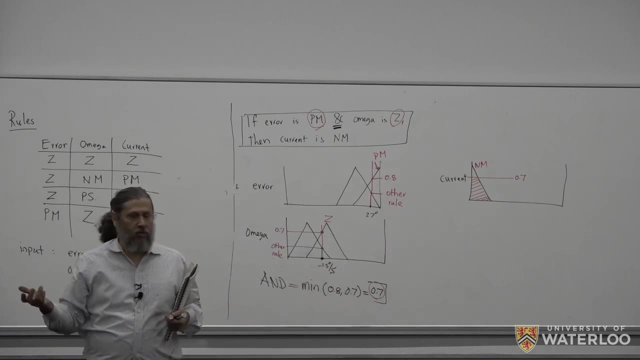 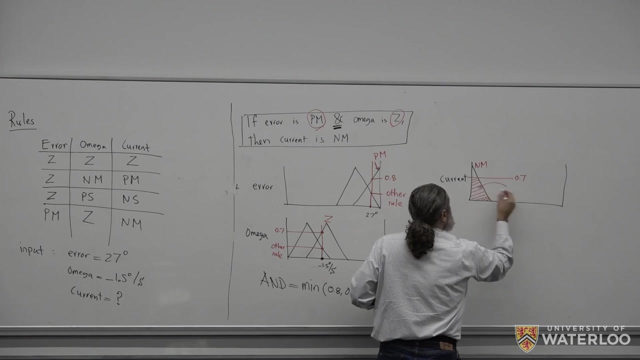 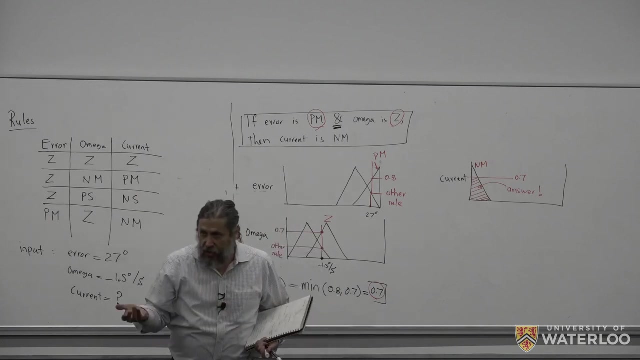 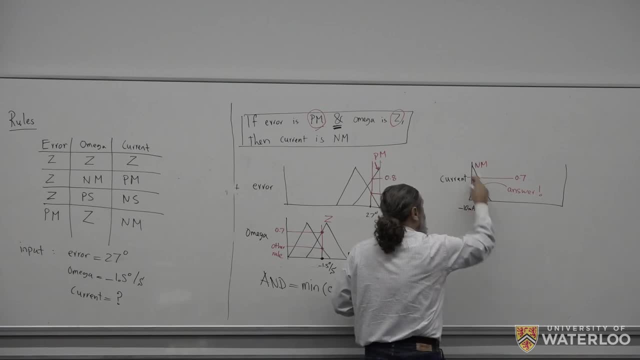 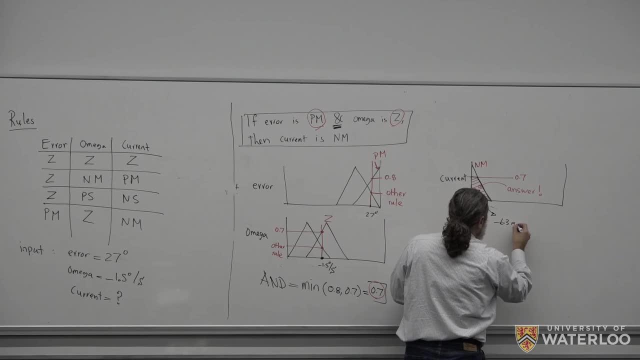 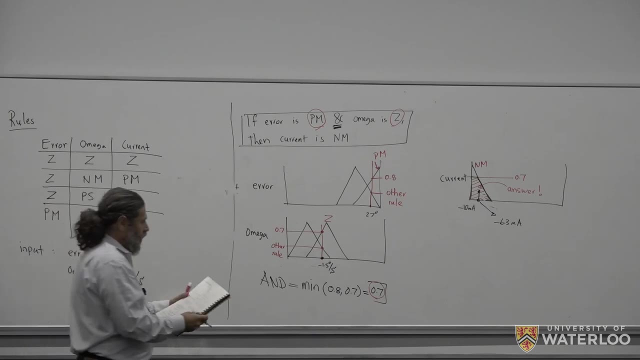 OK, And this will give you minus 6.3 milliampere. If you really draw these functions carefully and accurately, you will get that. So this step that I did, that was the defuzzification, Because that red part is the fuzzy answer of the controller. 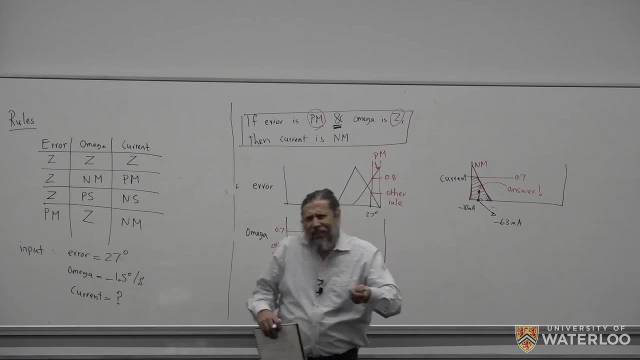 But I need a scalar. So I did a very simple trick And I say: you're giving me a surface, I calculate the center of gravity of that surface, The center of that surface, And I use it as a crisp number, as a scalar. 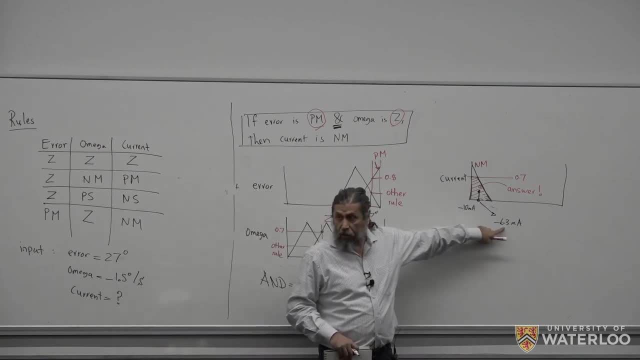 Because my controller needs a number. So I'm pushing that card back and forth. I need a number. So now, if you are measuring with the inverted pendulum 27 degrees and the angular velocity is minus 1.5 degrees per second, you have to push it to the left with 6.3 milliampere. 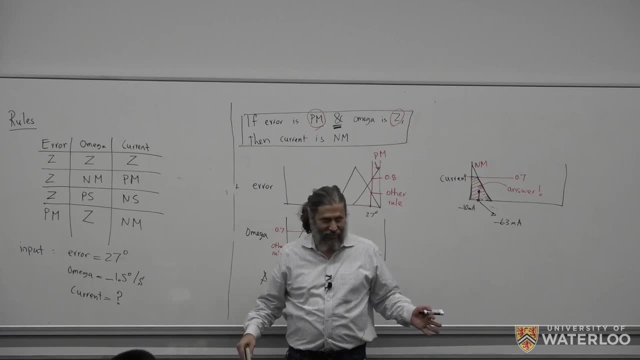 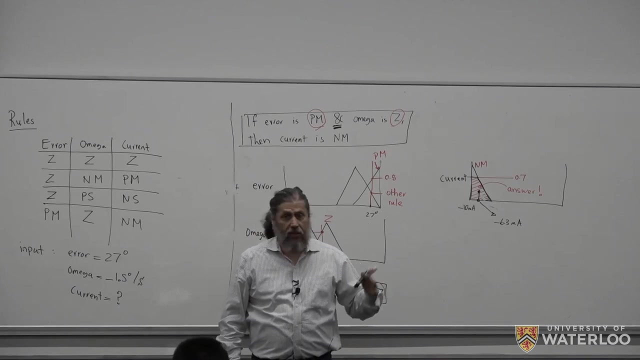 And you're going to be fine. So I guess it was 1984 or 85, the city of Sendai in Japan opened the first fully automated subway system that was completely controlled by fuzzy logic, And as one of the things that they did, 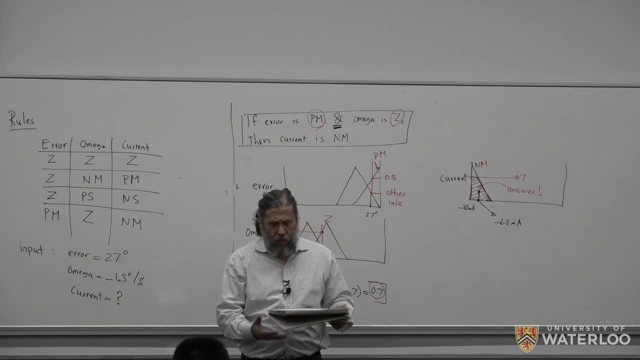 they put a little bit of a filter, OK, They put a colander with an aquarium full of water in there And the level of the water was marked with red And the subway would accelerate, accelerate, stop go, And this level would not change. 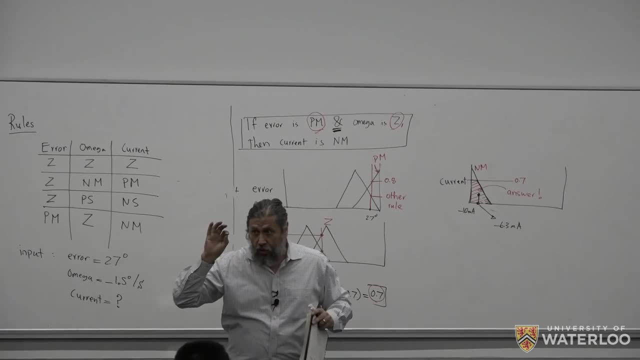 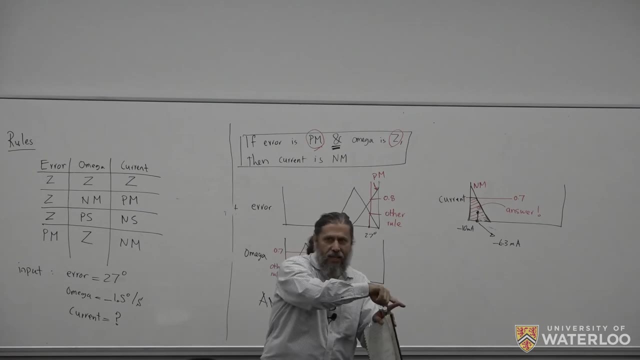 Nothing can impress an engineer who knows what controller does, than that How you can accelerate and stop, Because what is the challenge? When you go from station A to station B, you have to accelerate as much as you can because you want to be on time. But at some point between the stations you have to stop accelerating and start decelerating because you want to stop smoothly. Who likes it if the stop becomes? Nobody likes that. It's a stupid engineering design. It has to be smooth. 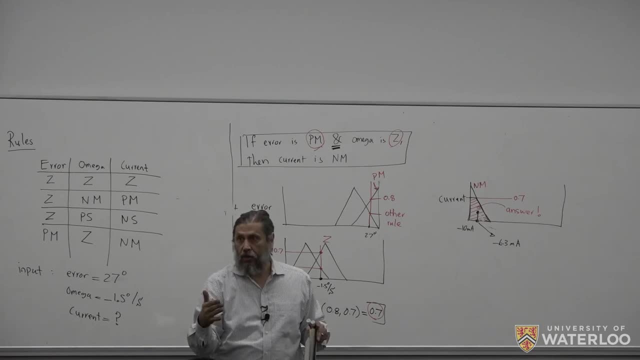 And it had more than 25% efficiency in energy. And the day this is the dream of every engineer- although the guy was a computer scientist- The day that they opened that Sendai subway system. if you can look it up in the first station, 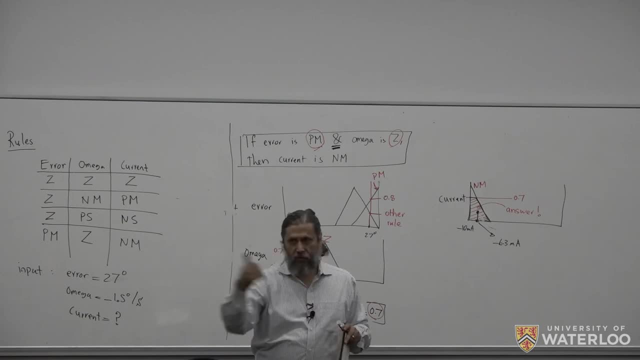 there was one guy standing And there was cameras on him. That was the guy who invented fuzzy logic. Honda gave him some prize. Japanese are really good. After they did that, Europeans came saying: what is this fuzzy logic? So if you want to get the attention of Europeans, 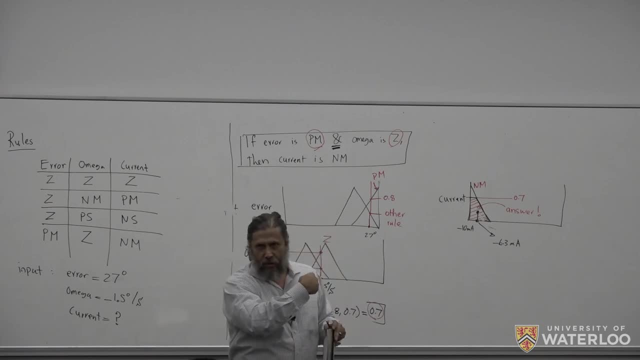 and North Americans. you have to ask Japanese to do something, Because here we spend millions of dollars first to do feasibility studies. What would happen if we go inside this technology and invest? So we spend five years, spend money, give advisors and consultants money to figure out. 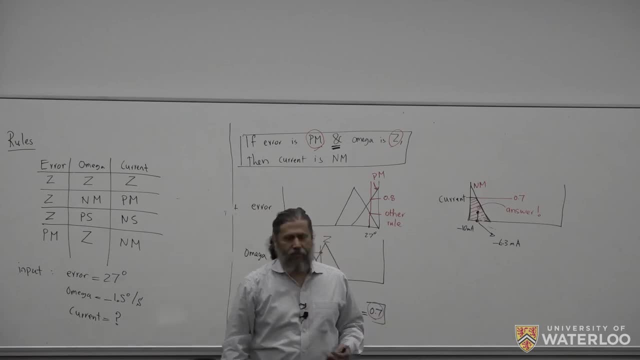 would it be good to invest in AI. What Japanese do they say? let's go in AI. Let's go in The money that you want to spend on the consultants and do feasibility studies, spend it on the AI project. Japanese were very good. 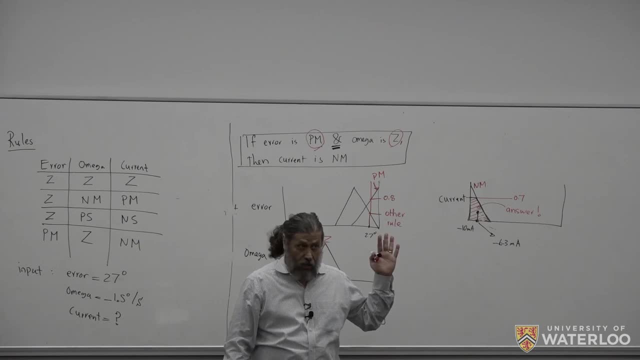 They are not very good anymore. So back in the 70s and 80s, they are not. They are not. They have lost that drive for innovation. They were insanely innovative in the 70s and 80s. They have lost some of it. 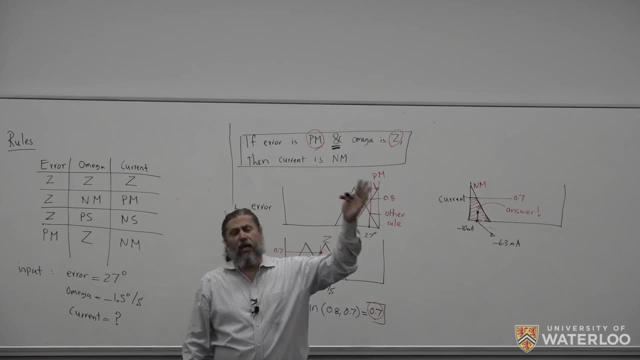 I don't know what happened to them. North American, we were sleeping anyway. Early 2000s. they say what? What Japanese are doing? what? So Europeans are doing it too. What is it? Have Japanese? Japanese have created that right. 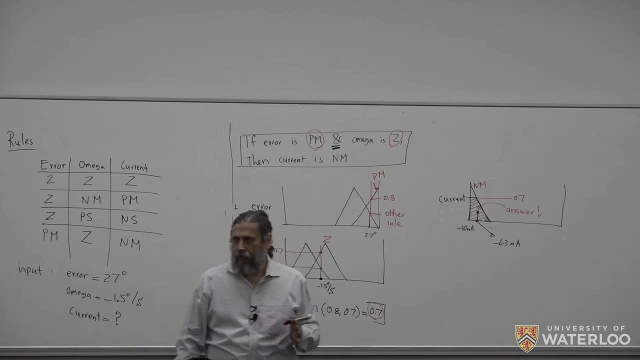 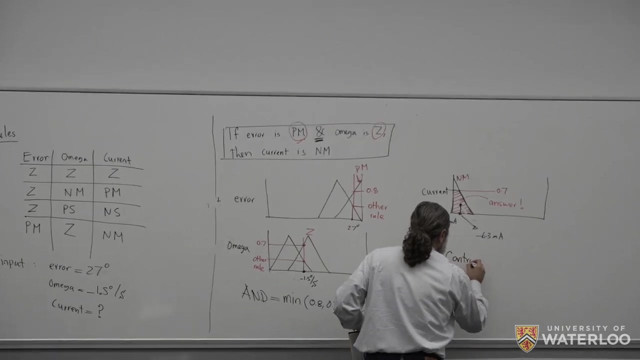 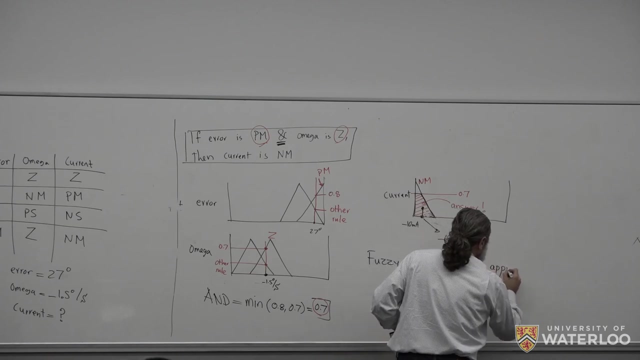 No, It's coming from UC Berkeley, What I don't know, Things like that. So it's very important. So fuzzy controllers can approximate, so you can see that the relationship between inputs and outputs via interpolation in a way that is not. 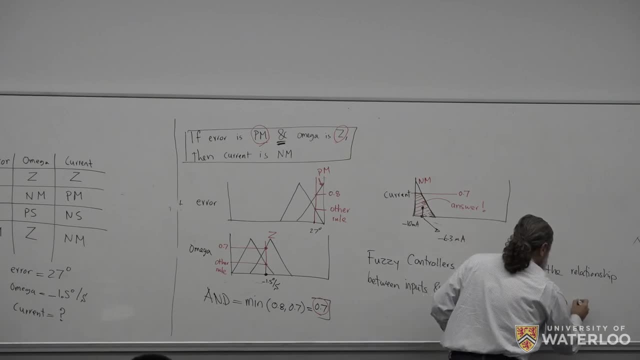 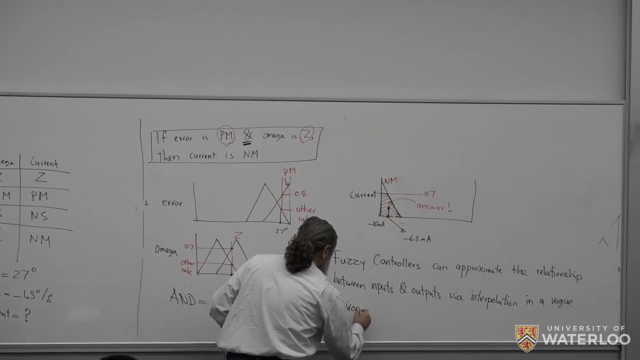 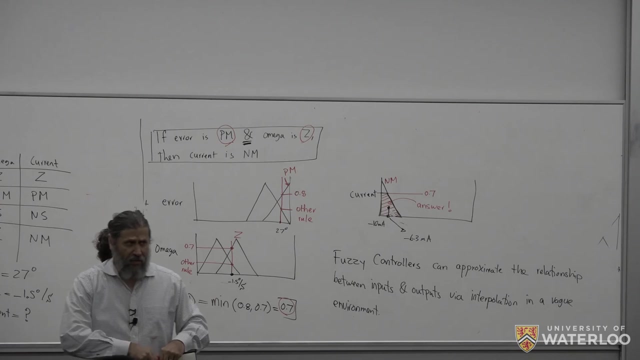 the same. It's not the same. It's a different thing. It's not the same. That's right. environment: This was one of the things that people didn't understand, And we do that with any new technology. I don't know what is wrong with us. We don't. 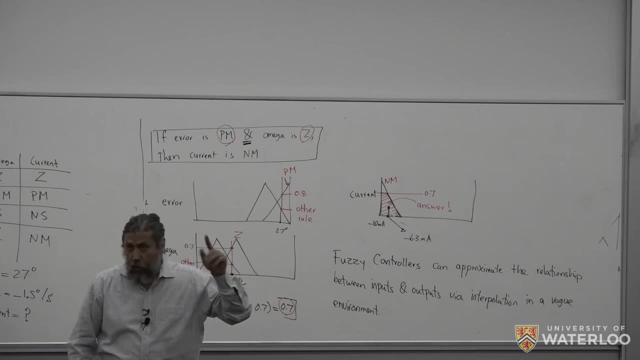 really learn. We did that with neural network. Neural networks in the 70s and 80s. they were underground theories. You couldn't say you are working with neural networks. You want to say I'm looking into connectionist models. You wouldn't. 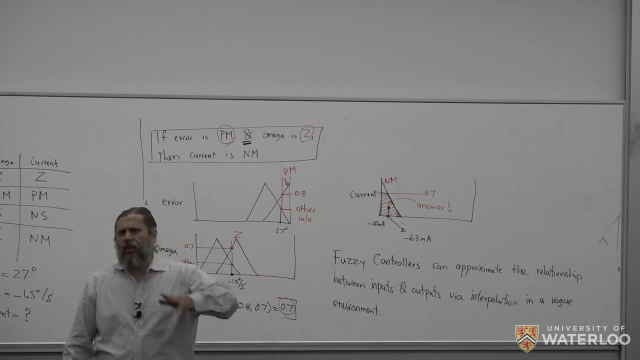 you wouldn't use the word neural networks. Same thing happened with evolutionary algorithms. How does that work? What is the math behind it? Same with physiologic, Any new, basically any new technology. The question was: what is this? What does it mean? Then we had in late 90s we had 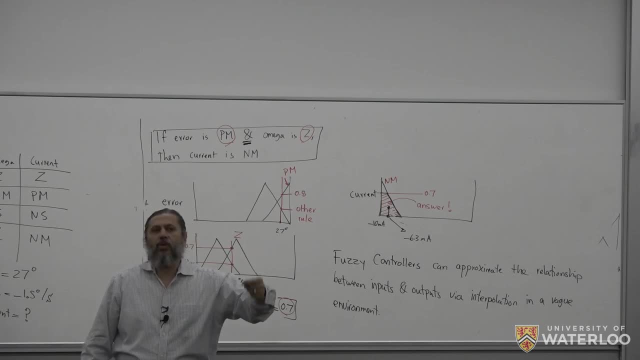 among others, many, many work on it. a PhD person from Germany wrote a PhD and and showed mathematically that what it does is a new type of interpolation. It's interpolation in a vague environment that numbers are not accurate. Oh, okay. 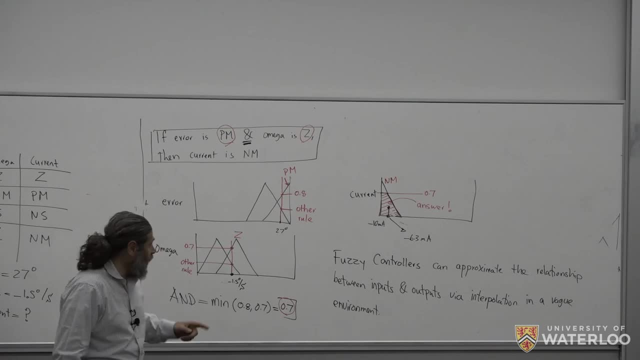 So we have a new type of interpolation. Fantastic Now, but fuzzy logic does not have any capacity of learning. So how do you get those rules? How do you get the rules So you can, if you have numbers, so let me write it here, maybe. 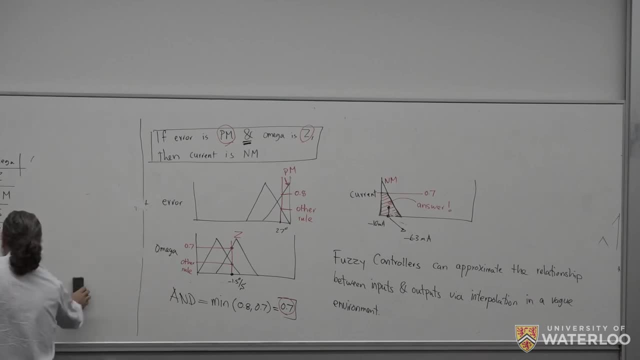 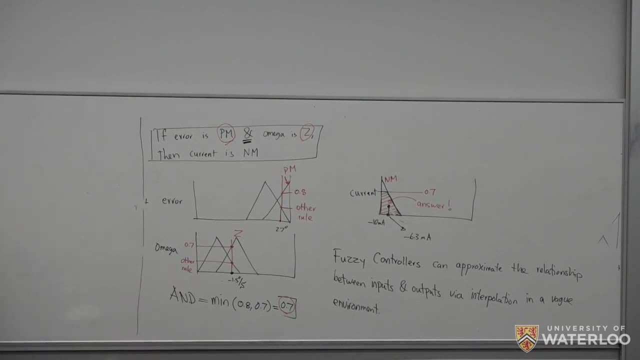 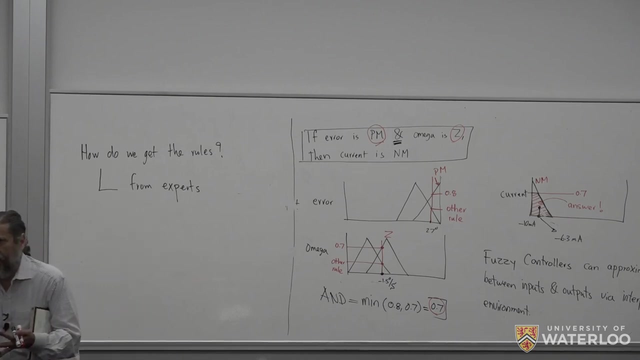 Okay, we have one more minute. So how do we get the rules? So, we can get the rules from experts, But that's not going to be efficient. I have to sit down with an expert, a financial expert, a medical expert. 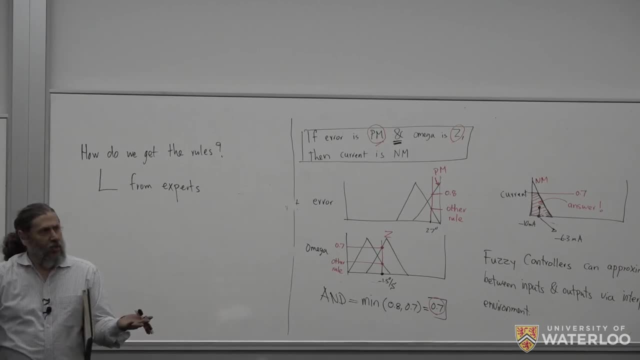 And ask him or her: how do you do it? So that's what one of the first applications of fuzzy logic and automation of concrete plant. They went in and sat down with the expert- how do you control the plant? And the workers? the workers were saying, yeah, if I look, if the難. 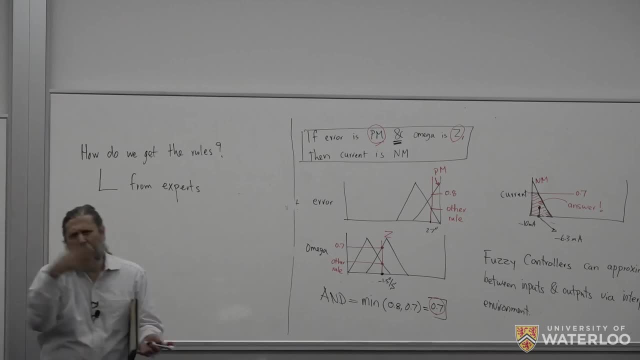 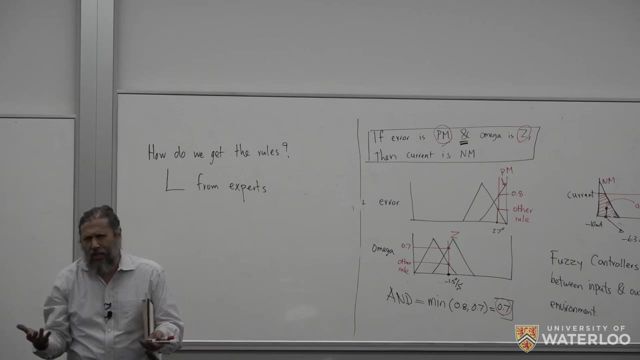 if the pressure is high and the temperature is low and my mood is low too, I do this, So you interview the expert and you get some rules. This is not very reliable, So most of the time we get it from data via clustering and via. 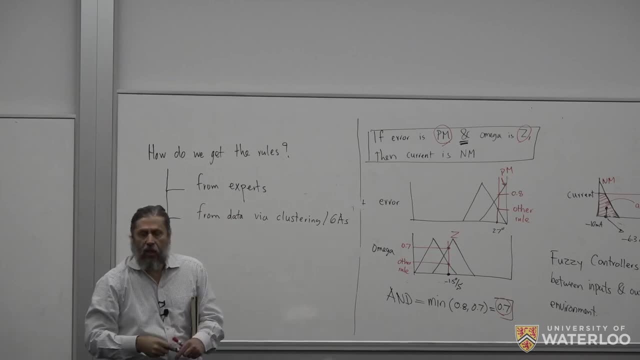 genetic algorithms and many other methods. You give me the data, I run clustering on it and I get the center of classes and I can define the rules. It's possible, we can do it. There is also the concept of evolving fuzzy rules. This 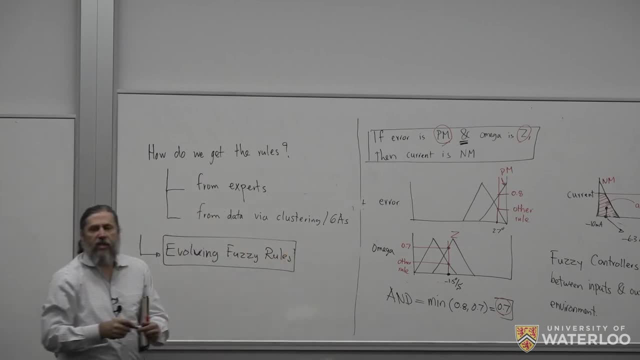 is one of the most recent development- that when you define the rules, there is something in difficult systems that we call concept drift. If you design something, also a neural network, clustering, reinforcement, learning, decision tree, fuzzy system- doesn't matter, Things in reality change. 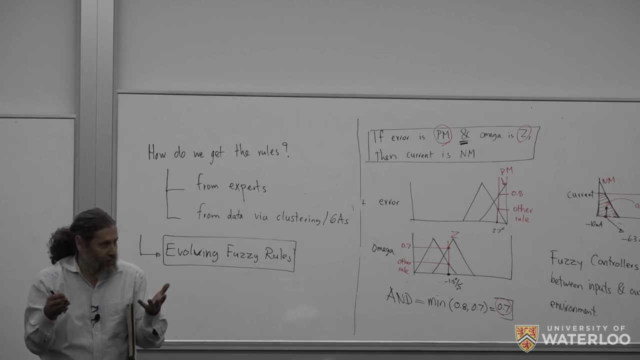 You do diagnosis and new disease arise, Or we rename the disease, Or we have new measurements for the disease, So the concept drifts, So you have to be able to adjust. Yes, reinforcement learning does a fantastic job in that regard, because interaction. 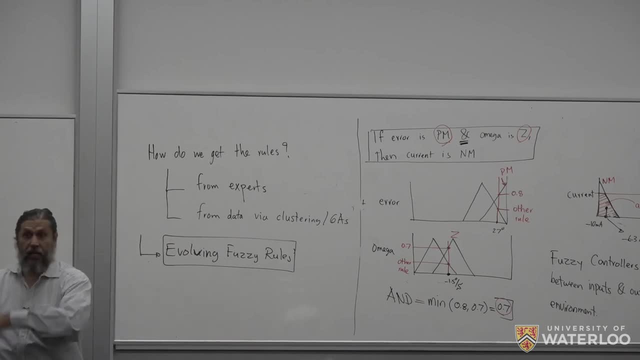 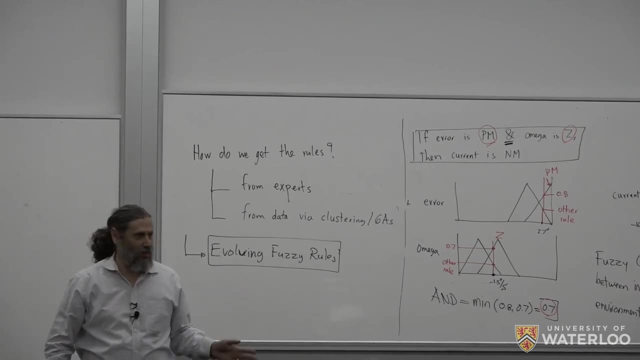 Neural networks suck at it. You have to take them offline, train them again and deploy them again. Very expensive, Evolving, fuzzy systems and decision trees- fantastic for those type of problems. They can adjust as you go. They just minimally. 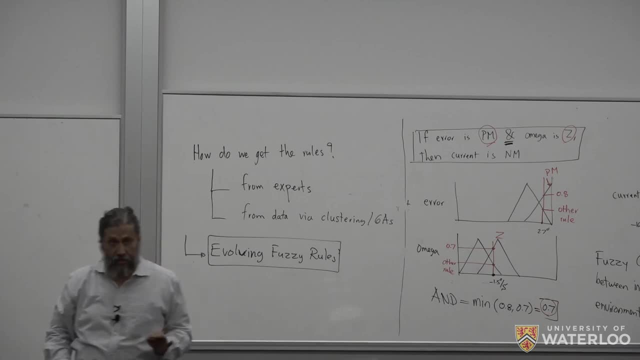 okay, I changed this rule, that rule, this rule. There you go, You're fine. So one of the things that I will look into that are evolving fuzzy systems And of course, there are combination of fuzzy systems and neural networks. There are. 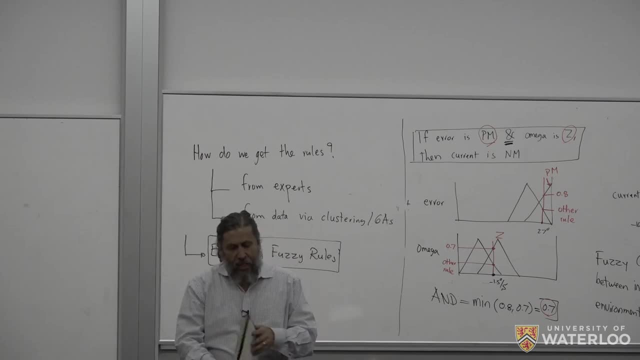 combination of fuzzy systems and evolutionary algorithm and so on. So today in the tutorial we will talk about TensorFlow and CNN. So how can you design a convolutional neural network in TensorFlow? And hopefully we can go step by step such that you can follow.